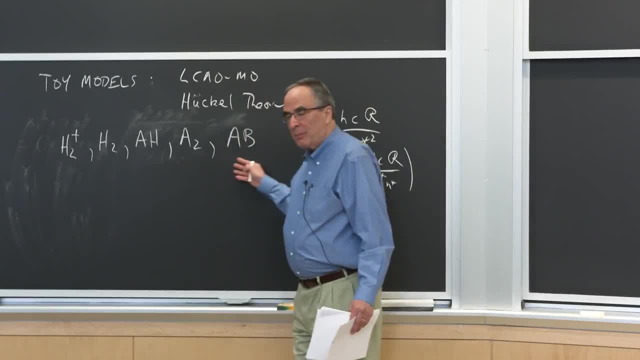 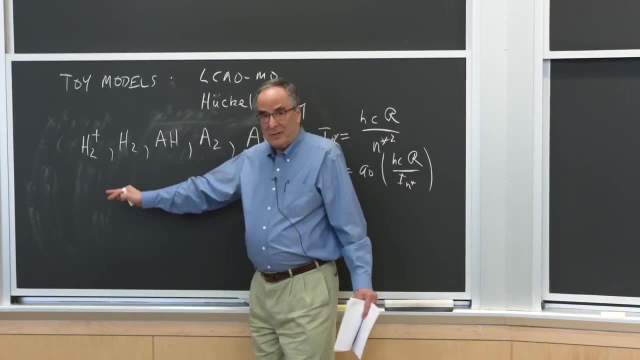 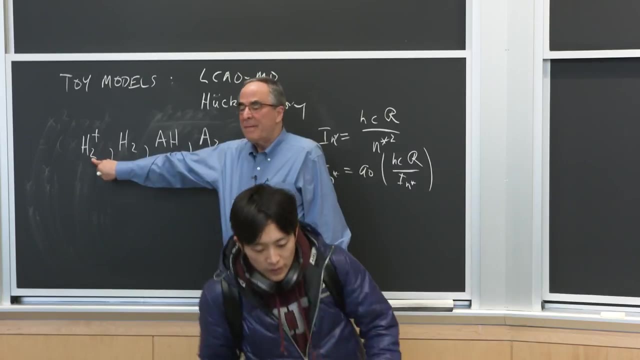 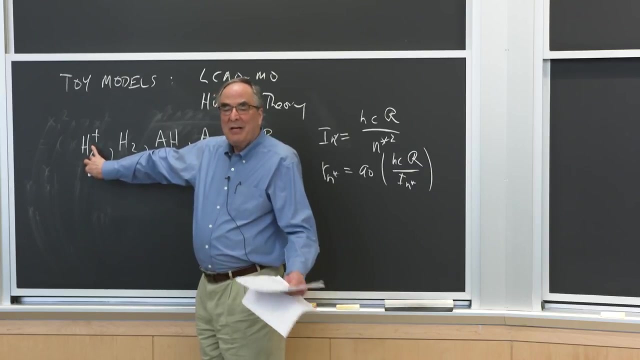 to basically an interpretive framework that can be applied to basically all diatomic molecules, And the logic is relatively simple. We know this one. We get the molecular orbitals for H2 plus. There are basically two: There's the bonding one and the antibonding one. 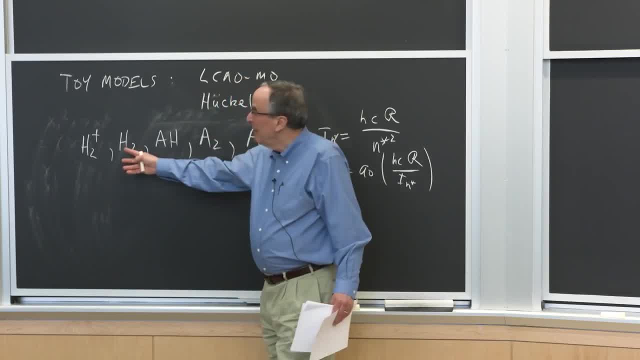 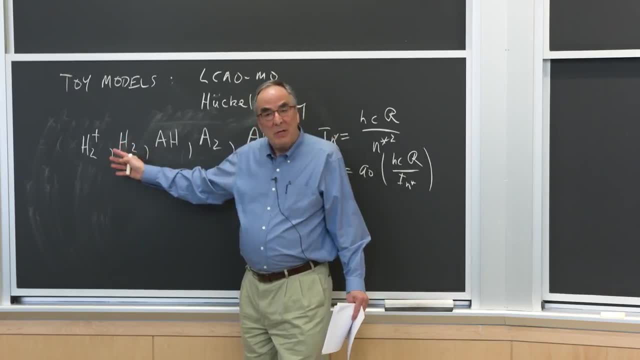 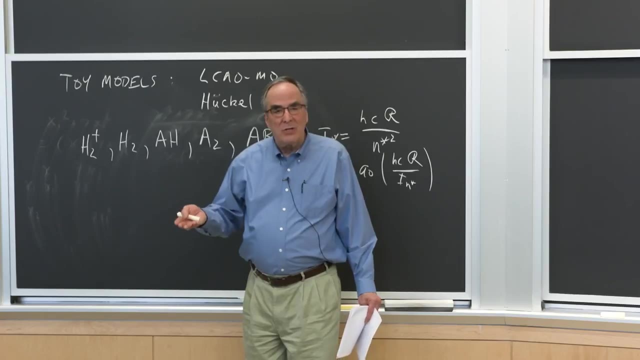 Of course there's many more, but we don't care about them. And then we go to H2. And again, there's basically only two orbitals that we care about, because the next higher principal quantum number has such high energy That we can just forget about them. 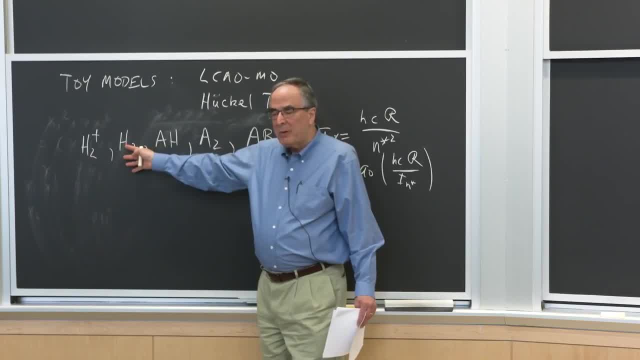 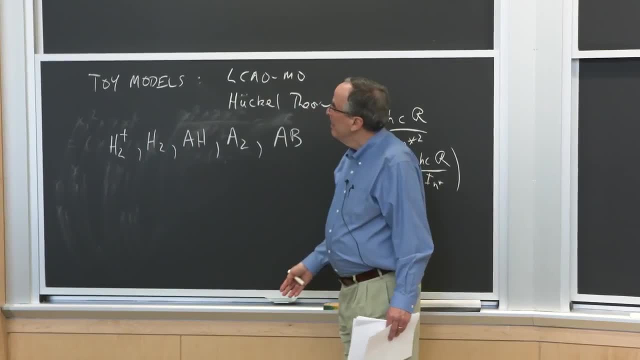 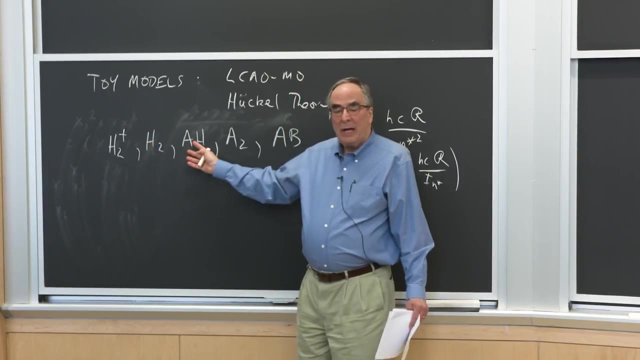 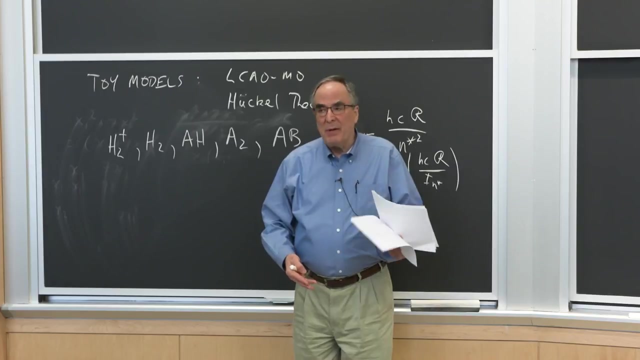 because those states that derive from the higher principal quantum number are Rydberg states or complicated things, because they're at such high energy. And then it's a very small step to go from hydrogen to the AH molecules because, well, we've got the electronic structure for the atomic, for the A atom. 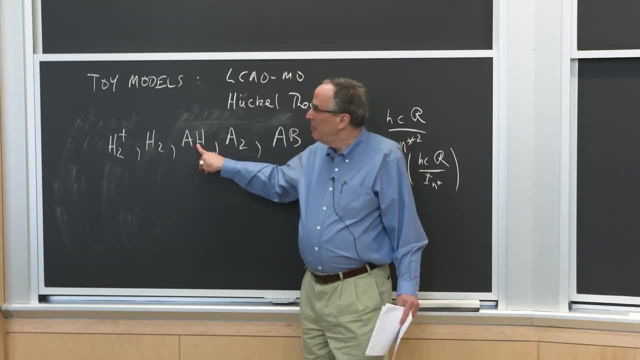 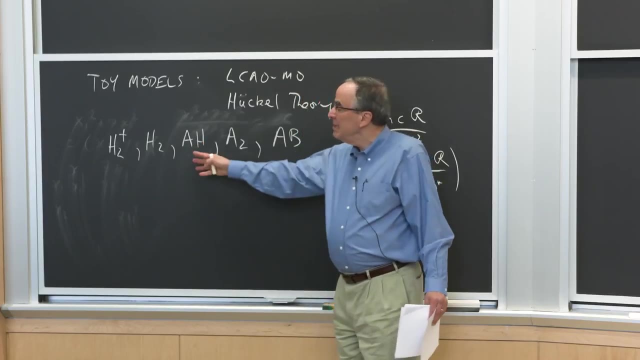 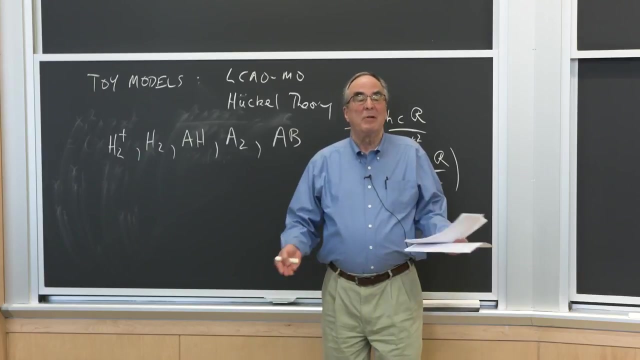 which is complicated. It's more complicated than hydrogen, But because hydrogen only can make sigma bonds, because the p orbitals in hydrogen are so high that it's a simpler picture and can easily be understood. This is in all the textbooks And it's more or less given to you as something to memorize. 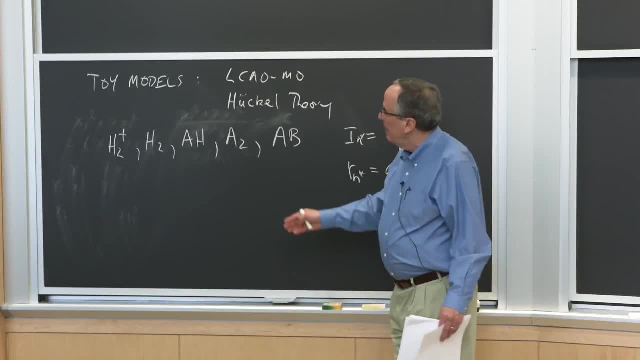 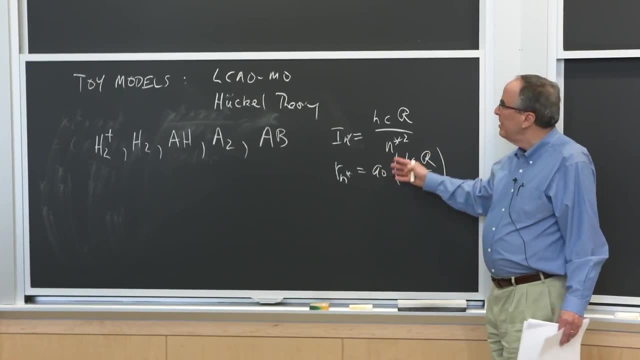 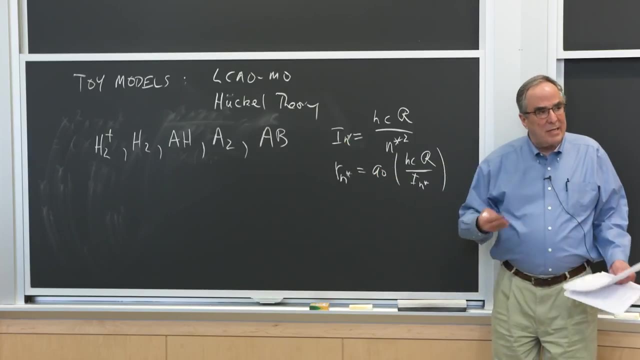 But there's a lot more to it than just memorization, And the important thing is that everything in LCAO MO for diatomics is based on the periodic table, And the periodic table tells you about the ionization energies, the periodicities of ionization energies. 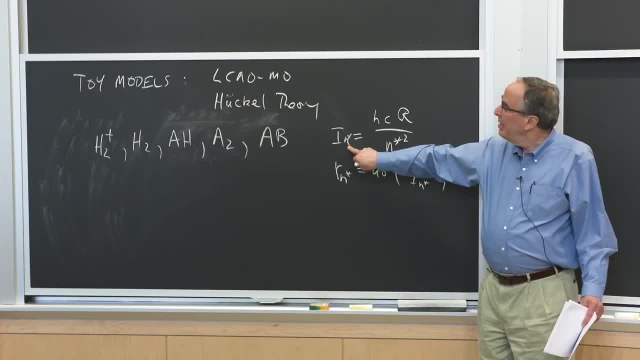 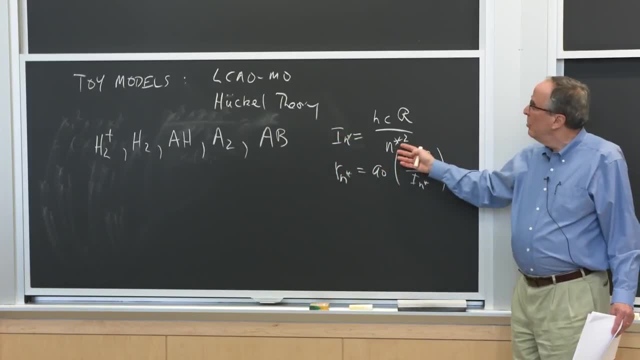 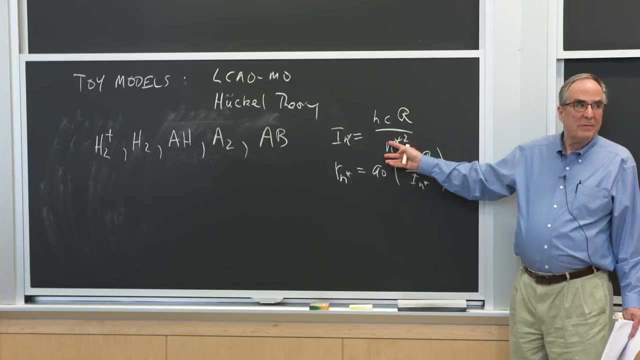 And so we can say for any non-integer, well, if we know what the ionization energy from a particular state is, we can use that. We can use that ionization energy to derive a non-integer principal quantum number. This is all empirical. 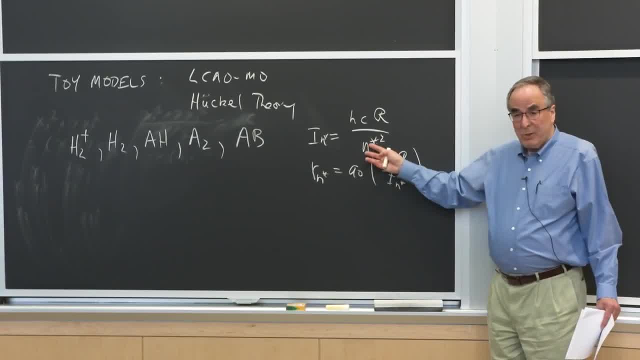 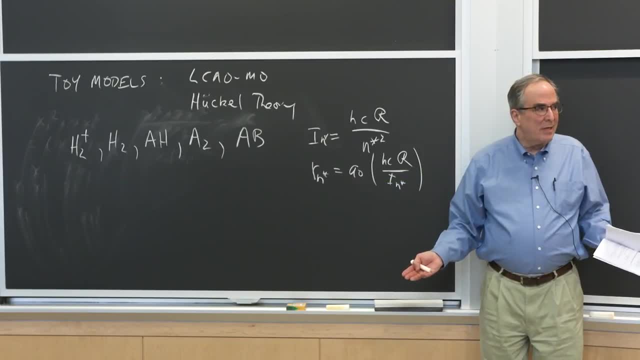 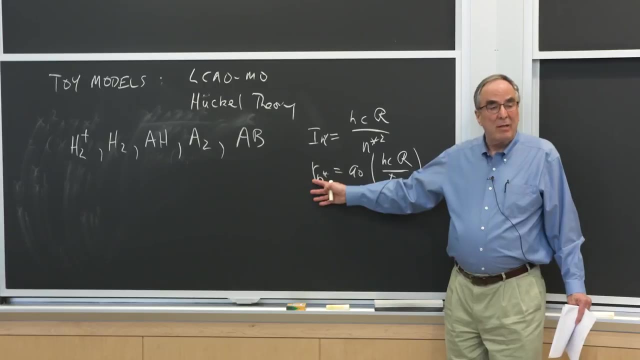 And then use that empirical principal quantum number to get the size of the orbital And basically the size is everything, Because everything is based on overlap And the inter-nuclear distance in a molecule is based on the relative sizes of the diatom. 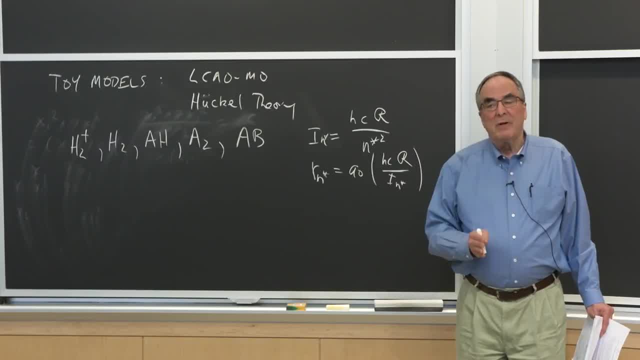 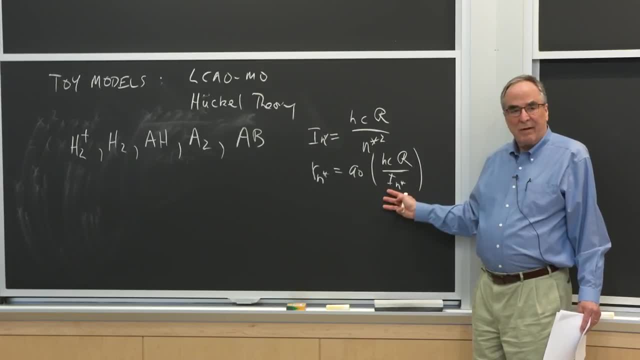 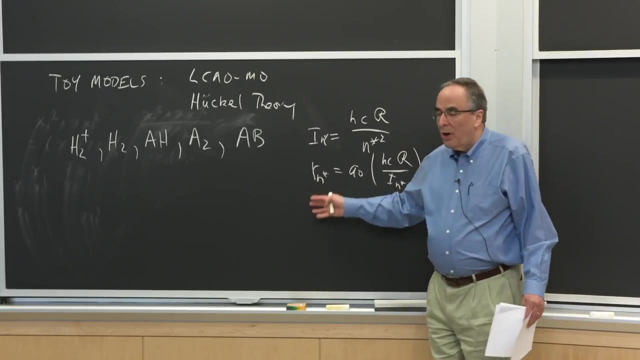 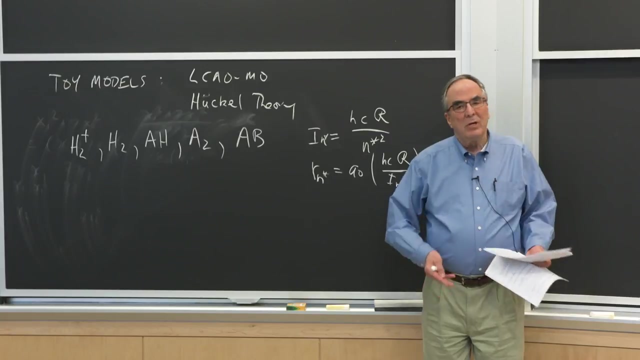 Different atoms And for different electronic states of the atoms. these sizes are different because they have the ionization energy from that level implicitly expressed. So because you know about orbital sizes and that the different atomic orbitals have different sizes, you can do an enormous amount as far. 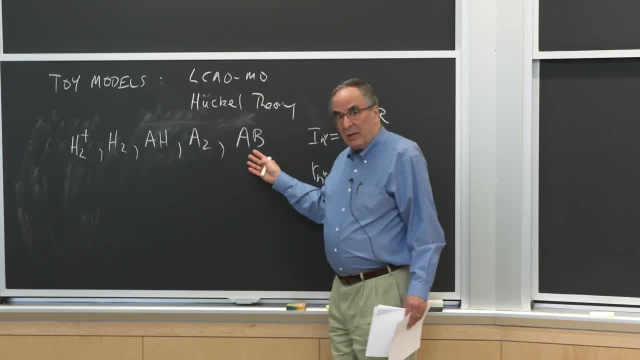 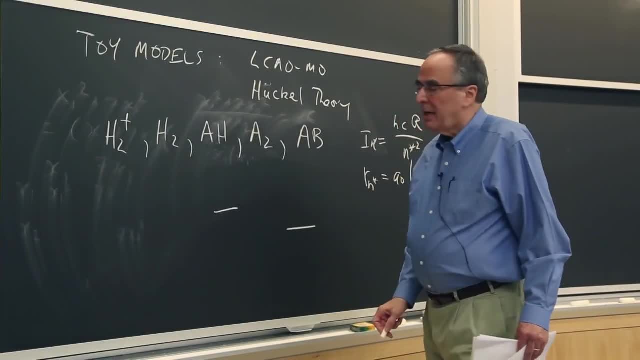 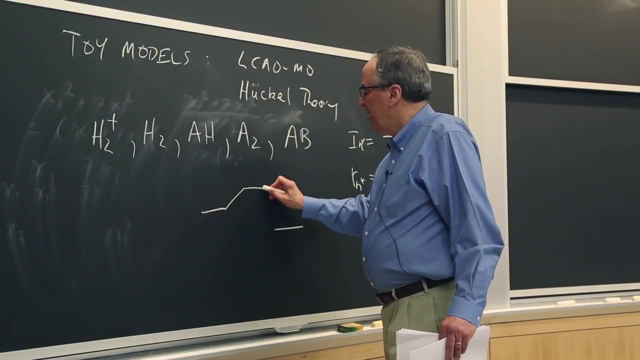 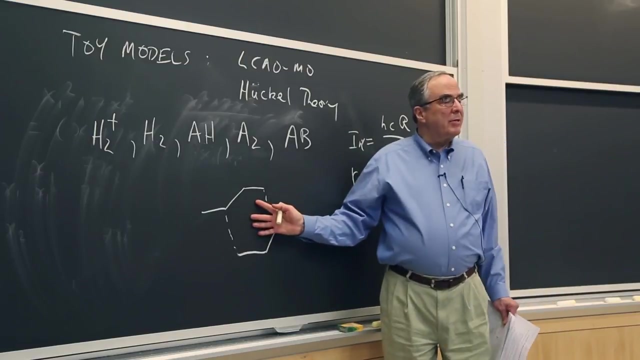 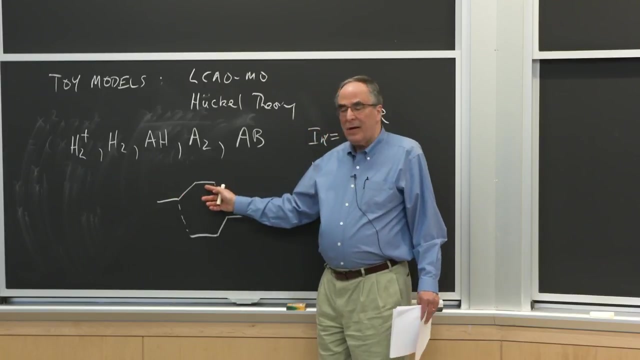 as understanding the electronic structure of, say, all diatomic molecules. Now this: when you have two states which have different energies, we do something like this to describe the molecular orbitals that arise from them. That's perturbation theory. So the solid line is the dominant character. 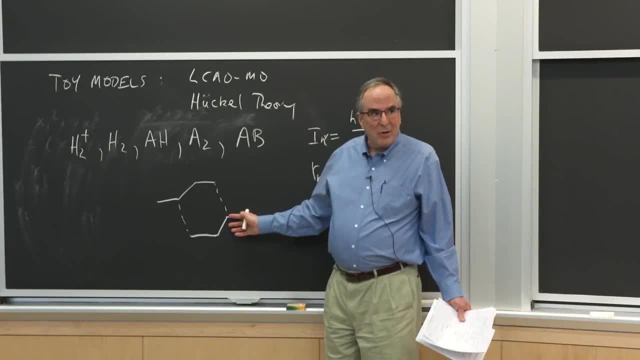 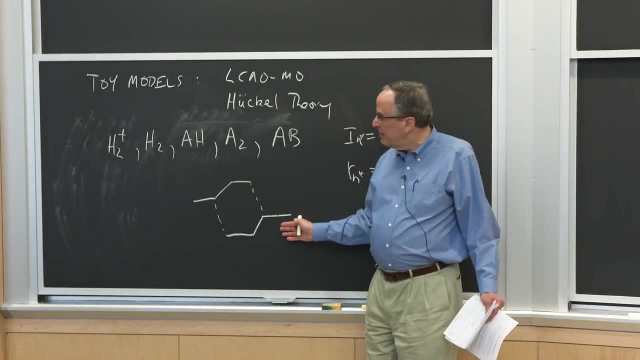 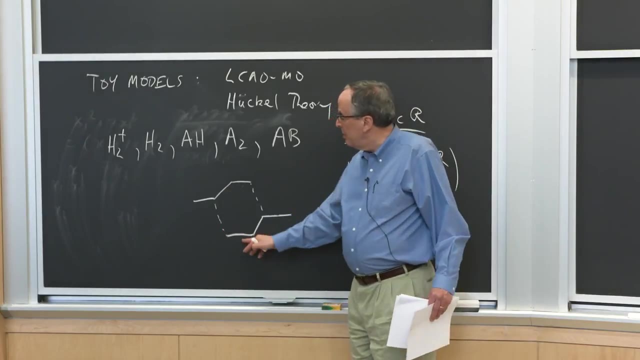 The dotted line is the admixed character of the other orbital, And this is all qualitative. but you have these different atomic orbital energies, You know them from the periodic table, basically, And so you can say: yes, an orbital. there's going to be two orbitals derived from these two states. 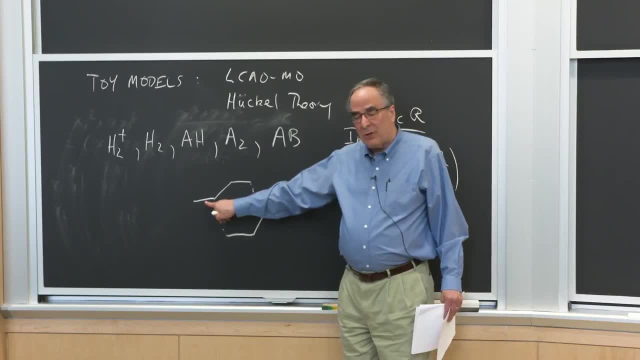 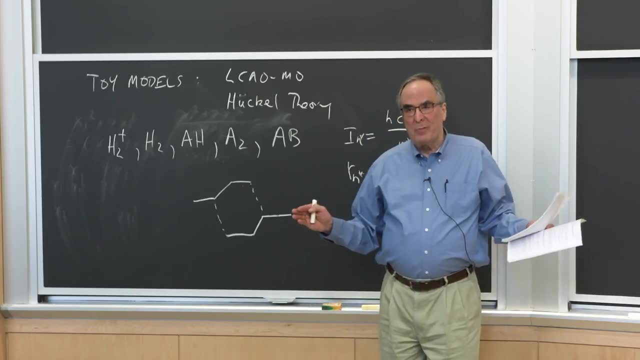 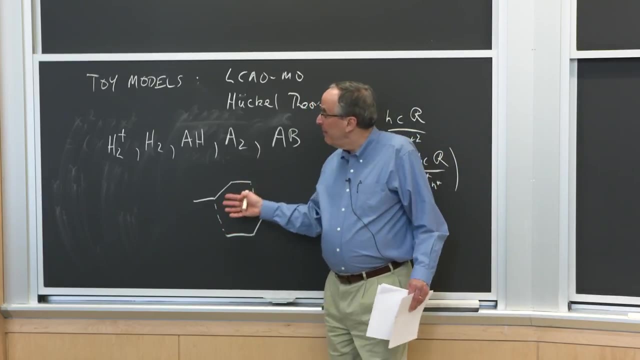 And one is polarized towards this atom, The other is polarized towards that atom, And so you get the orbital, The shape of the orbital, and it's actually useful for saying: well, is this if I were to do chemistry? 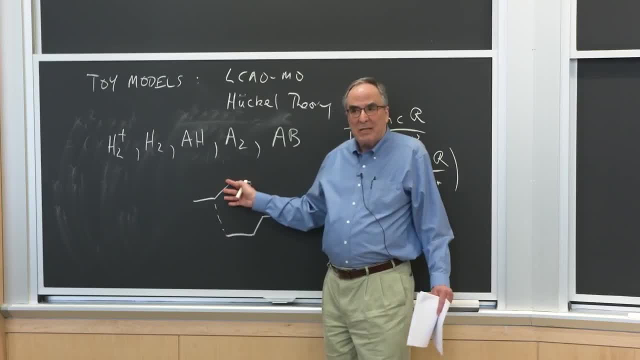 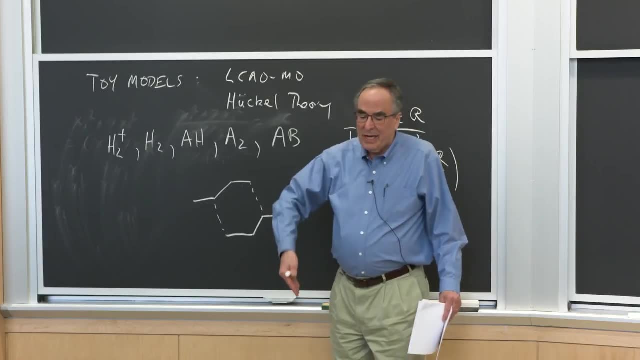 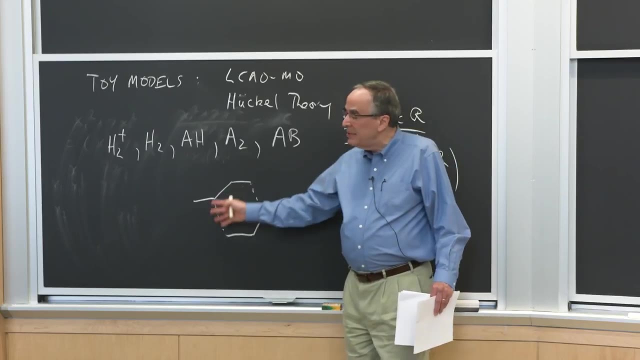 which end of this is electronegative and which end is electropositive, Or which end of this would attach to a metal surface. Would it attach pointing into the surface or lying down? And there's all sorts of insights if you can draw these sorts. 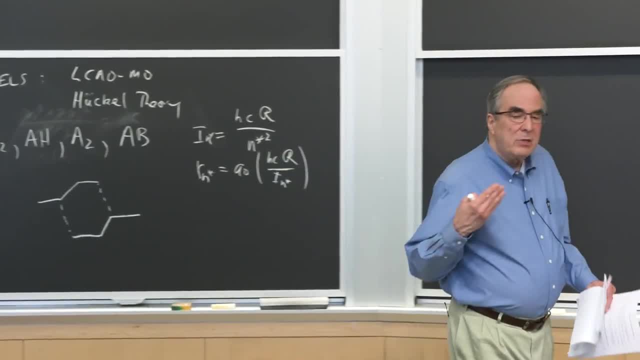 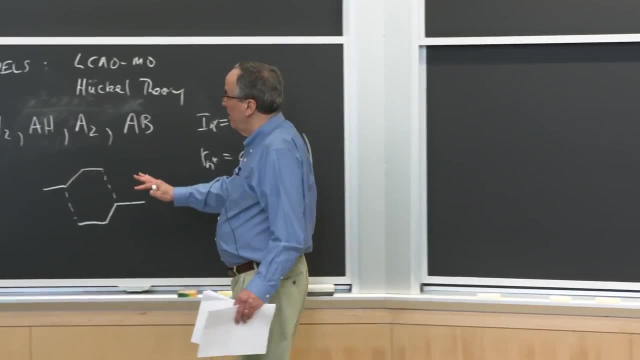 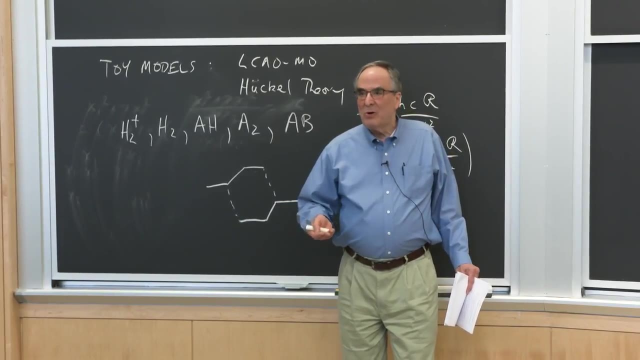 of pictures. And this is what we do as physical chemists: We take the crudest model and we say, OK, we understand the important features And as we discover new important features, we build them in Or we forget about them because they're too subtle. 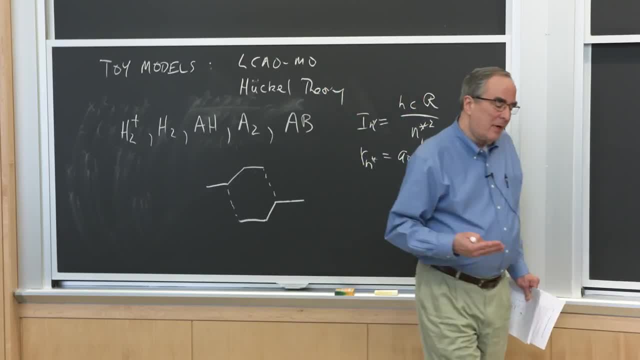 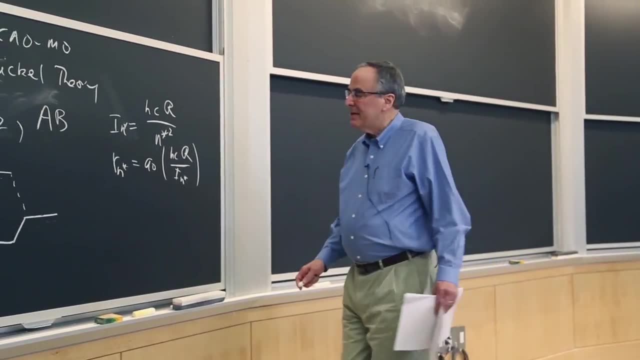 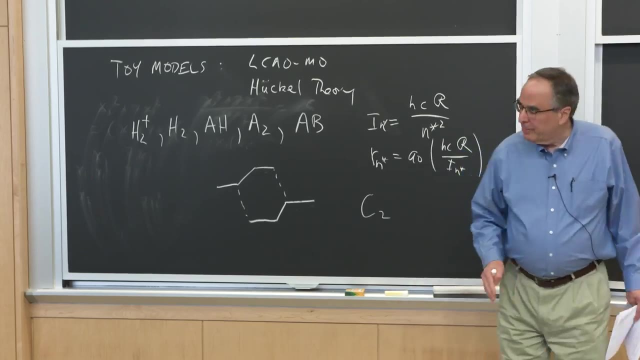 And we're always looking for something where the crude picture doesn't work and we then find the important thing that is needed. And, for example, if you were to look at the molecular orbital diagram for C2, which is a perfectly legitimate gas phase molecule, 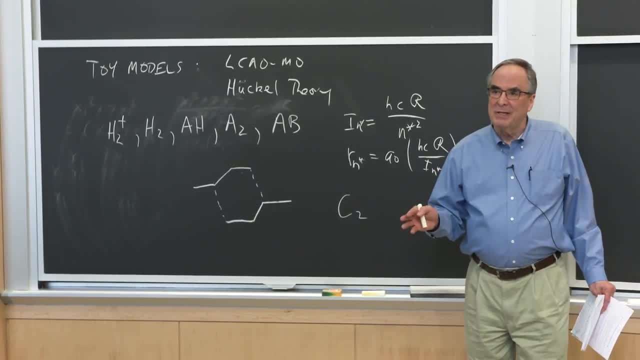 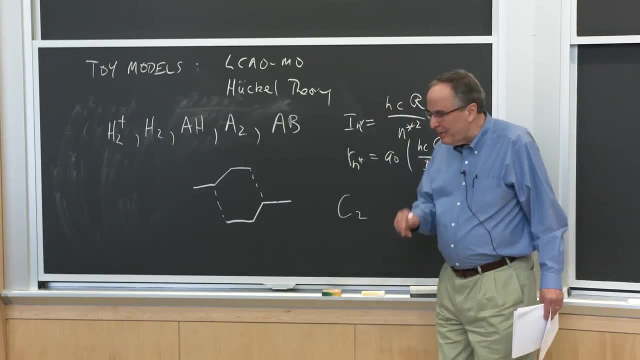 you'll see that there's a little bit of ambiguity about which is the ground state, And this is an important thing, And there was a big controversy about this. that was settled by spectroscopy, OK. So If you can build an intuitive picture, 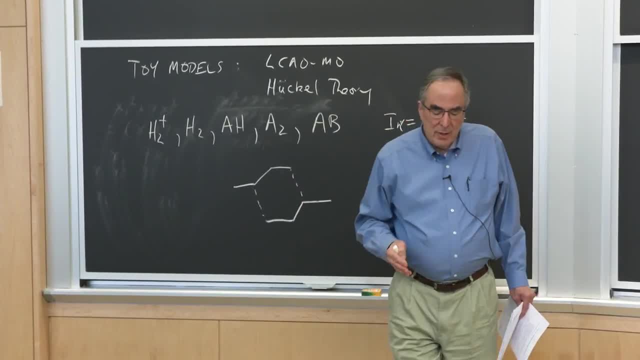 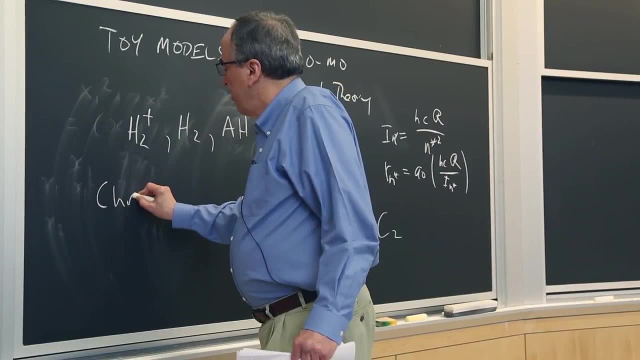 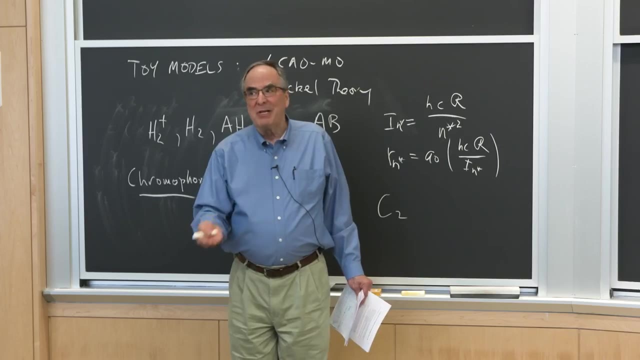 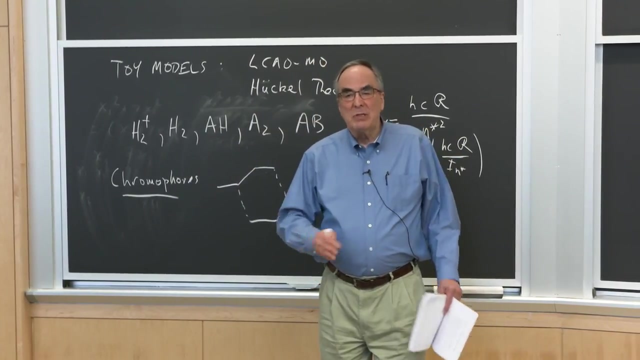 for all diatomic molecules. you can also build an intuitive picture for what we would call chromophores. So there are a lot of molecules that are larger than diatomic molecules, But the electronic structure is mostly nothing except a few atoms that are close to each other. 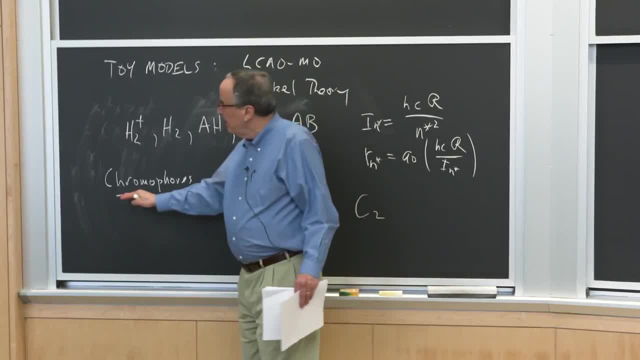 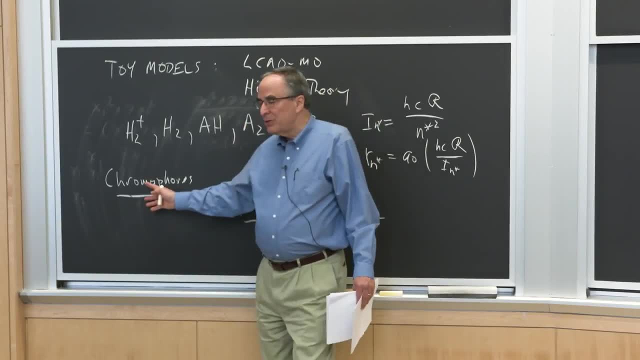 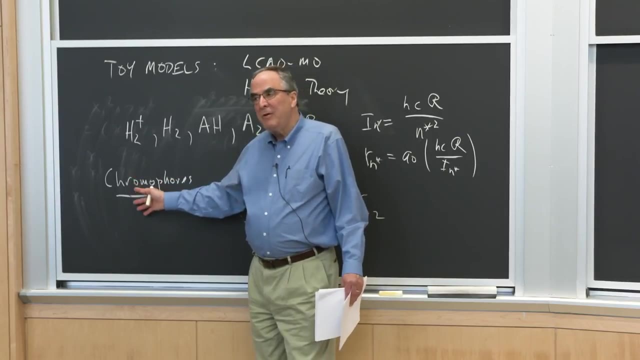 where there's a double bond or there's something special, And so if you can do LCAO, MO for diatomic molecules, you can also address electronic structure in much larger molecules, Because it's really due to a few important atoms or several different groups of important atoms. 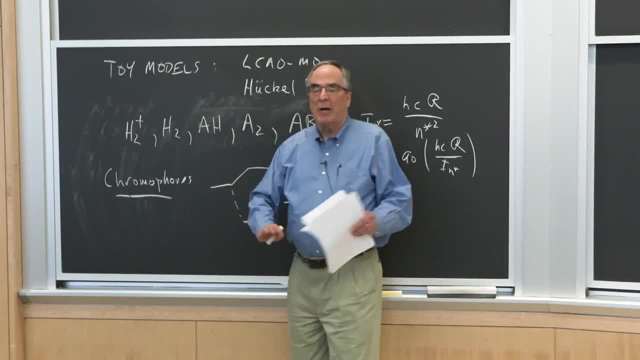 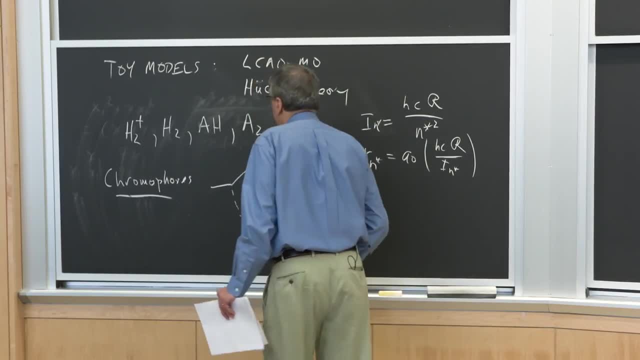 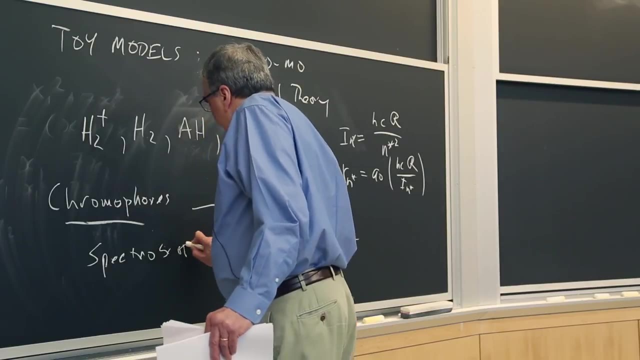 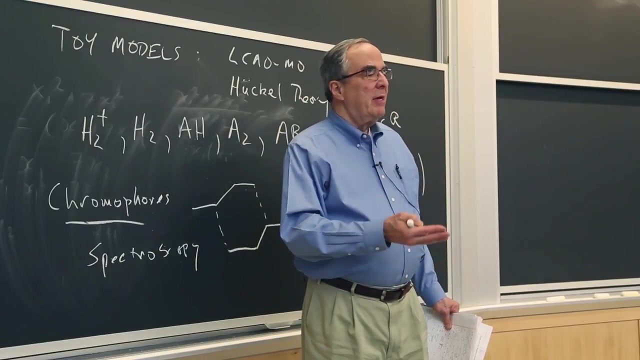 And the ideas in here enable you to talk about the electronic structure of almost anything, And one of the things that we care about is spectroscopy. How do we learn about the structure of a molecule? And mostly you learn about it from doing electronic spectroscopy. 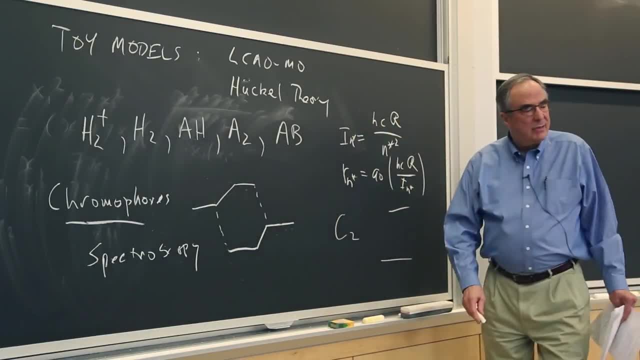 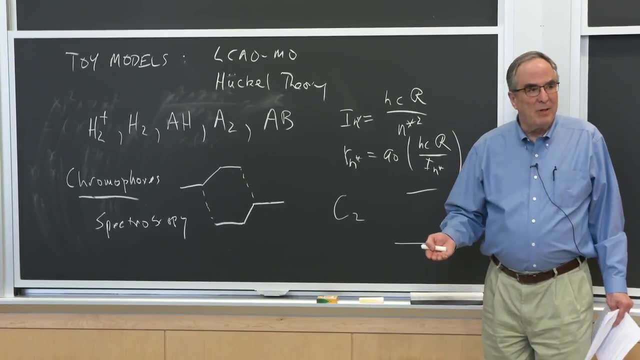 You do transitions between the ground state and some higher states And you want to be able to put it in the ground. You want to be able to predict what you're going to see And, for example- and I think you may hear about this a little bit- 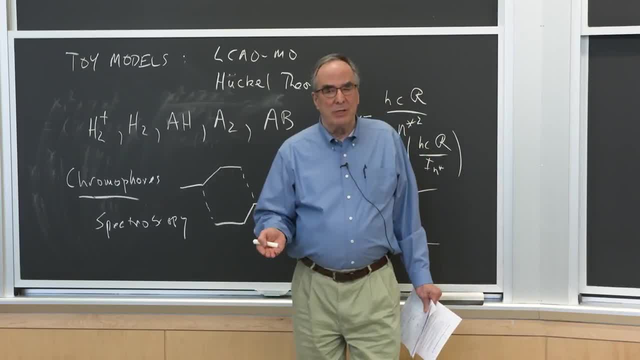 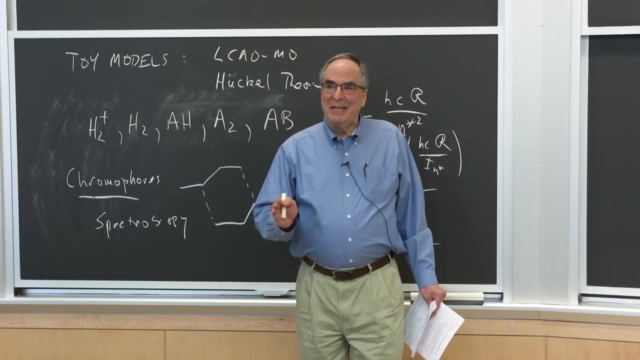 more if you know the spectrum of nitrogen. it doesn't start absorbing until far into the vacuum UV And then go one atom over the spectrum of oxygen. Well, that defines the vacuum UV. It starts to absorb around 200 nanometers. And that's the reason: It's the vacuum, It's the vacuum, It's the vacuum. Two and a half billion years ago, oxygen started to enter into the atmosphere and profoundly changed life on Earth. Because with the vacuum UV radiation nothing could live on the surface of land. Because it would all be killed by this hard UV, And so everything was under water at the bottom of the ocean. But all of a sudden, when oxygen came in, it was gone. When oxygen appeared, there was protection, And then there's additional protection farther out. 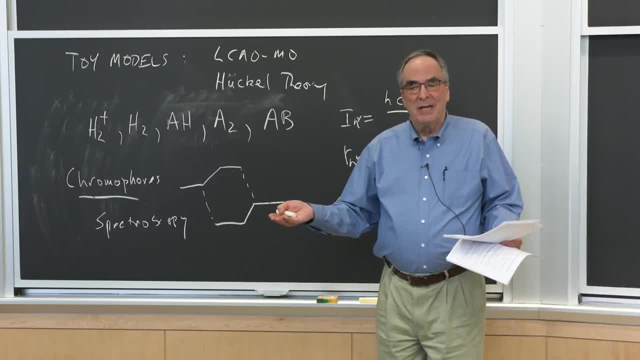 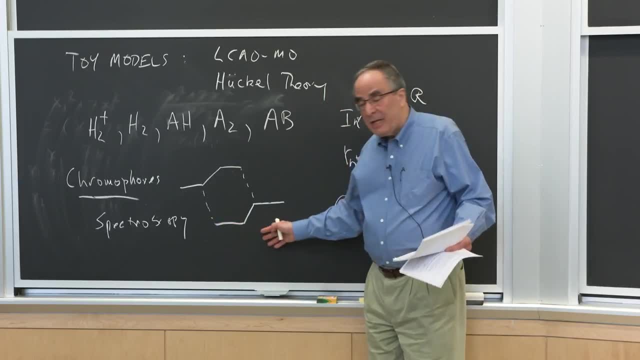 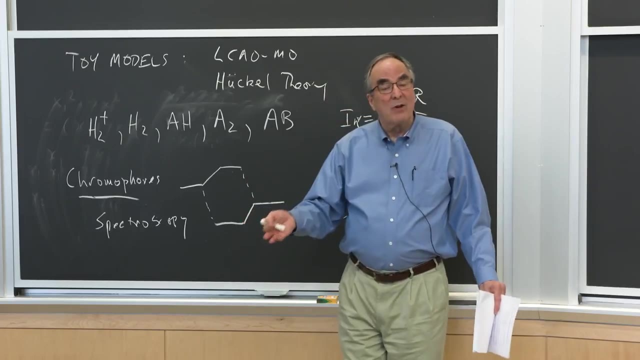 towards the visible from ozone. It's not such a good shield, but it absorbs between 200 and 350 nanometers And it protects us too. But the big thing is oxygen. And why should oxygen be so different from nitrogen? Why? 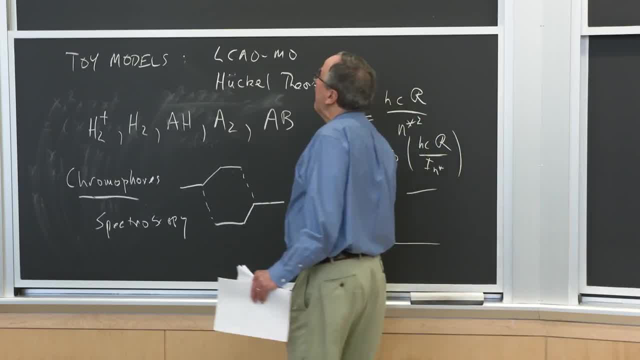 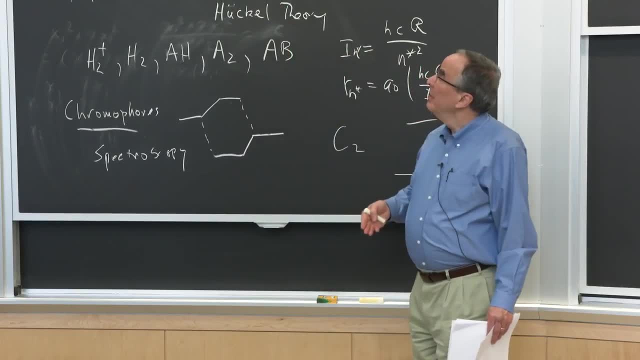 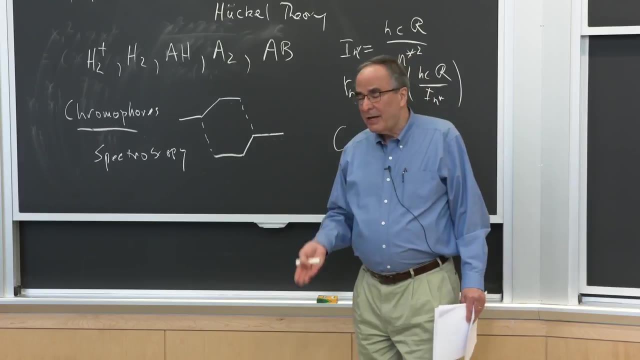 Why- And maybe you should think about that- I should have mentioned the schedule up there. I'm going to give another lecture on perturbation theory, one of my favorites, which I thought I wasn't going to get to give on Friday, And then Troy is going to give two lectures. 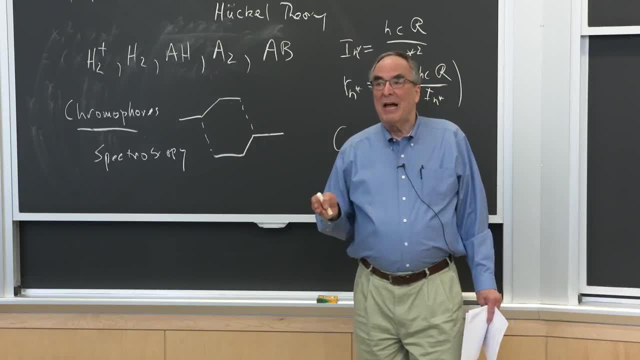 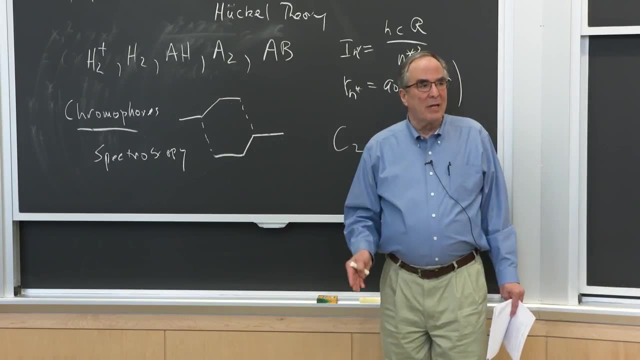 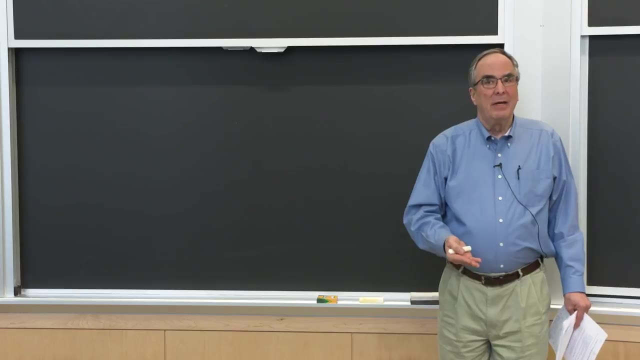 on quantum chemistry And there's going to be significant lab experience And you'll hear about that from the TAs And so you will do real calculations. So LCAO-MO is- it could be- the basis, the organization structure for quantitative calculations. 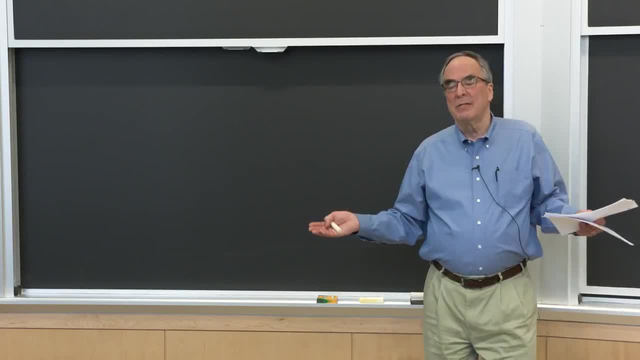 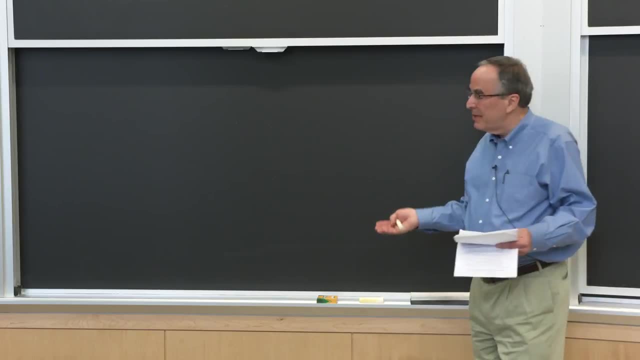 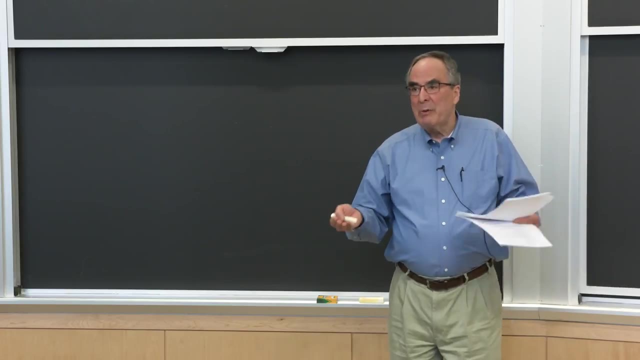 But quantitative calculations are usually huge basis sets And you lose the LCAO completely. One could take the results of such a calculation and then project it onto a LCAO-MO basis- Right, Right Picture, And that's generally what we do. 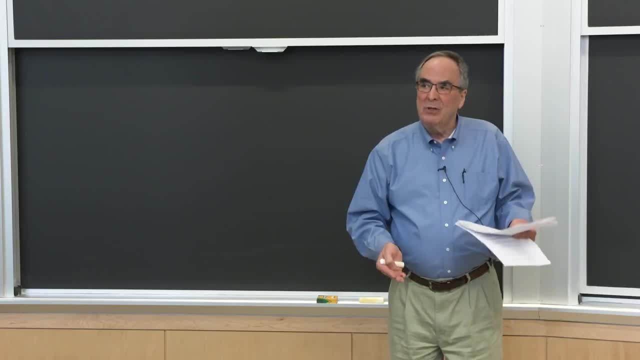 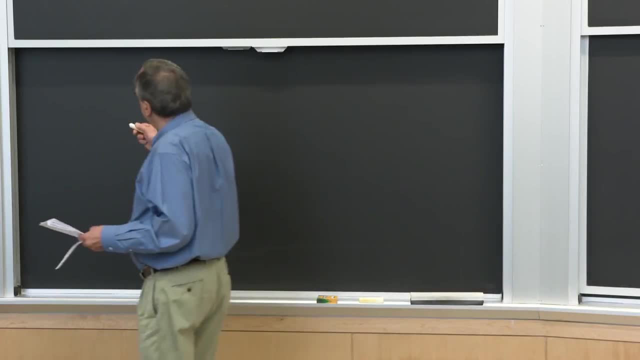 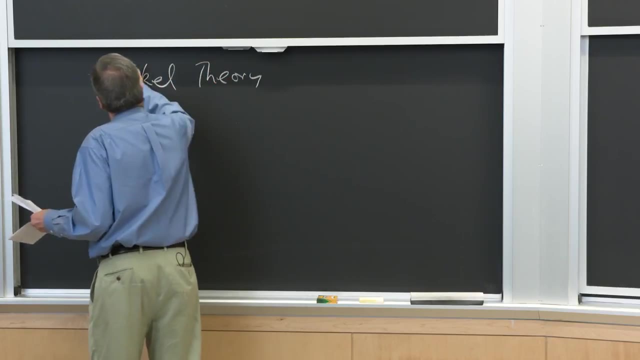 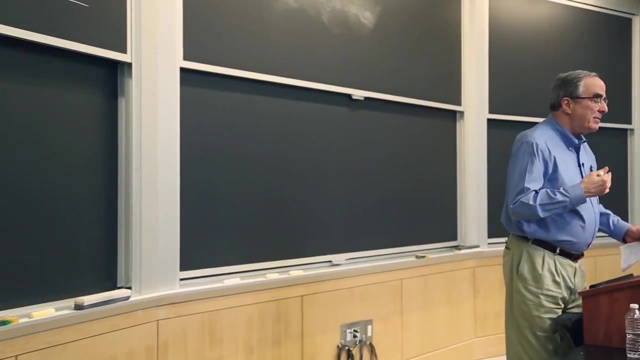 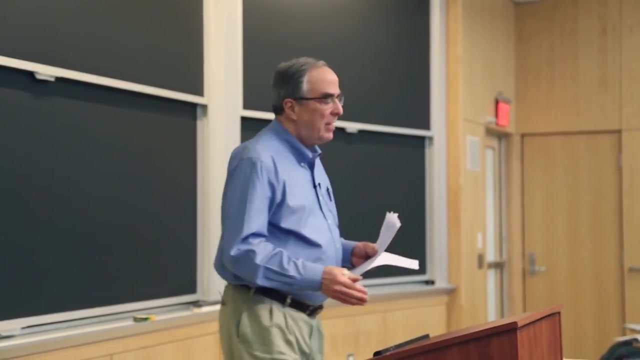 We reduce experiments, We reduce theory to something that we can intuit, And it's really important to have intuition. OK, Huckel theory. Huckel theory is another kind of non-rigorous theory, Right Rigorous theory, In fact. it's laughable in its simplicity. 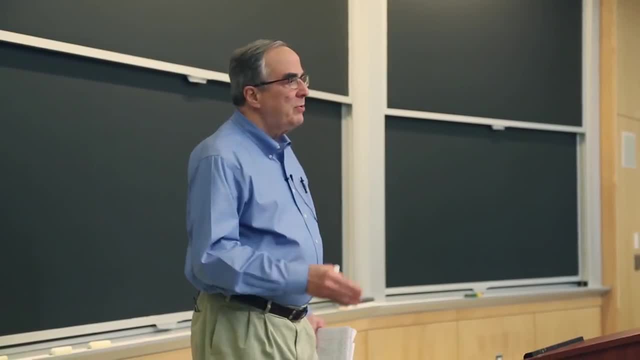 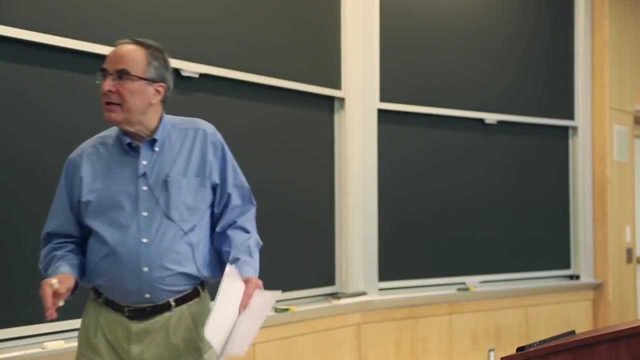 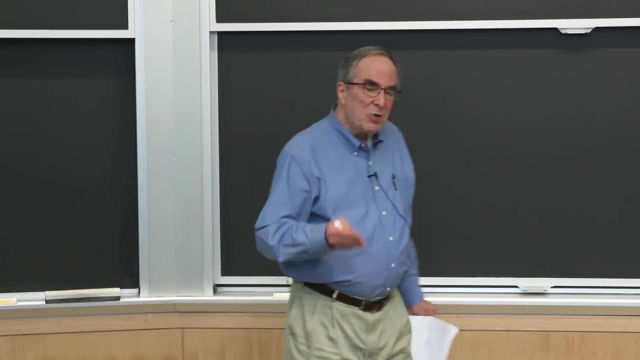 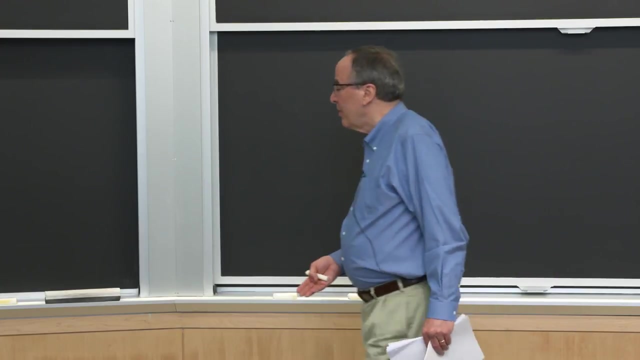 And the idea is that even such a crude theory can make sense out of huge families of molecules and enable you to be quantitative about things without having to do a huge calculation. Now, you almost always have to diagonalize a matrix Because usually in Huckel theory, 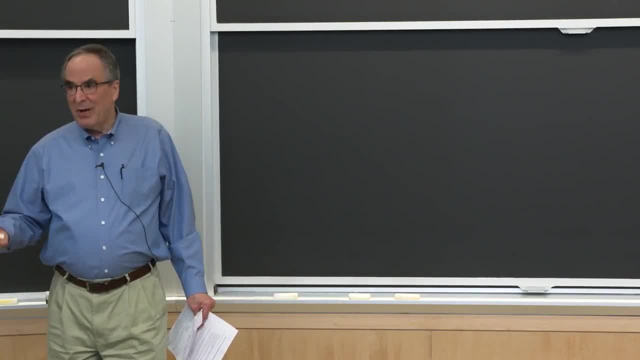 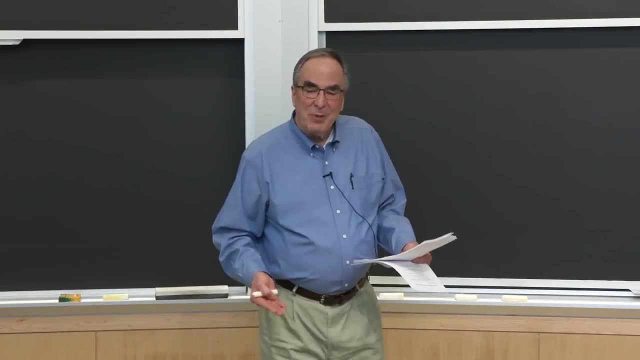 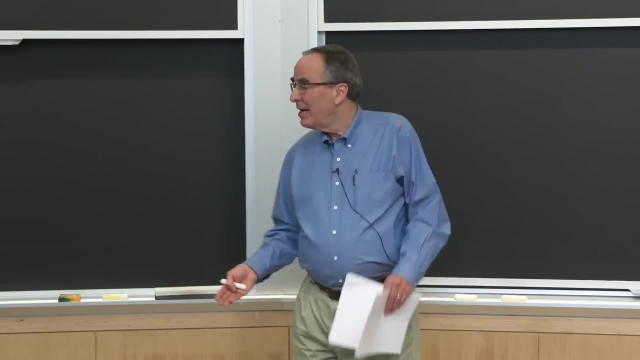 you're dealing with more than two or three relevant orbitals. It's a big deal. I don't know whether you have experience with matrix diagonalization routines, but there are many of them And you're going to have experience with them, But the things you put into them have absolutely nothing. 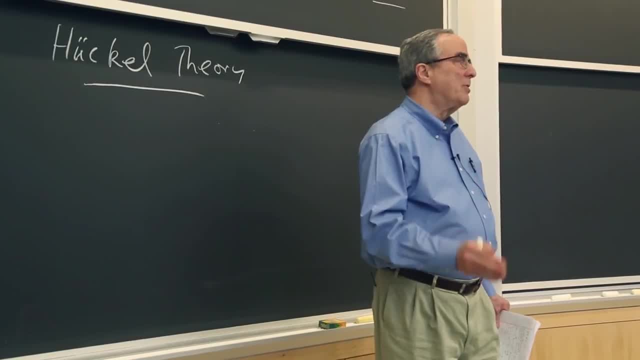 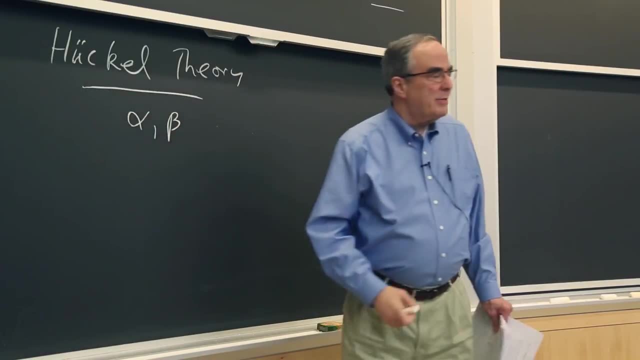 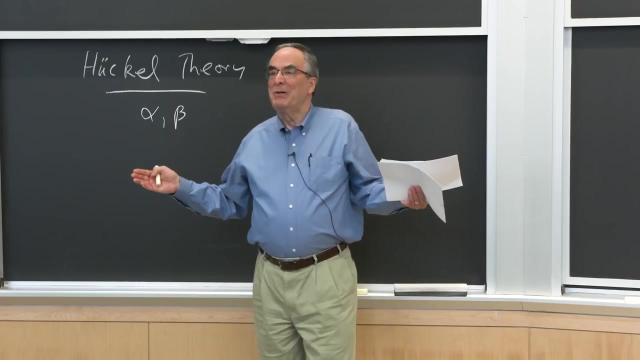 to do with a real Hamiltonian. It's a make-up picture. It's a picture based on basically two parameters, alpha and beta, And I'll talk about this. And these are parameters that are sort of agreed upon by international committee. It's not a committee, but people say OK. 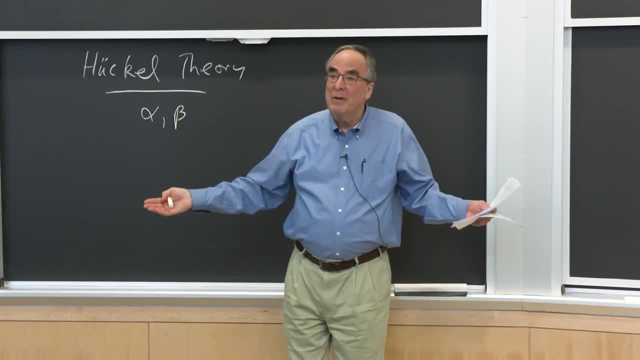 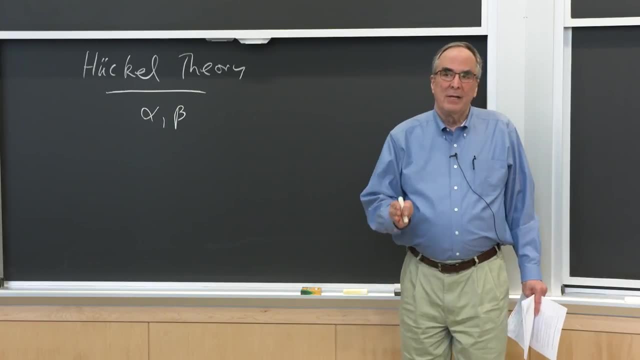 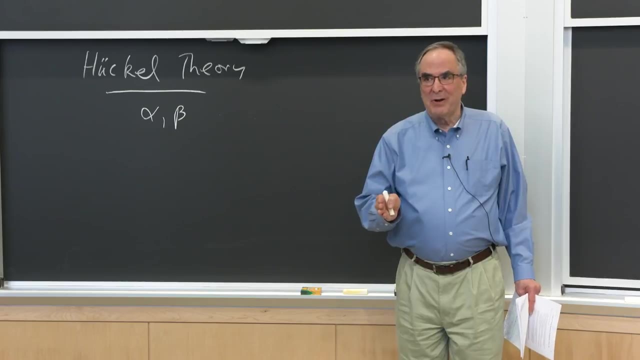 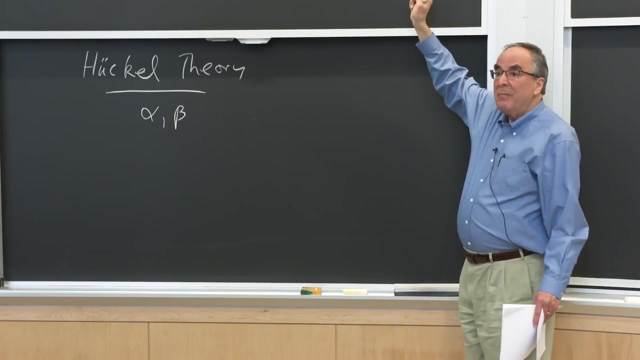 this is the value of alpha and beta that we're going to use to describe many problems, But I do. I just want to make sure you understand that Huckel theory is only a little bit more ridiculous than LCAO MO theory, Because in LCAO MO you really have some semi-empirical sense. 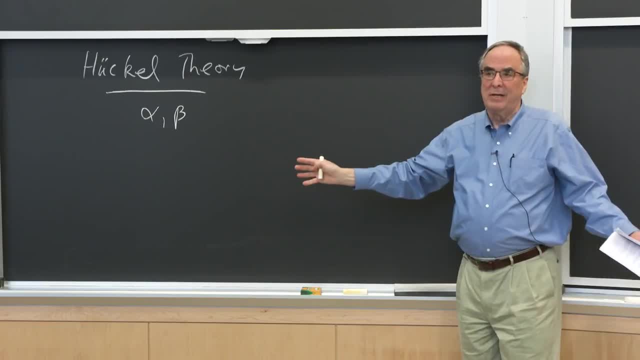 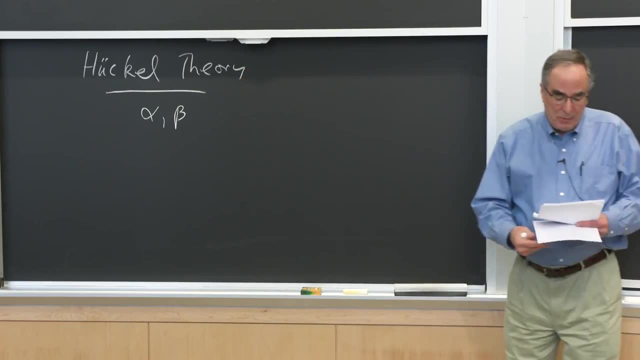 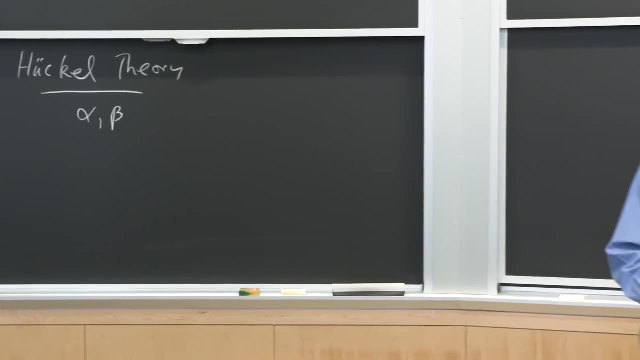 of how big orbitals are, And once you know how big orbitals are, you know what's going on In this. you just have a couple of parameters that says, OK, these are the rules, Let's now apply that. OK, don't carry around too much stuff. 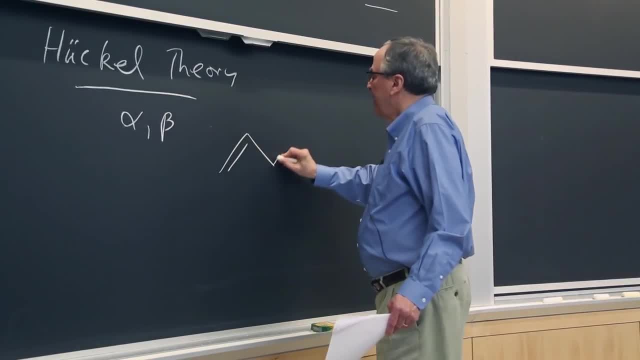 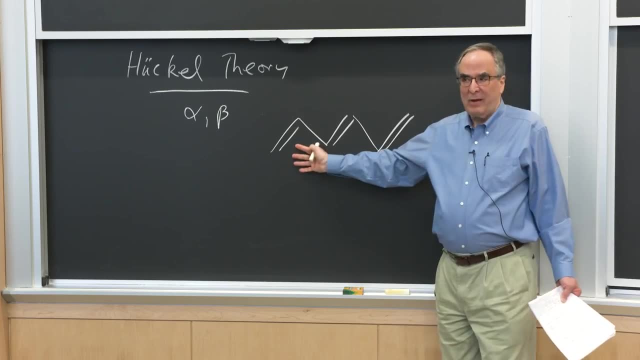 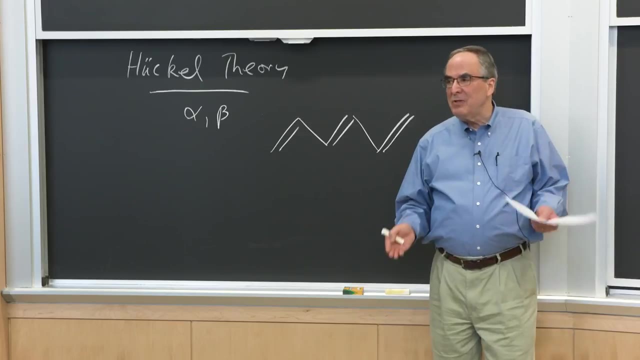 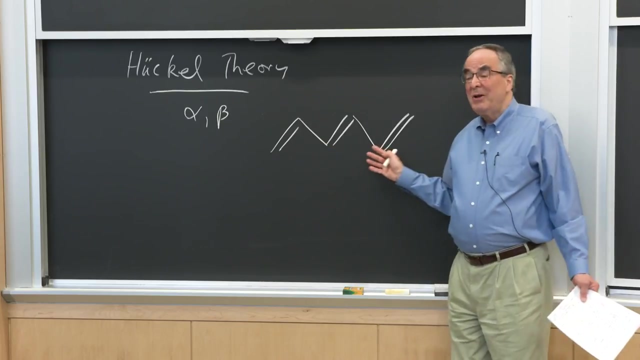 So organic chemists are really wonderful because they give you an abbreviated way of drawing a molecular structure, And almost everyone in this room is gifted in being able to visualize three-dimensional structures. Physical chemists tend not to be so gifted, But here is something where we don't have any hydrogens. 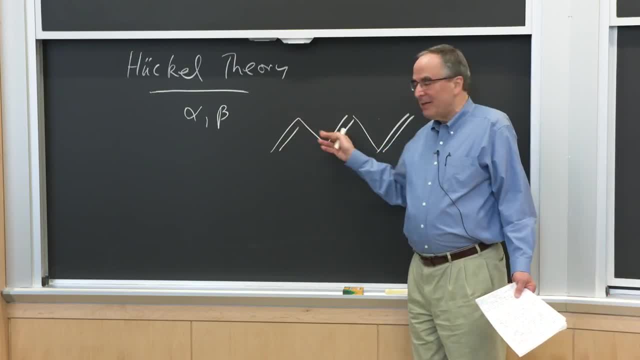 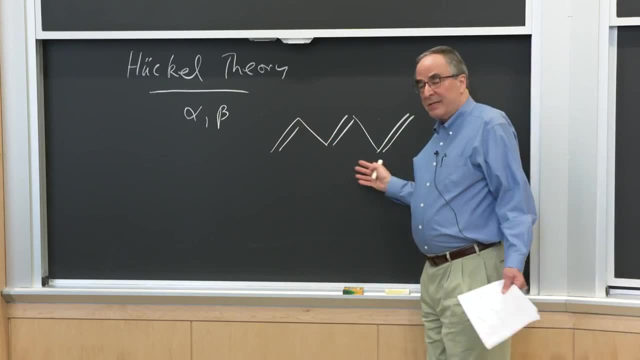 I mean, there are hydrogens, but they're implied And we don't put carbons here. We just say, at every vertex there is a carbon atom, And so we consider these things, And every organic chemist knows if I draw something like this: 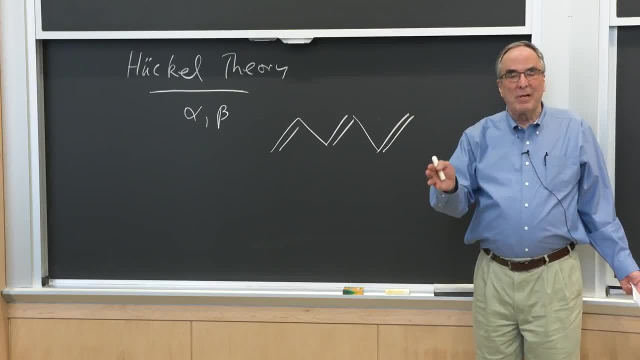 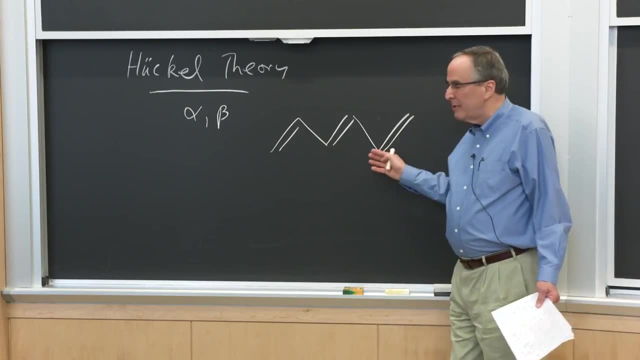 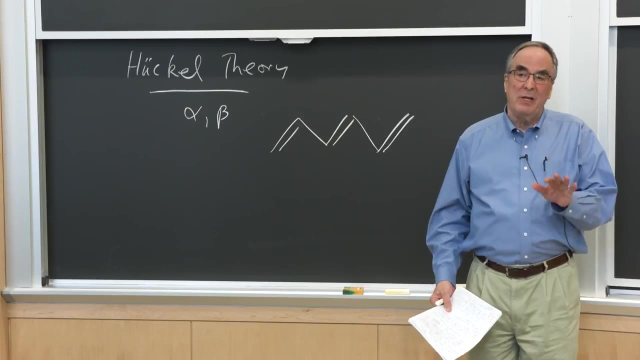 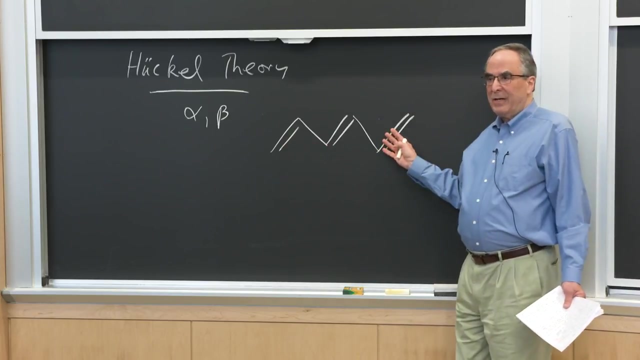 that either I was stupid and I drew something that was impossible, or what the structure is OK. now, this is a conjugated system. We have double bonds and single bonds, And that kind of thing is known to be unusually stable, And in order for it to work, it has to be planar. 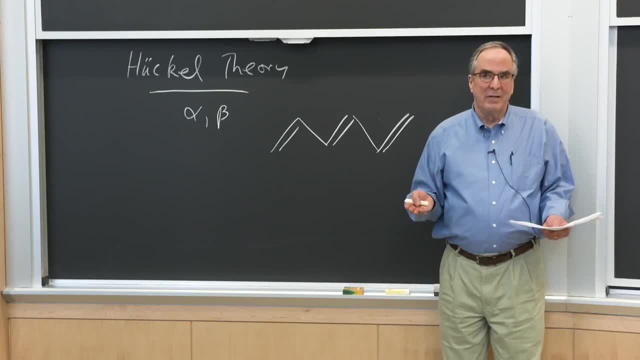 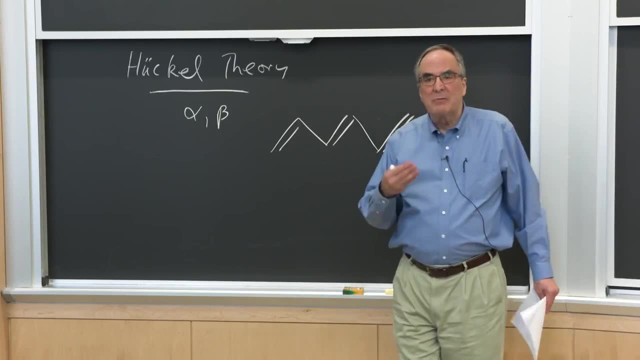 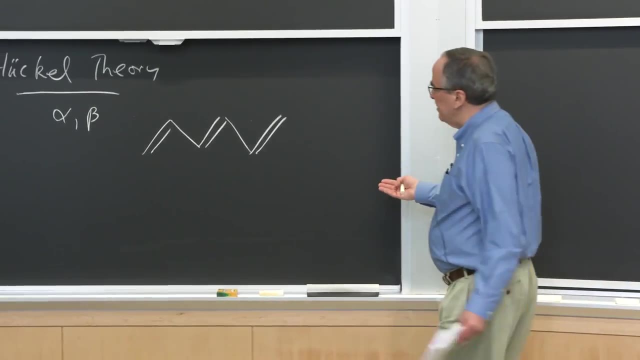 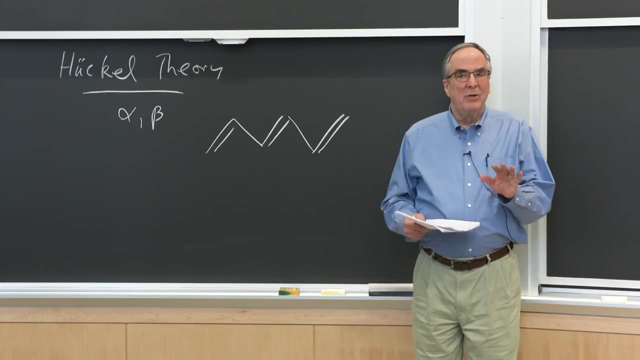 If you have a conjugated system which is not planar, then it's not as stable. So this is based Local theory is based on the existence of unusual stability of conjugated systems, And it can be extended to non-conjugated systems. 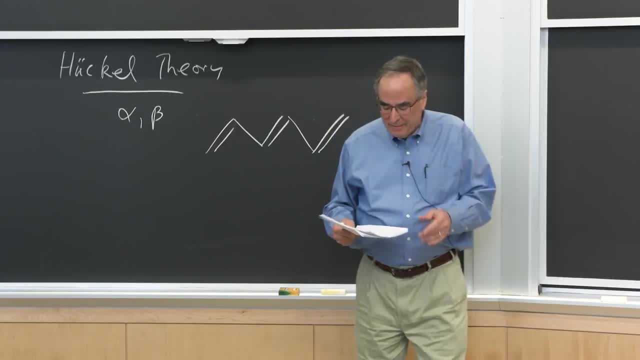 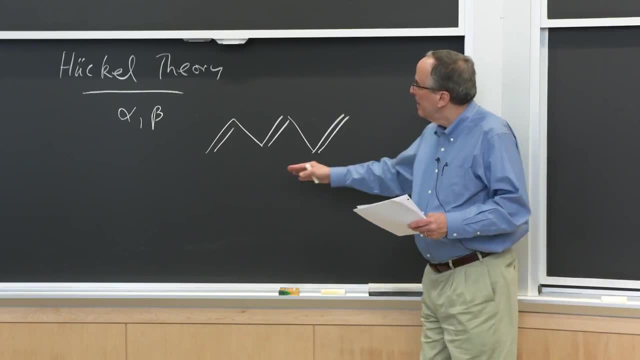 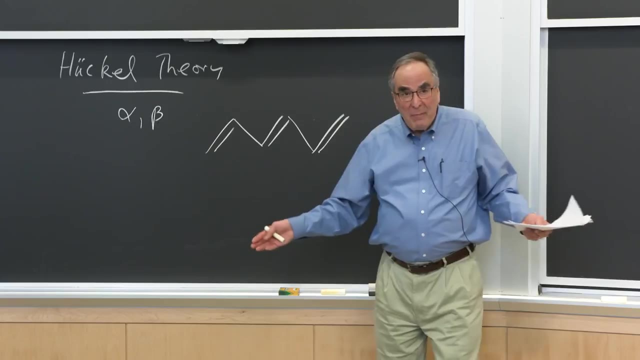 to non-planar systems And we have rules for how to do that. But the simple rules are: you start with a picture And you can write down a Hamiltonian And it's a toy model, but it's still something that the computer has to diagonalize. 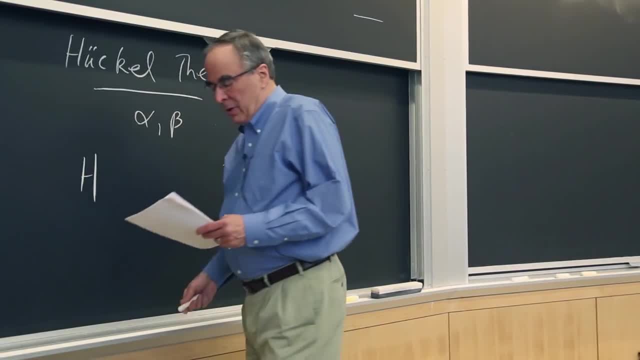 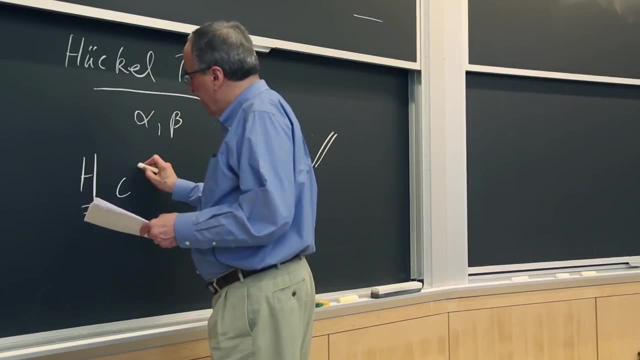 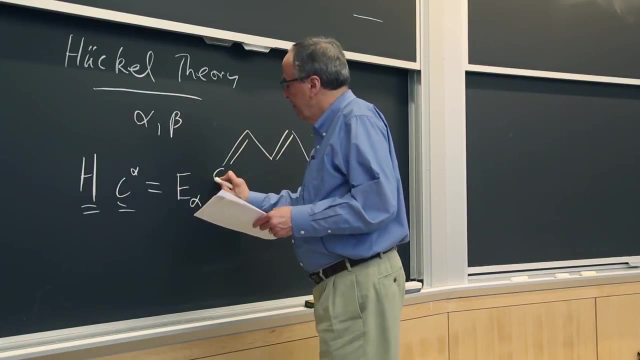 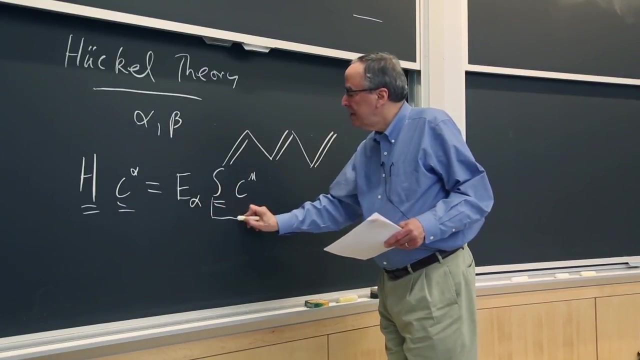 So when we're doing a variational calculation expressed in matrix language, we have a Hamiltonian matrix, We have eigenvectors And we have eigenvalues, And we have the overlap matrix And we have something where this is C alpha, where here we 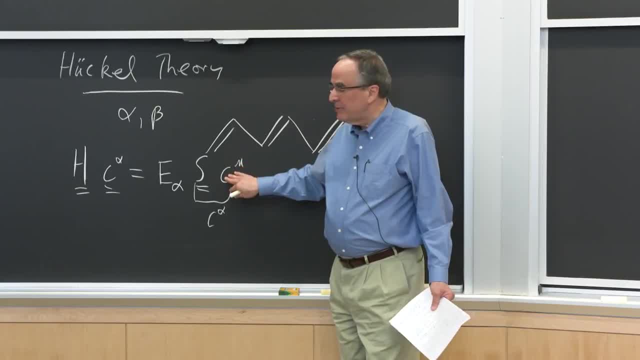 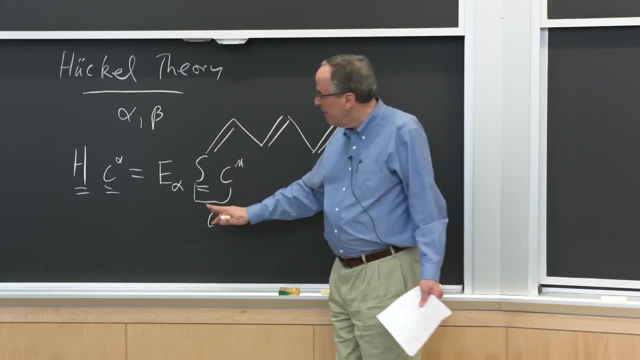 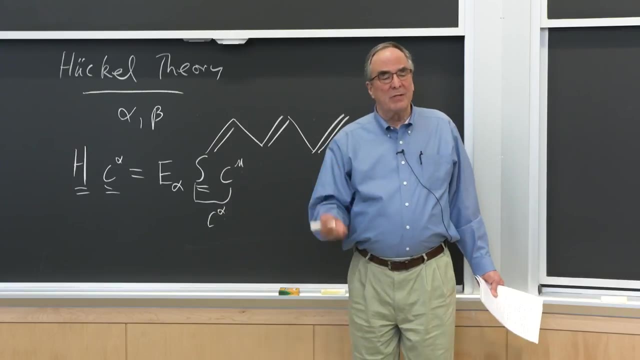 can have non-orthonormal basis functions And this makes them normalize. So these are the normalized, Ortho Normalized basis functions or basis vectors, And this is the kind of equation we have to solve. It's the generalized eigenvalue equation. 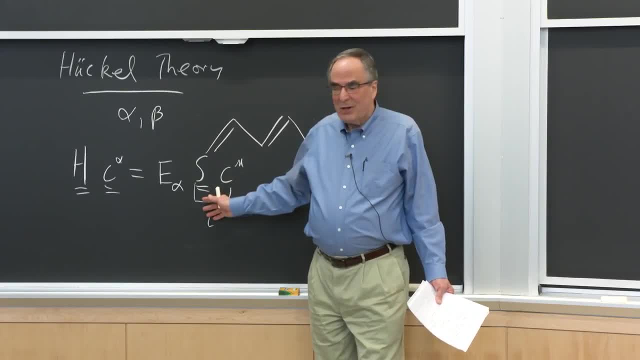 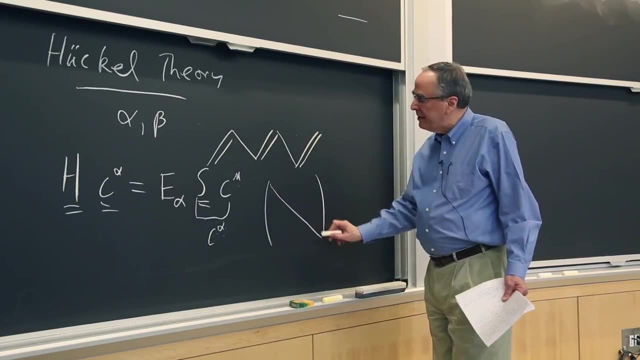 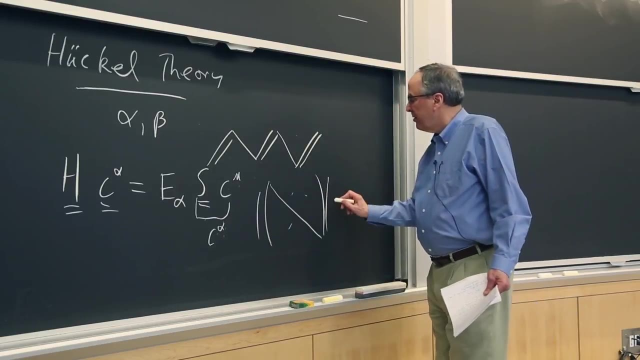 And we don't like this because it doesn't have the simplicity of just a Hamiltonian, where we have matrix elements along the diagonal and somewhere else And the idea is we want to take the secular determinant and make it 0. By 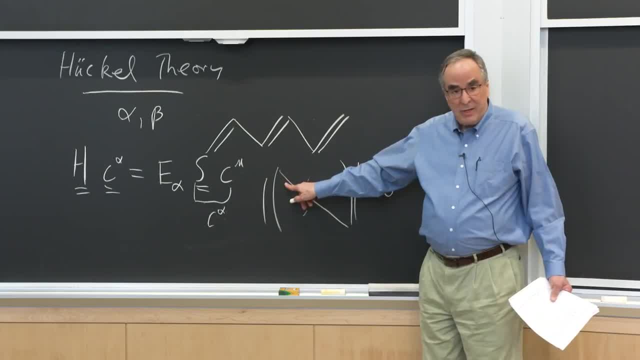 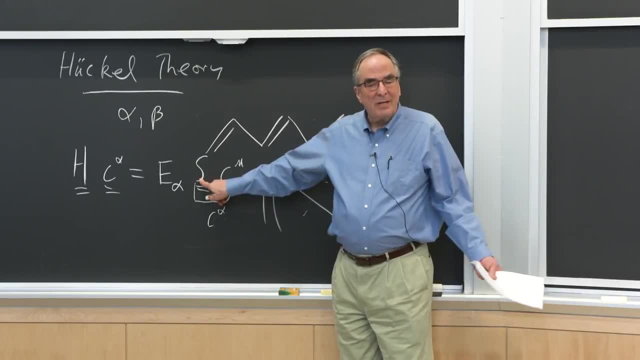 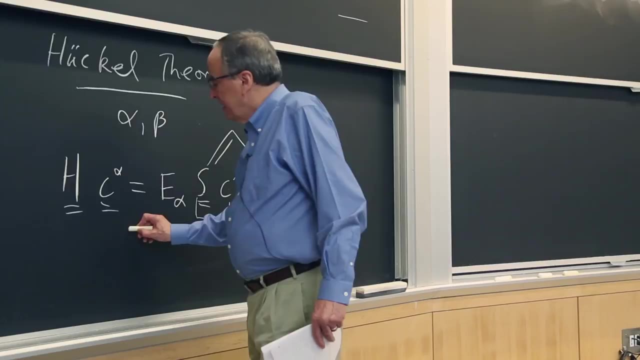 By adjusting values of the energy differences along the diagonal. But when we have this overlap matrix it's complicated. Now there's a way of dealing with the generalized eigenvalue equations, But one way to deal with it is to say S is equal to the unit matrix. 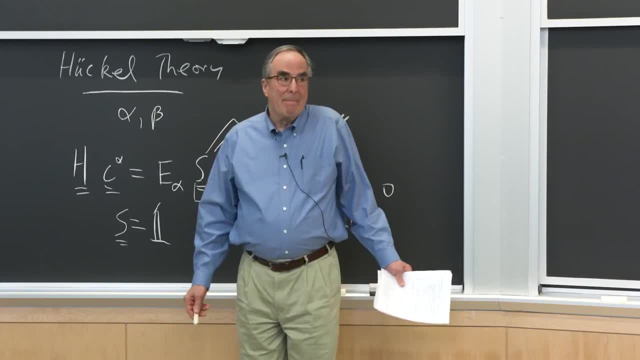 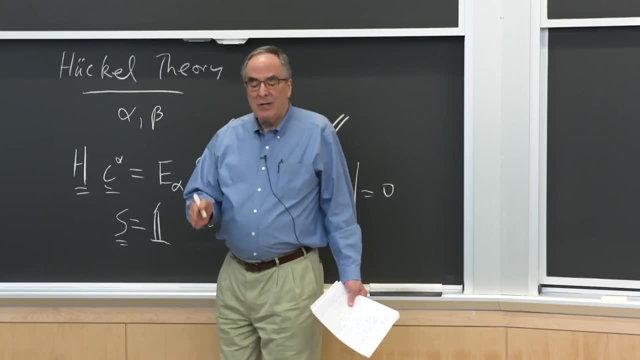 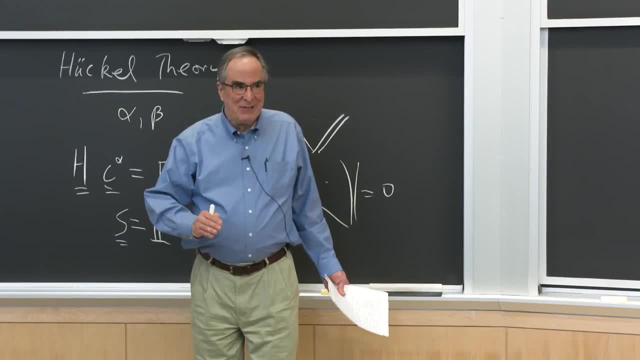 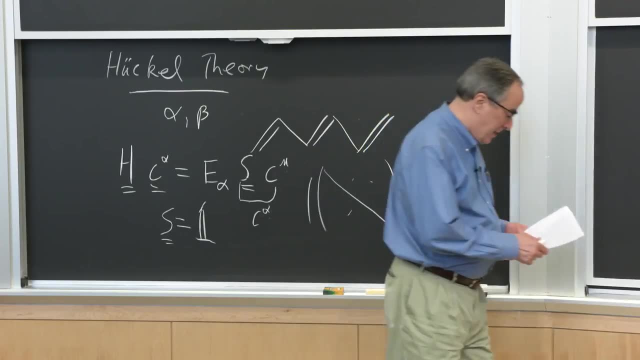 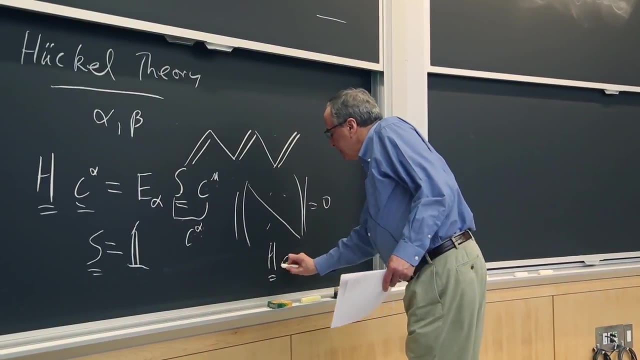 We're going to neglect it and then we're going to bring it back if we need it. But it's a wonderful simplification because it enables you to write down a simple, effective Hamiltonian which looks just like Hc. alpha is equal to E. 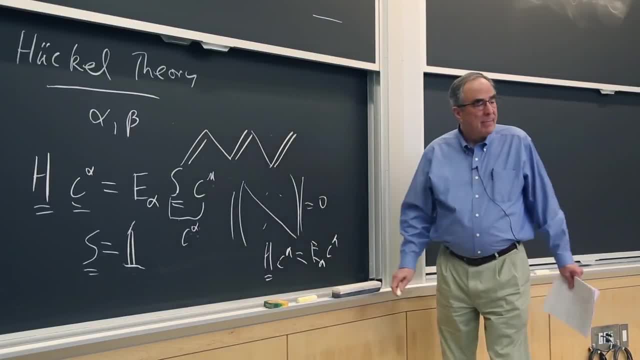 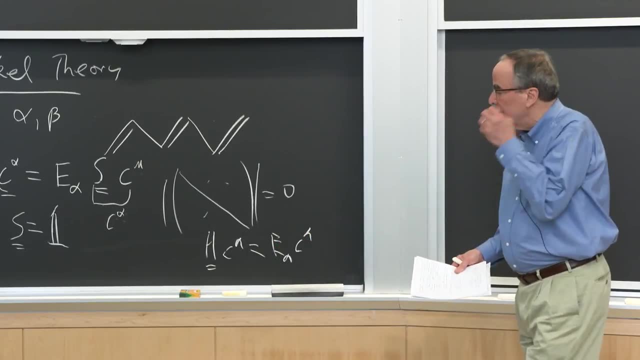 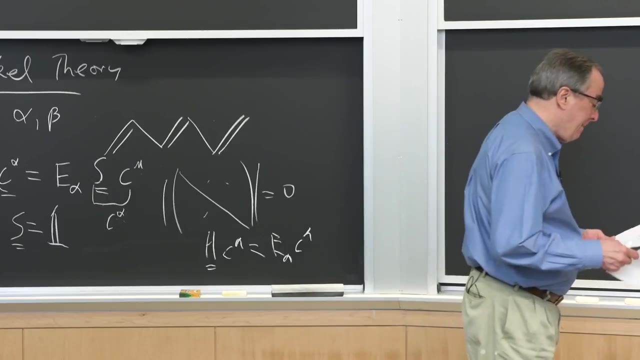 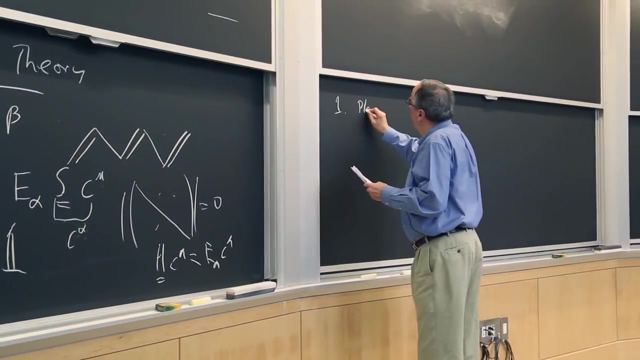 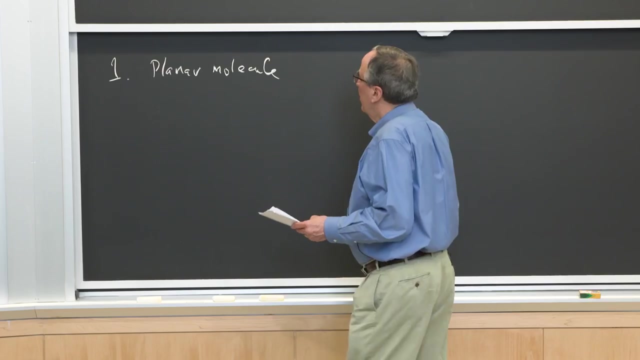 E alpha is equal to C alpha. OK, This we know how to solve And we can use the same procedure. OK, So these are the rules. If we have a planar molecule, we can say there are p orbitals, one on each carbon atom. 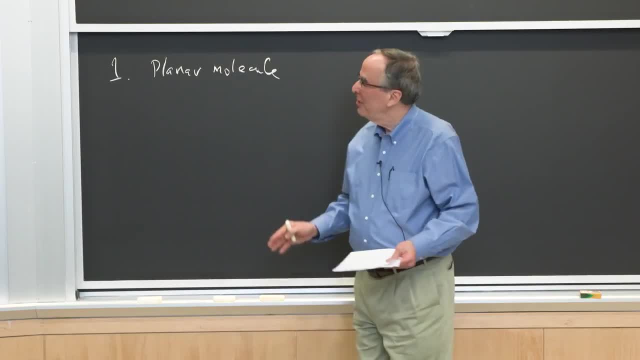 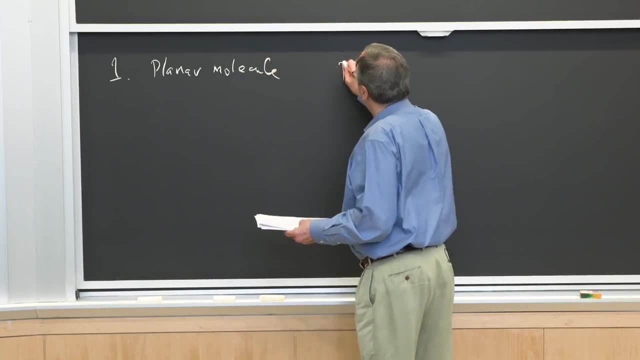 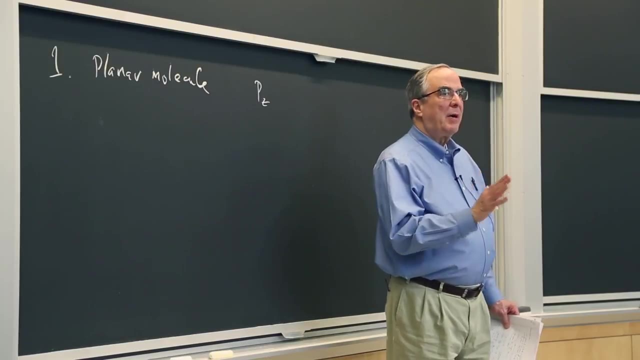 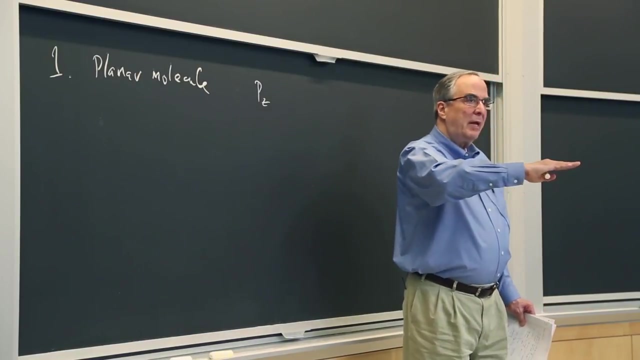 or one on each atom- that's not hydrogen- which are perpendicular to the plane of the molecule. So pz orbitals- And those are special- They give rise to pi bonds. Pi bonds are bonds where there is one plane of symmetry containing the bond. 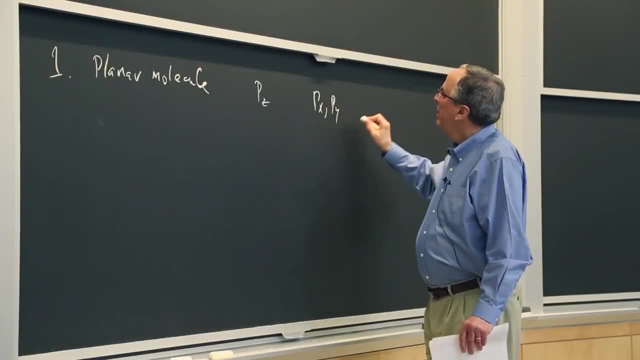 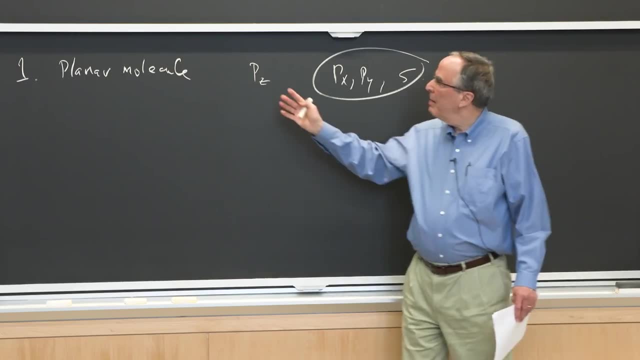 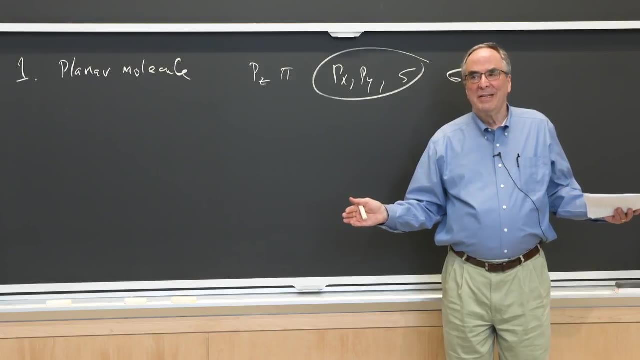 And then there are px and py and s, And these give rise to sigma bonds. So we have pi bonds and sigma bonds. Never the twain shall meet. And we don't care about the sigma bonds, because anybody can make sigma bonds. 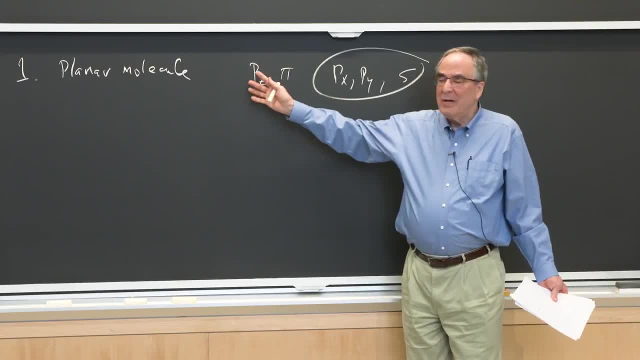 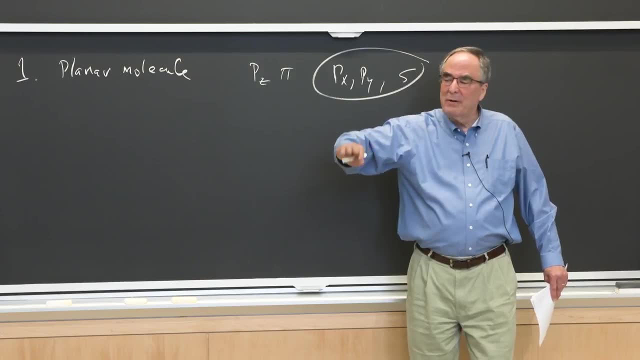 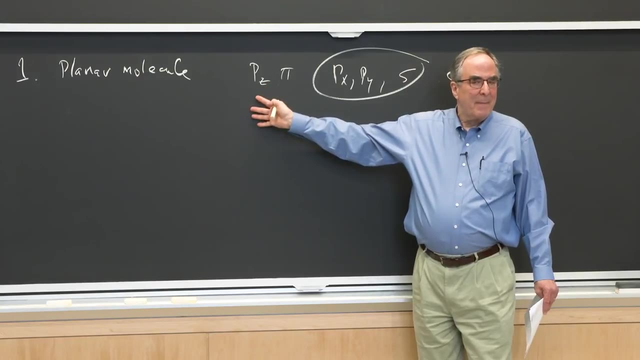 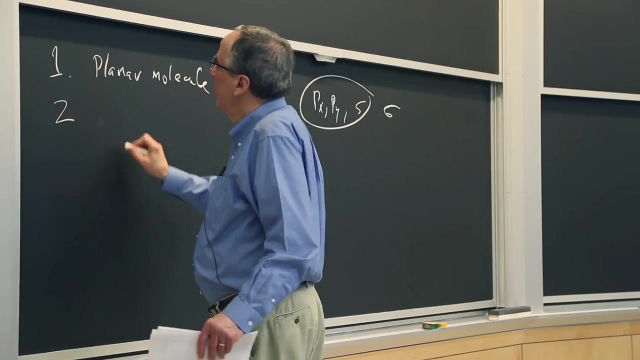 but only the special perpendicular to the plane guys, which are responsible for the fact that the molecule likes to be planar, And so we're only going to consider these pz orbitals, One on each atom, So we don't care about pi sigma interactions. 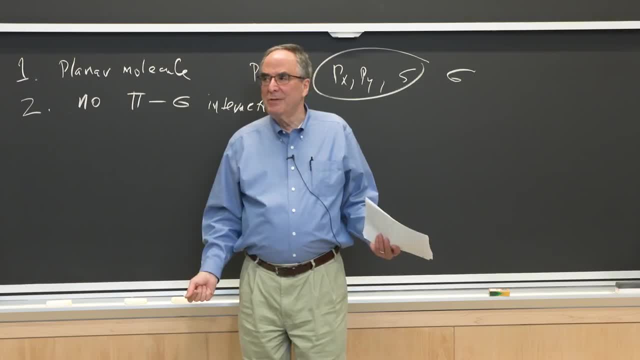 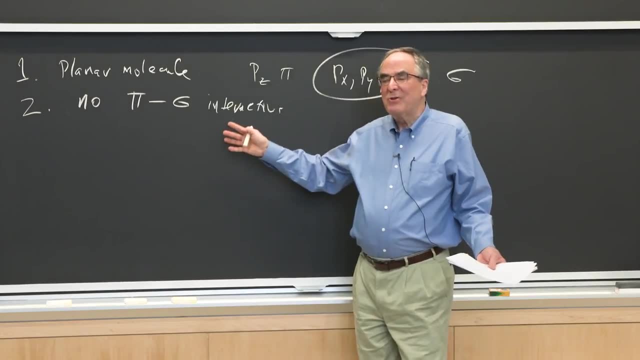 And we're going to neglect the sigma orbitals, because they take care of themselves And we can do anything we want. It's just a question of if we make two of them, we're going to lose them. OK, I think too many ridiculous assumptions. 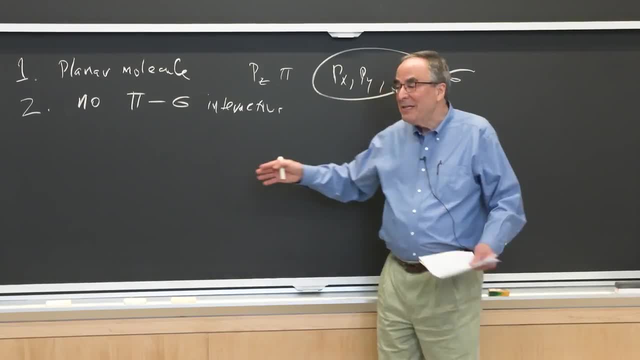 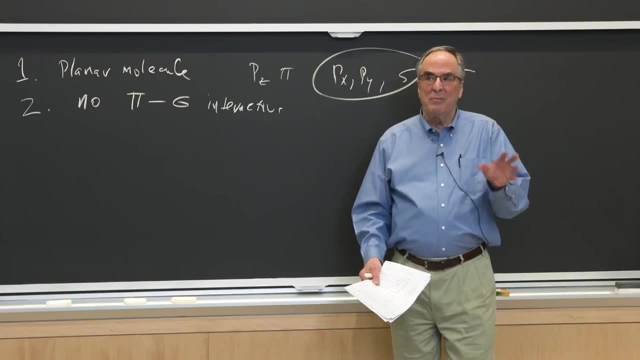 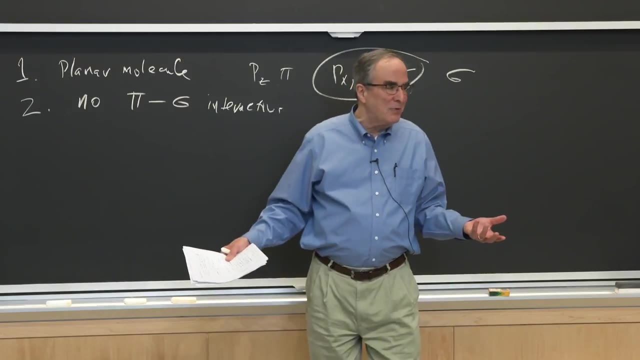 will get ridiculous results And this has been time tested And it gives pretty useful stuff And it provides a framework for making arguments about molecular structure and molecular reactivity. And in organic chemistry you learn about resonance forms And this is compatible with generating the resonance forms. 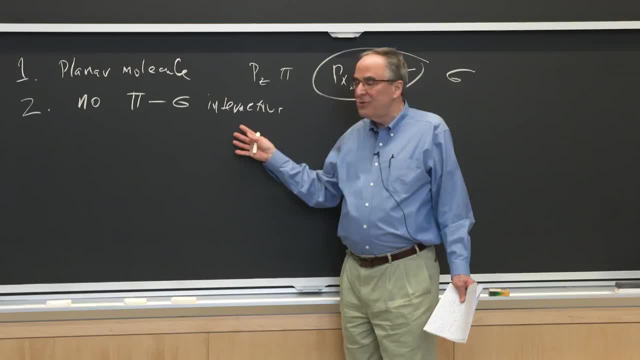 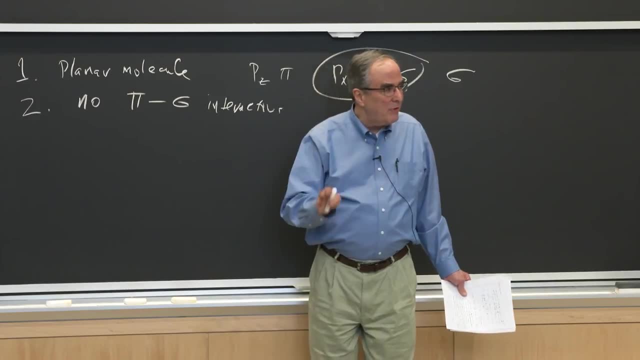 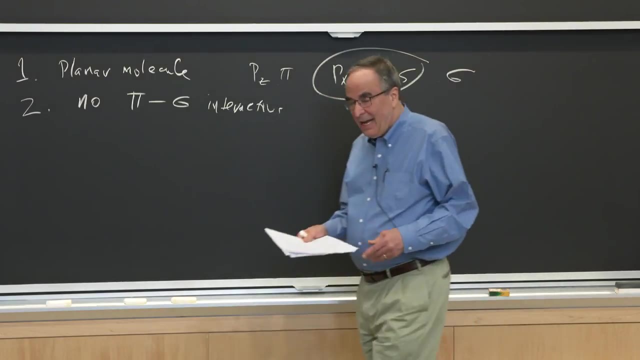 and saying what is the relative importance And what is the charge, distribution and bond strength And strength and everything like that. So it's really useful using the most primitive tools that organic chemists introduce at an early stage in your education, And that's one of the reasons why a lot of people 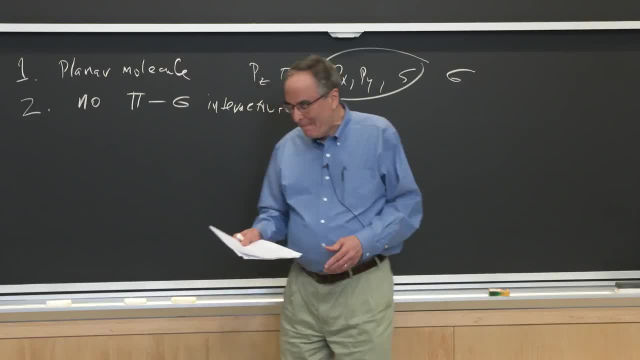 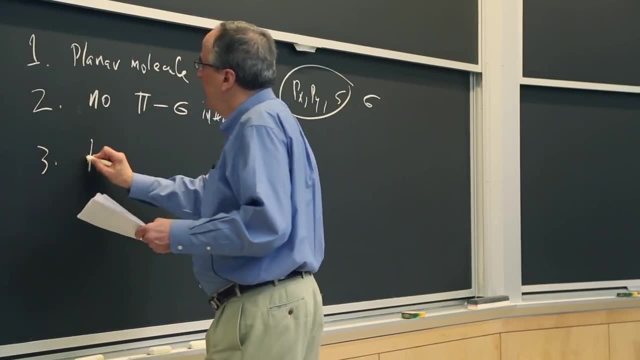 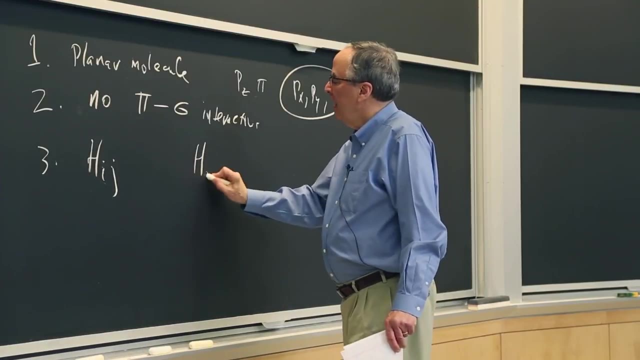 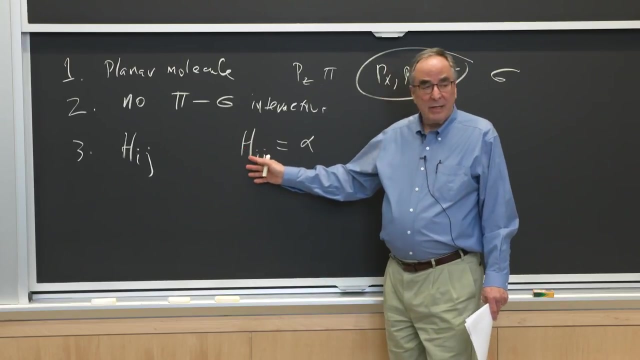 become organic chemists because it's so beautiful. OK, So our H-I-J matrix, So we have a bunch of matrix elements And we say, OK, H-I-I is equal to alpha, So every carbon atom has its alpha value. 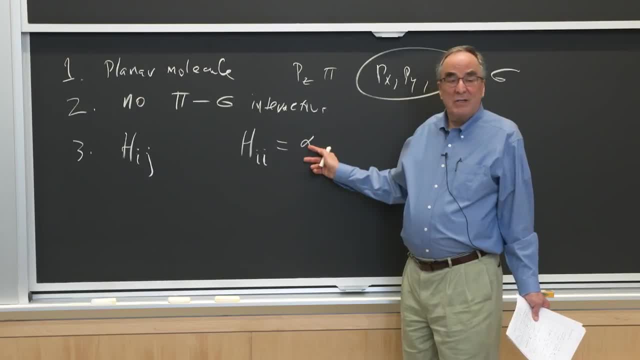 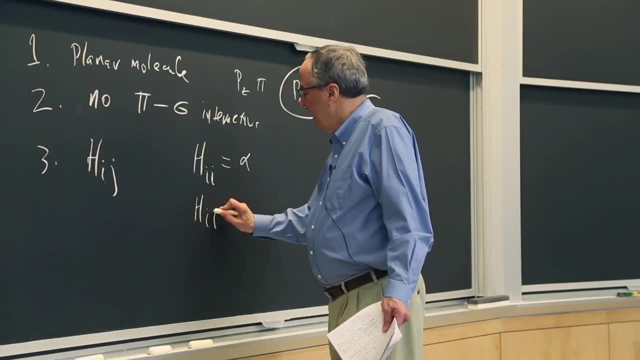 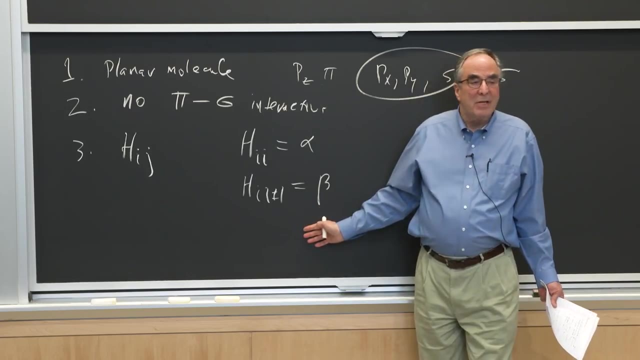 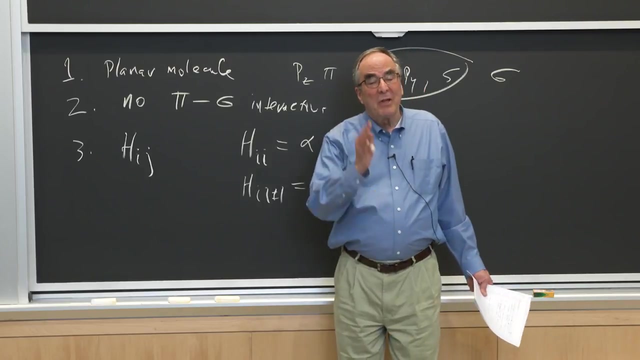 It's the same for all carbon atoms, regardless of who's nearby, And we have H-I-I plus or minus 1 adjacent atoms And it's beta. That's it. That's the whole ballgame And it's really a simple you know. 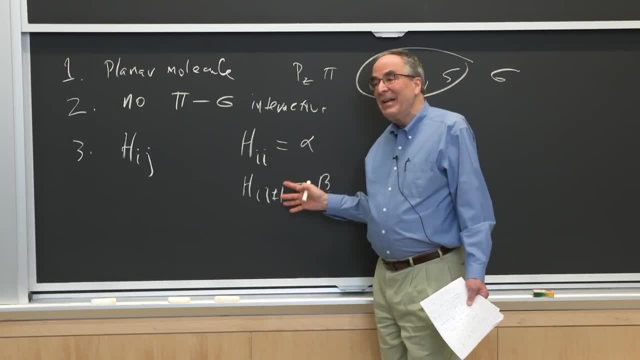 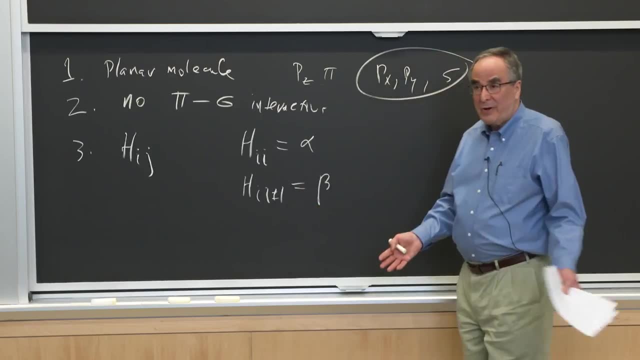 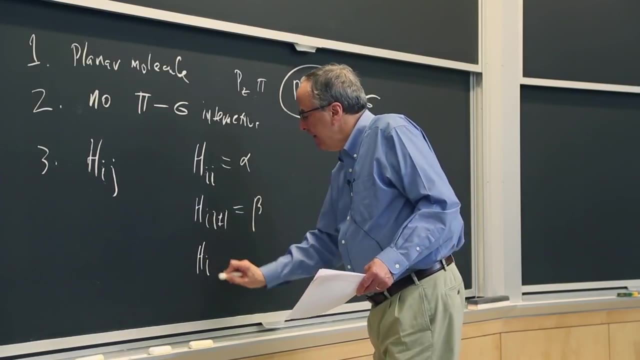 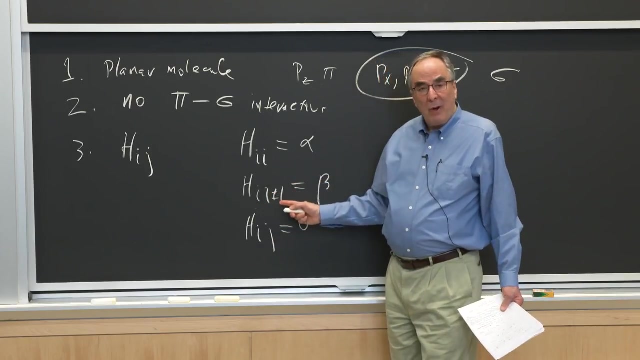 there's far less here than in LCAOMO, But it's still a toy. Both are toy models and they're both very useful. OK, And everything else OK Which is not diagonal or off-diagonal by 1, 0.. 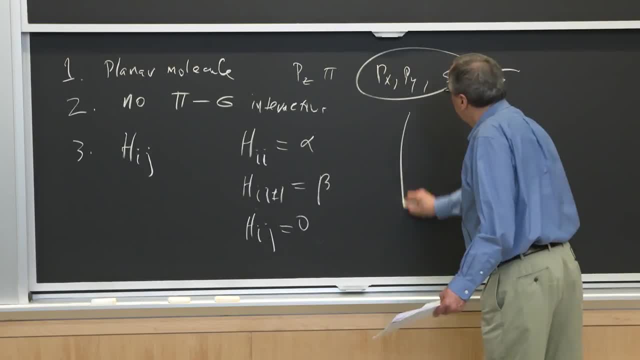 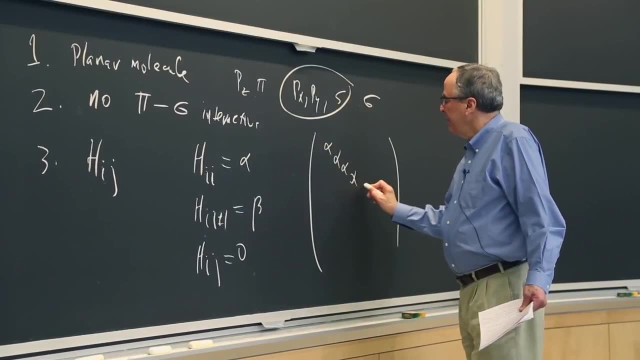 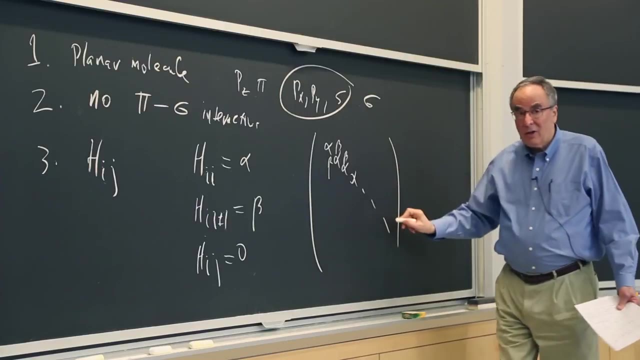 That's really convenient, And so you can draw this H matrix, regardless of what it looks like, as alpha, alpha, alpha, alpha, et cetera, along the diagonal and beta, beta, beta, et cetera, beta along the near diagonal. 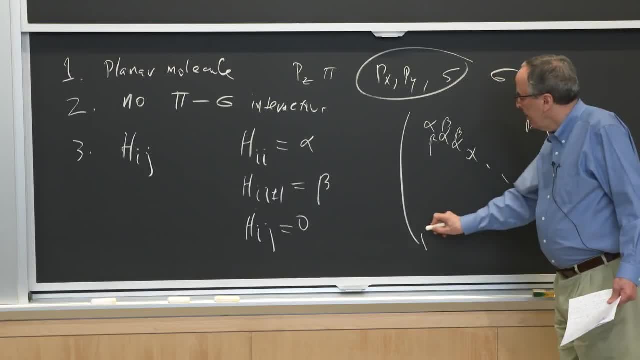 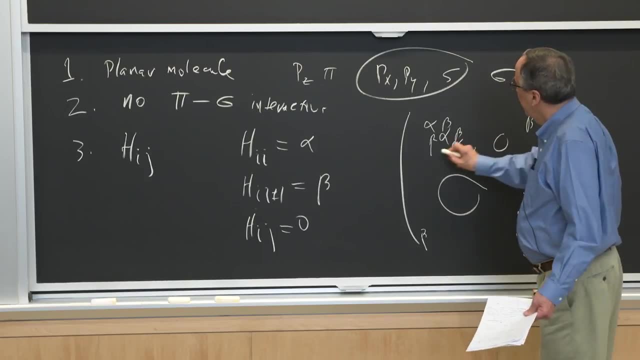 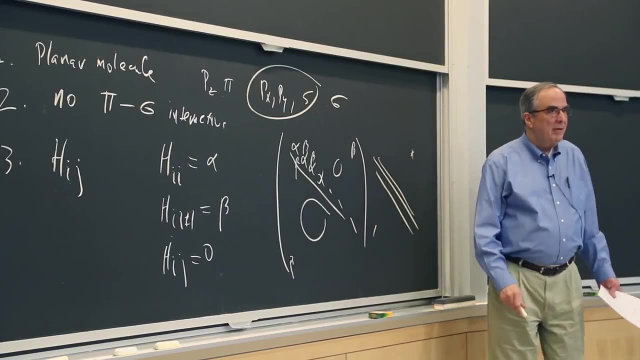 And if it's a ring, you have a beta here and here. So that's pretty simple. So we have 0s, 0s. So it has a tri-diagonal structure with something up here and there. Never forget this thing, here and there. 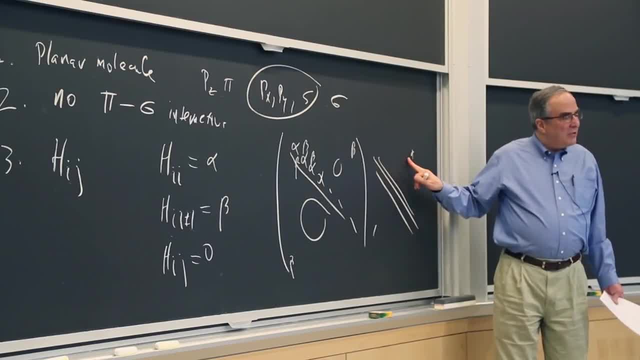 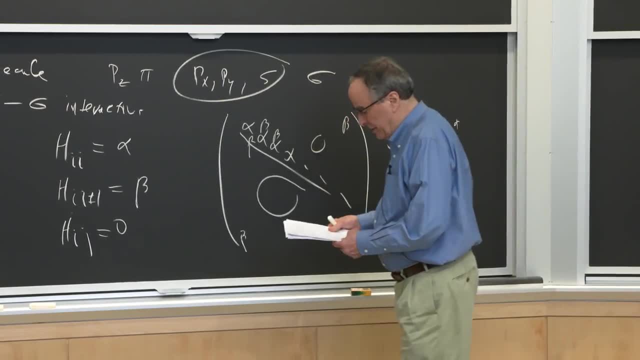 which is present when you have a ring and it's not present when you don't. That's it. That's it All. that's in the Huckel theory. It's just, It's there, OK, And so now things can be more complicated. 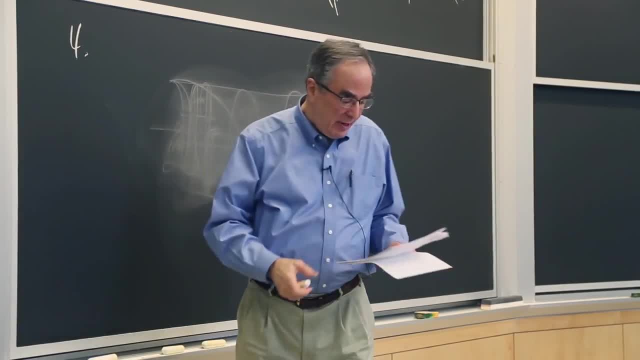 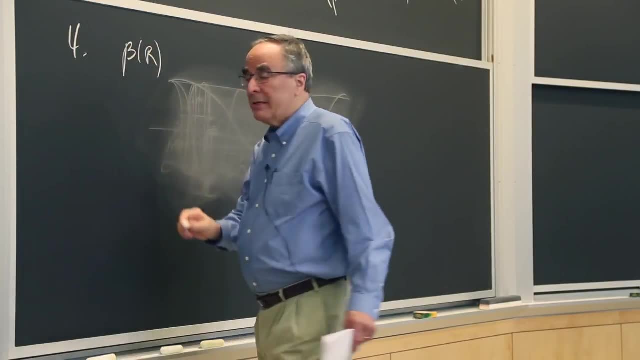 So if we're not content with what we get from the really primitive theory, we can do something like saying: well, we can make beta be dependent on inter-equilibrium distance if the molecule for some reason is constrained, trained, to have non-equal bond lengths. 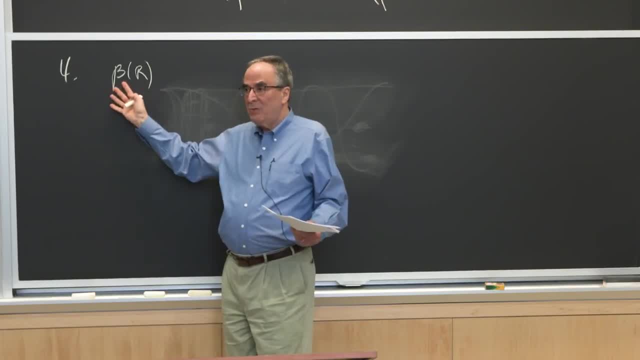 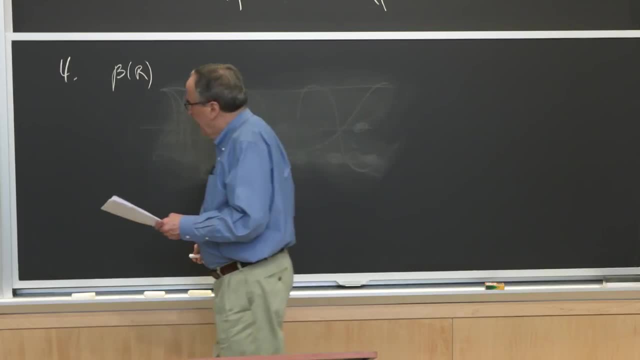 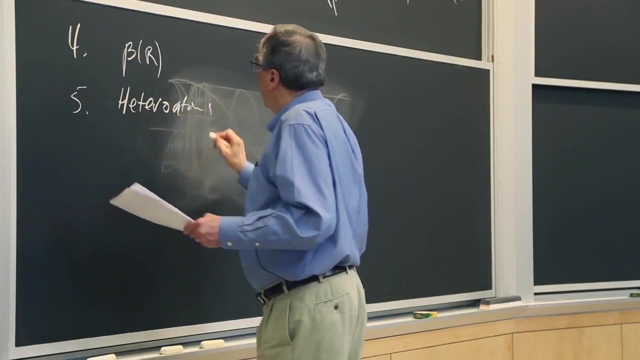 So we can add an additional parameter, some kind of reason for this beta to be dependent on R- But that's already getting sophisticated- And heteroatoms, in other words, if you have a nitrogen instead of a carbon in a benzene-type ring. 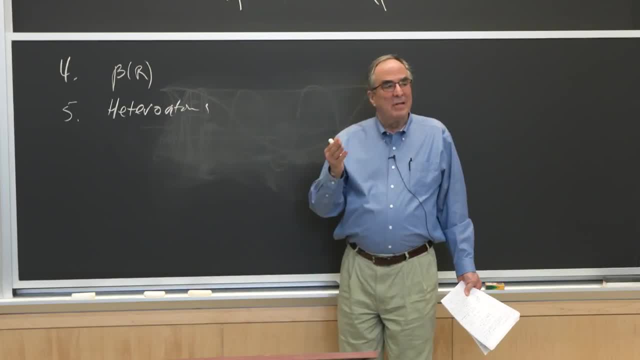 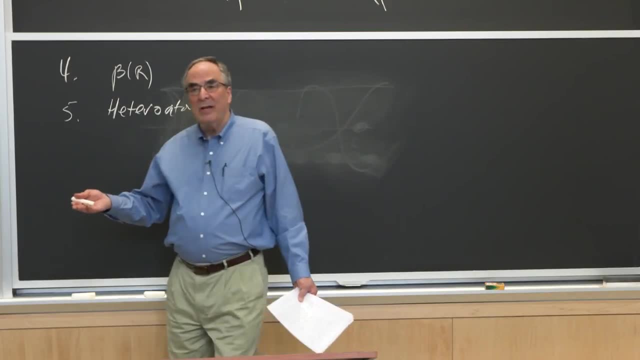 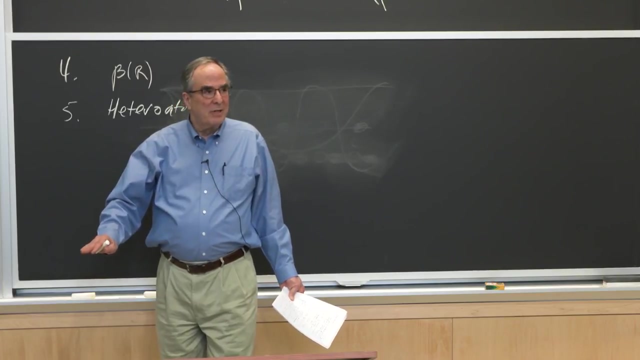 and you can have a. so well, nitrogen is different. Nitrogen is different from carbon. It has a different in LCAO theory. the distance, the ionization energy for nitrogen is different from carbon. It's larger And so the heteroatoms can be included. 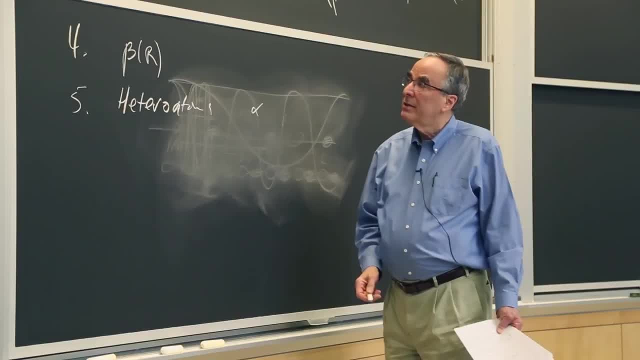 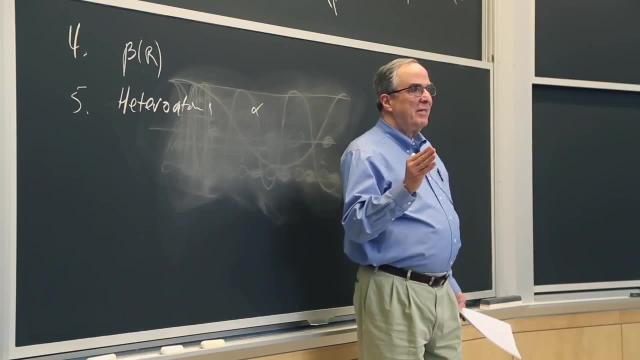 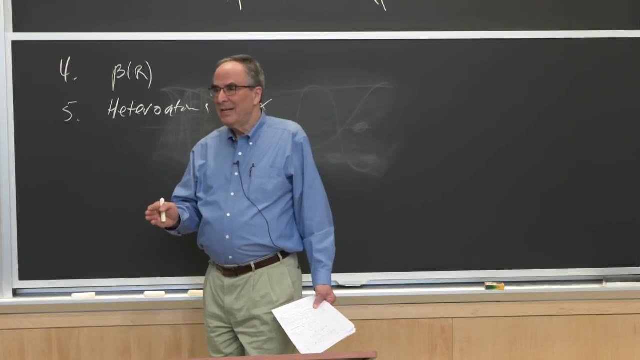 if you use a different value of alpha, And now alpha and beta are both negative. Now this is a little bit fraudulent. Yeah, Do you also have to pick a new beta for? Yes, But the main thing is alpha, I see. 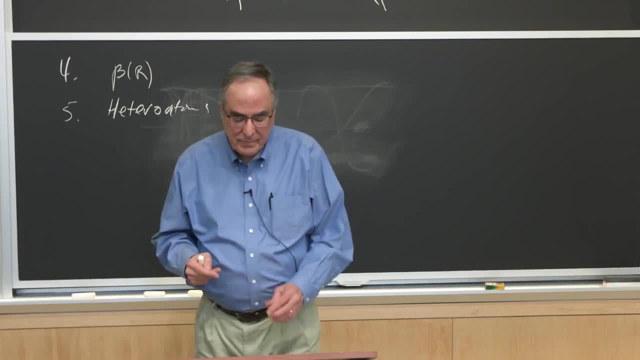 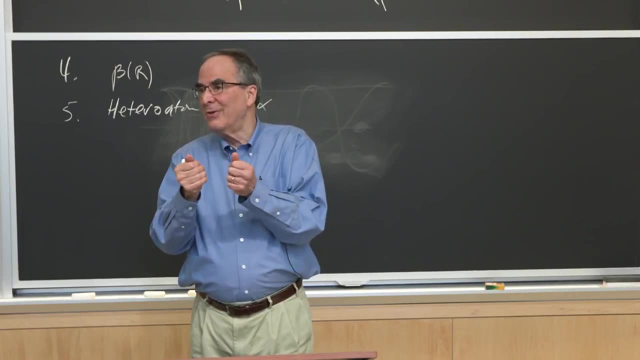 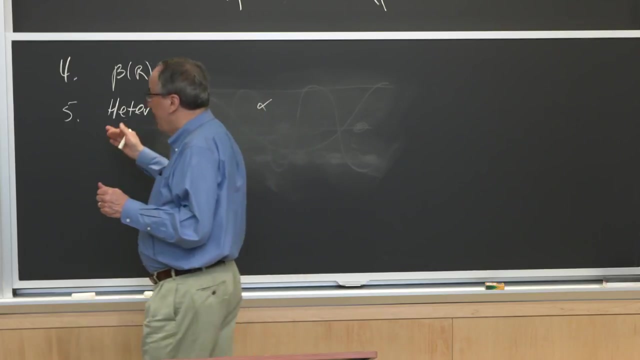 Why is that? Why is that Because the overlap between two beta, it comes from overlap, even though we're neglecting overlap, And so the bond distances between normal and heteroatoms are not usually that different. And so, but the thing is, 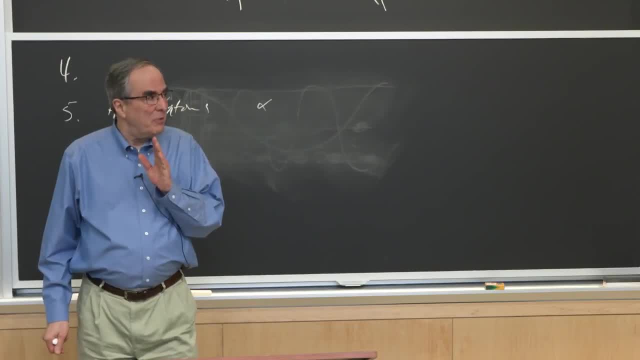 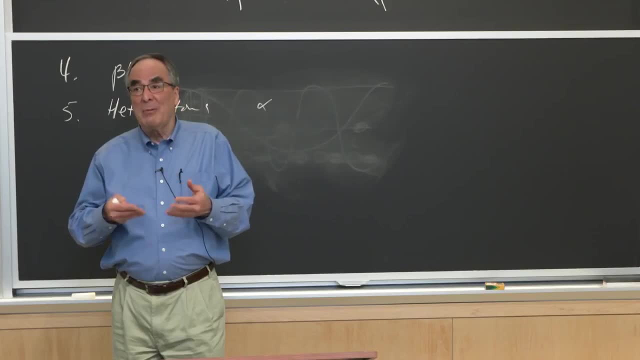 You put what you need into the model And the first thing you do is you solve the most simple model And you say this is not quite what I wanted And so I allow a couple of extra degrees of freedom, And it's really instructive how these things work. 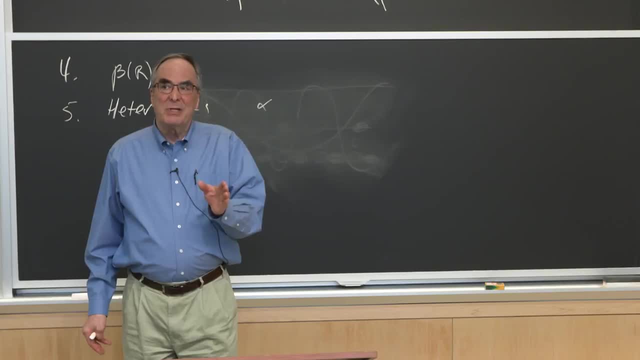 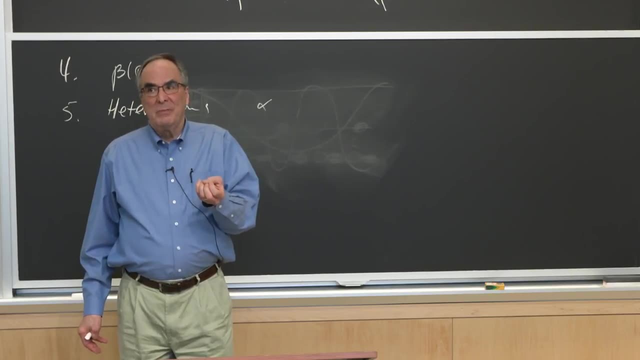 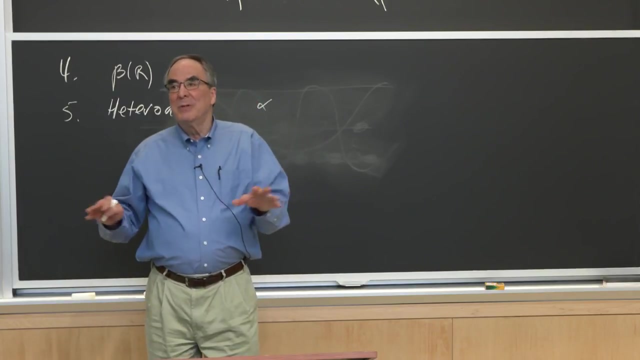 But the thing is you're not calculating the matrix element of a real operator. It's all make-believe But it's really powerful because what you're comparing is families of molecules And the reality might be really complicated, but the complexity in each member of the family, 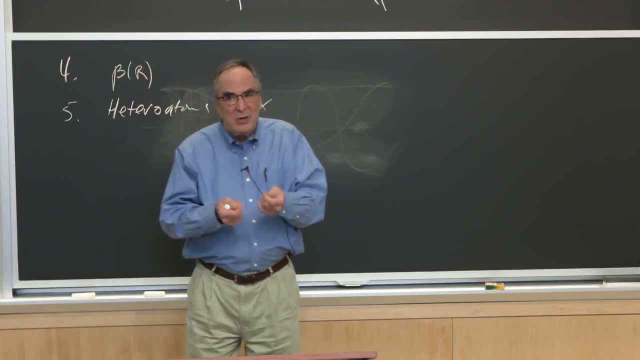 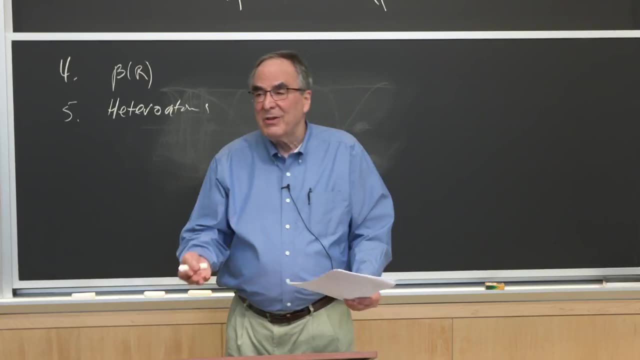 is pretty much the same, And what it's allowing you to see is: what are the differences? It allows you to see the big picture, And this is. I love this And in fact, at an early stage in my education, I thought Huckel theory was wonderful. 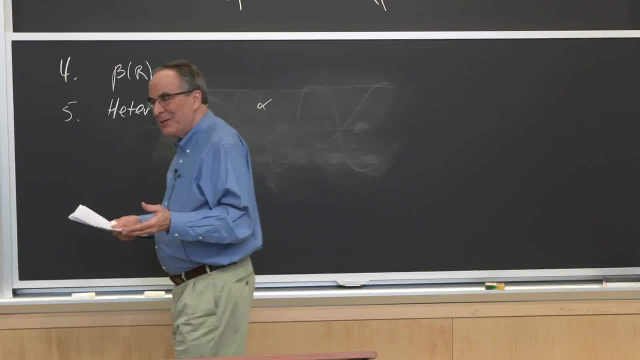 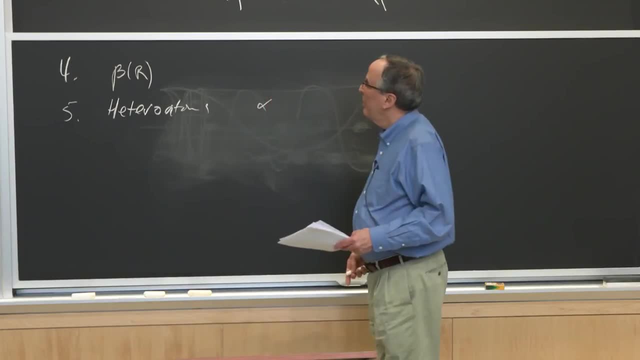 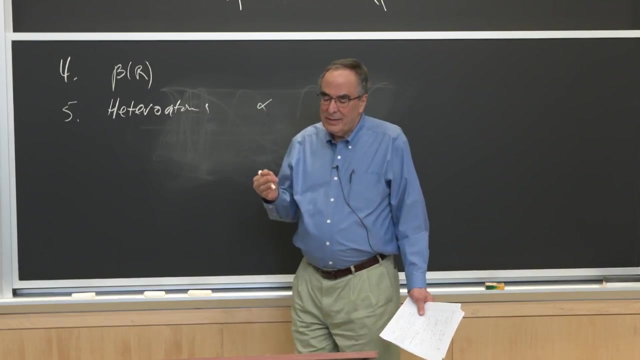 And it was sort of what got me interested in quantum mechanics, because it You normally see Huckel theory before you know anything about quantum mechanics, because it's just a game. So heteroatoms, you can fiddle with alpha, Now the ionization energies for carbon and nitrogen. 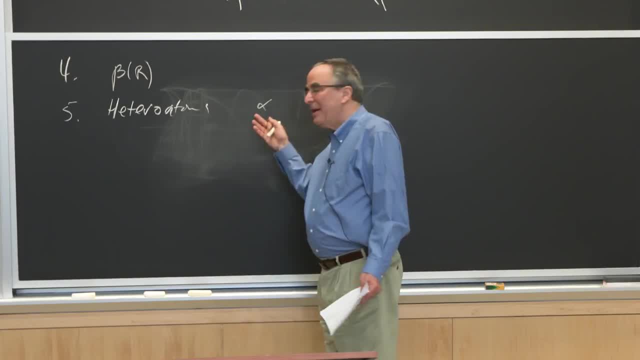 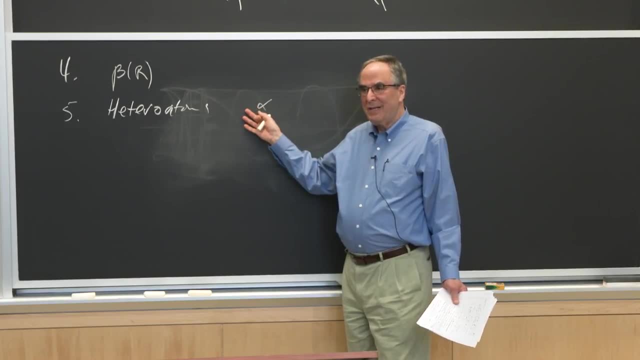 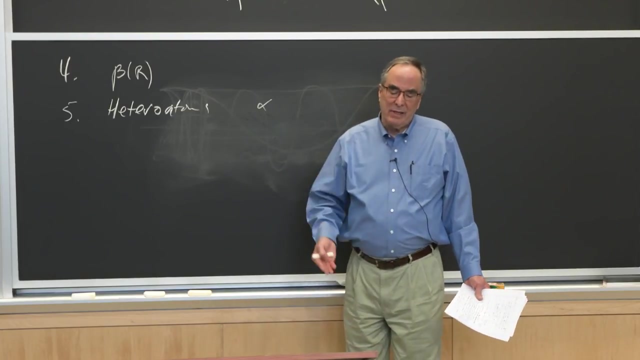 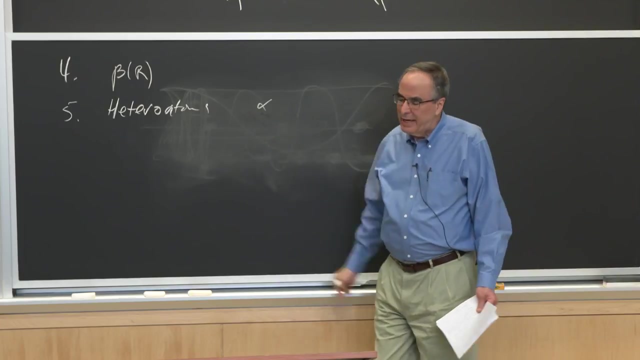 are not that different. I'm sorry, they're very different, But the effect on the alpha value in Huckel theory is very small. Well, so it is. So. the more electronegative or the higher the ionization energy, the alpha value becomes increasingly negative. 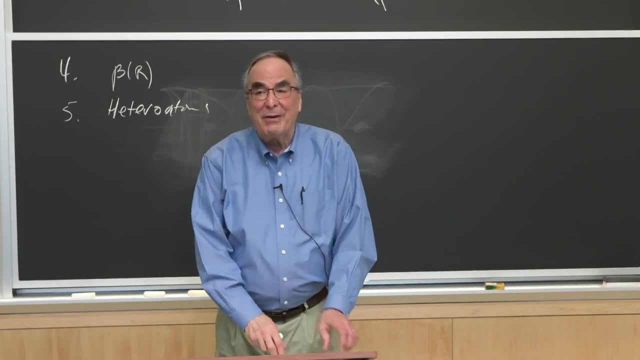 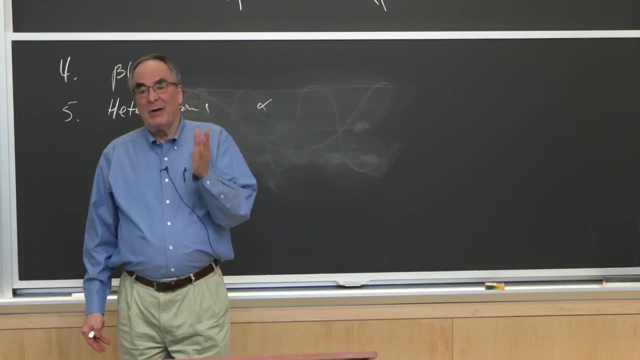 Now I was starting to say something is fraudulent and I was distracted by a really good question. Alpha is on the diagonal And we know we can determine the sign of a diagonal Diagonal element, And we know we can't determine the sign. 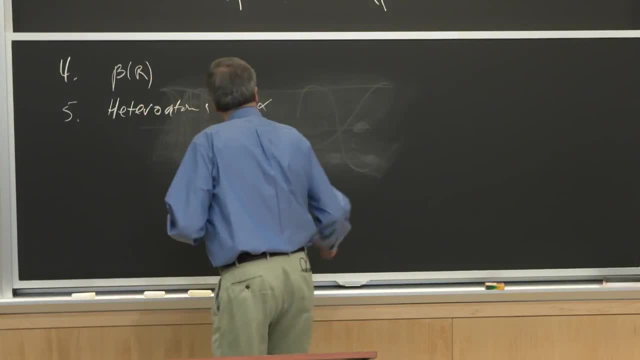 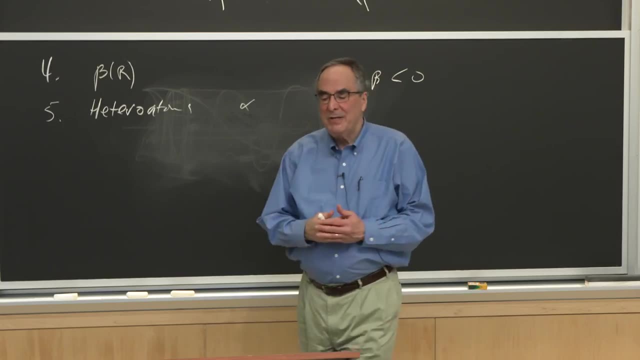 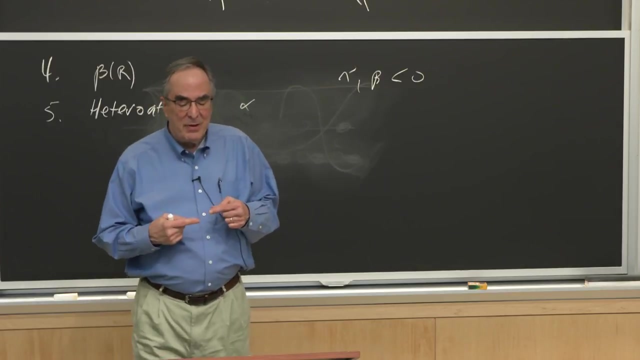 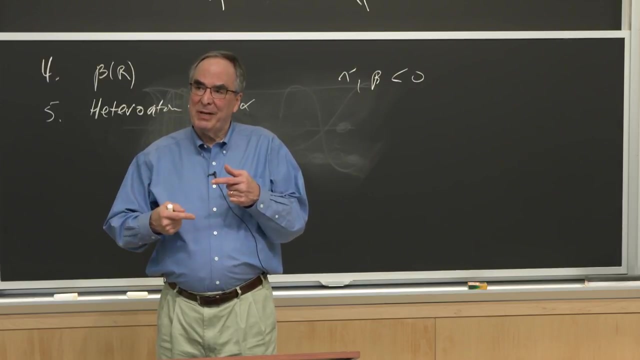 of an off-diagonal element, But we say that alpha and beta are both less than 0. And the reason for this is that when you solve the secular equation especially, you get two eigenvalues: one where you have minus beta and one where you have plus beta. 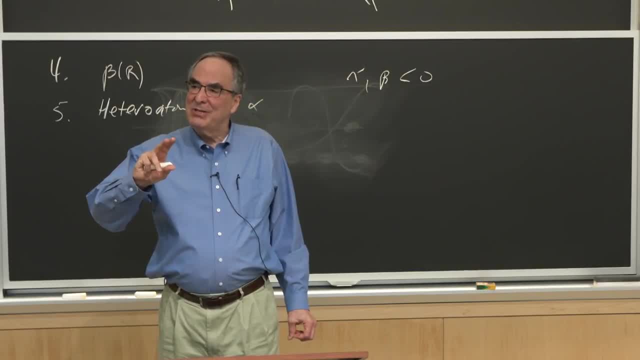 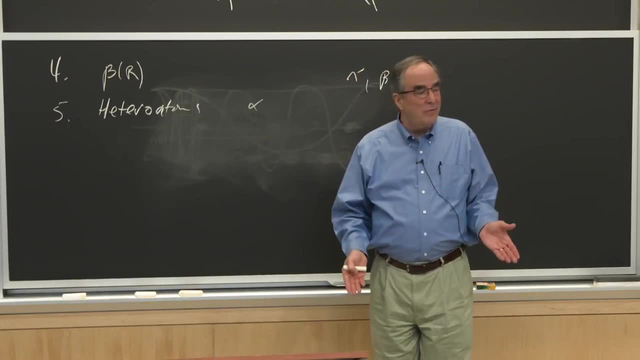 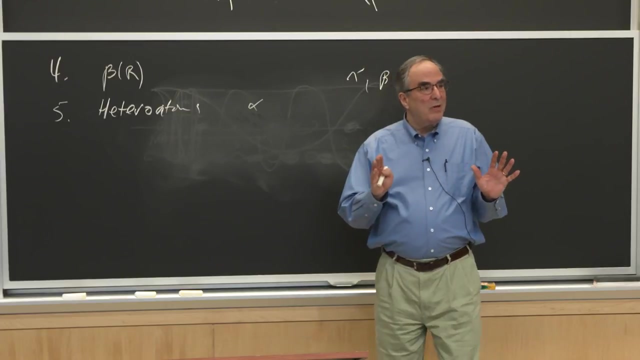 And so, in a sense, beta is present, but it's just a sign choice, And since alpha and beta have to do with stability, we just say alpha is negative, We know that, And beta is chosen to be always negative. You could have had beta be positive. 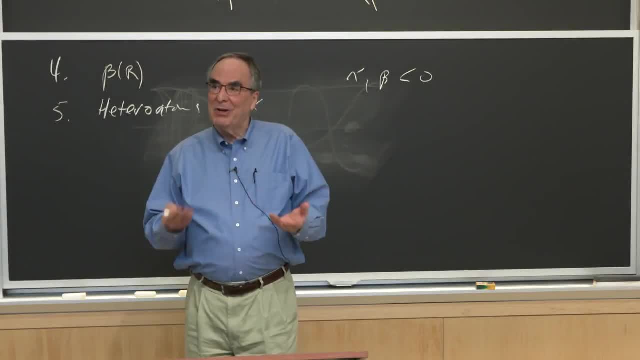 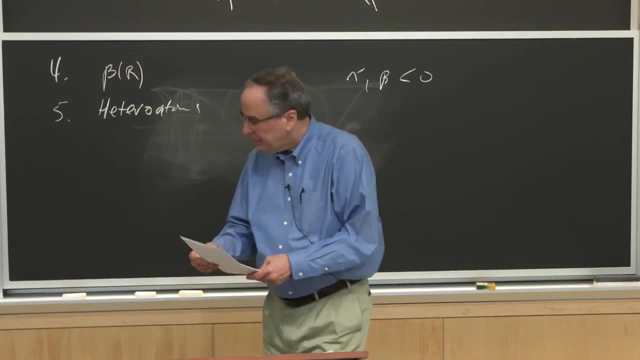 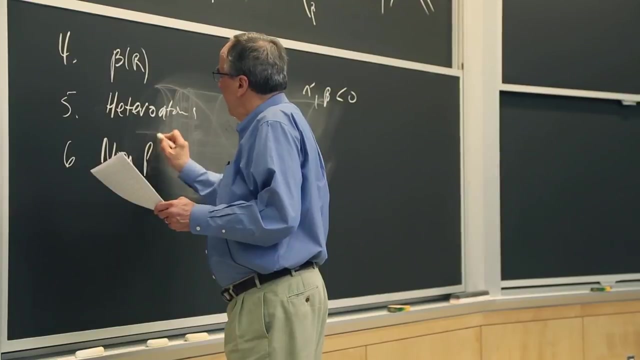 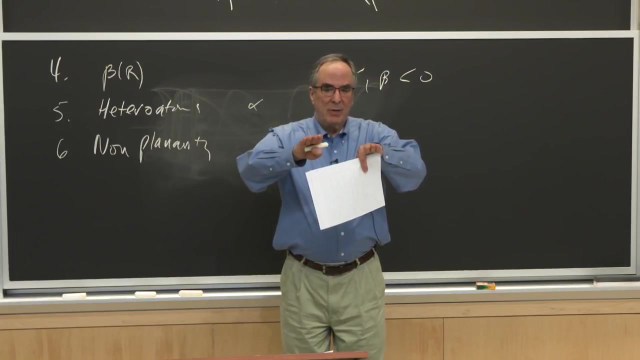 and you could do all the theory. It's just a lot more complicated explaining all the cases, All right, So let's continue with this. And so we can do heteroatoms. We can So if we have a non-planar system, 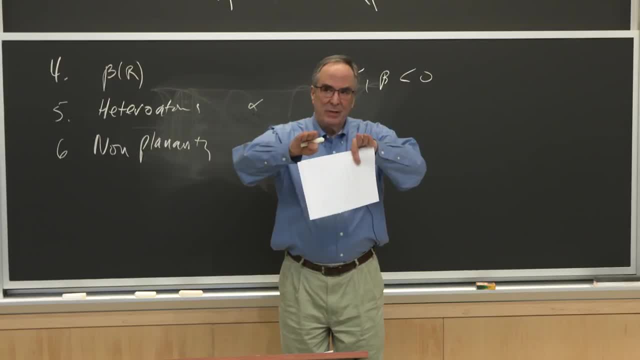 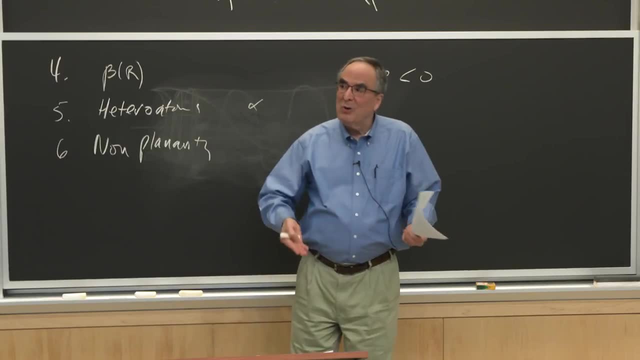 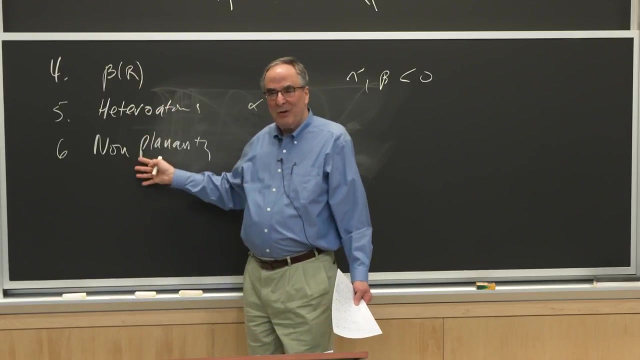 we can say that beta is a function of the dihedral angle. We can put that in, We can do anything we want. We have a molecule and we're trying to describe it, Describe its properties relative to the normal members of the group, which are planar and no heteroatoms. 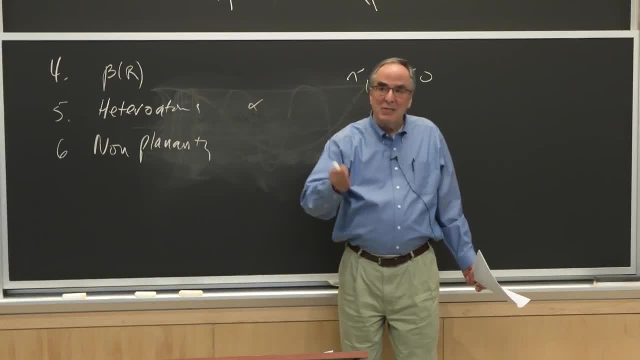 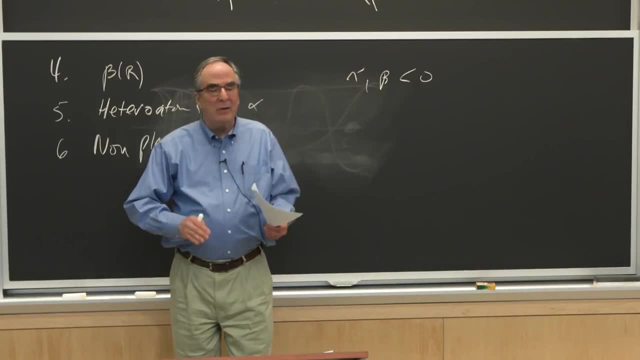 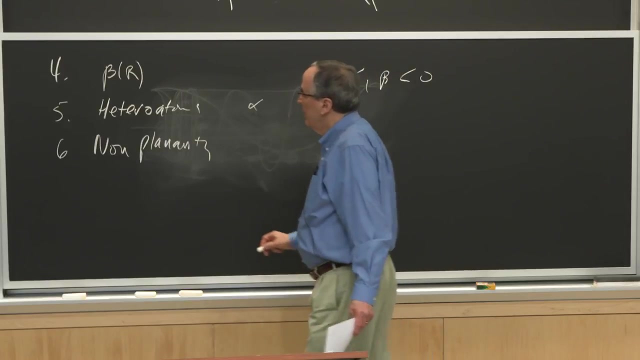 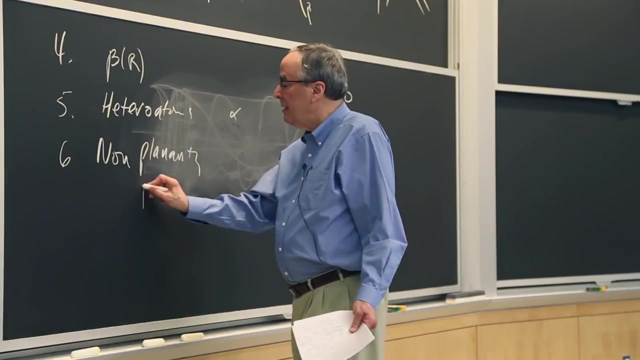 And we can do stuff that will accommodate these interesting differences, which you can impose by putting the molecule in a constrained environment or doing stuff that distorts the geometry. So we do this and we can also count. So when we do this, We get a Hamiltonian and we get the energies of the orbitals. 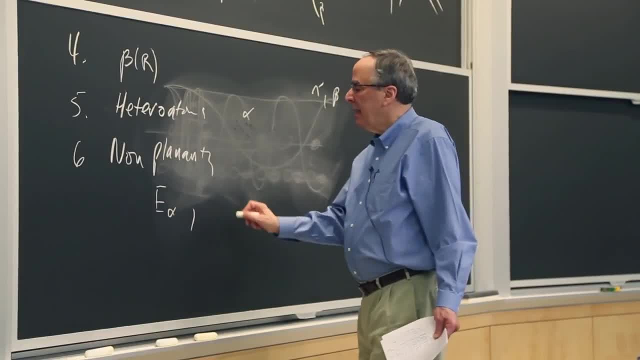 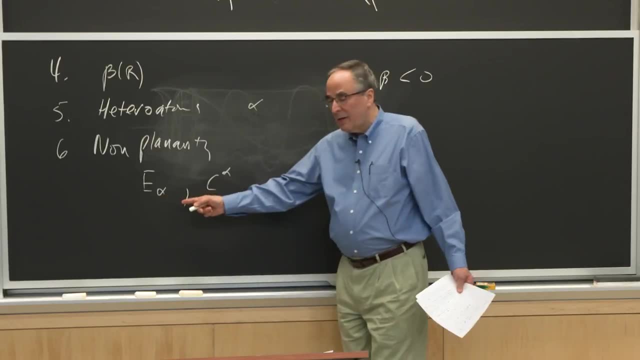 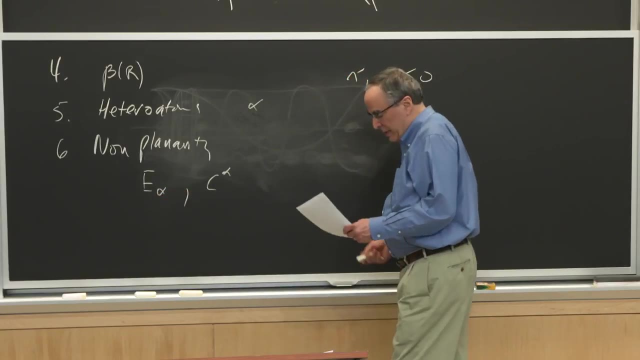 And we get the eigenvectors. the eigenvector that corresponds to each energy And the total energy involves the sum over the energies of each of the occupied orbitals, the number of electrons in that, And we can also get bond order. 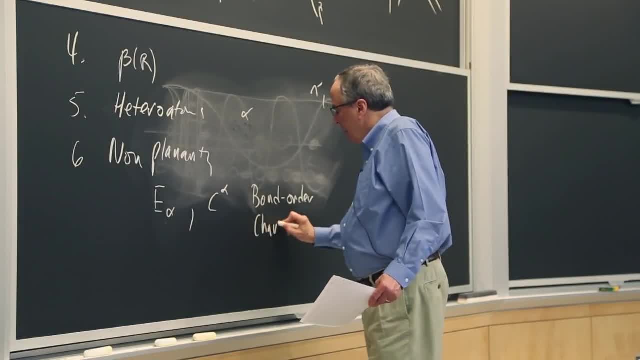 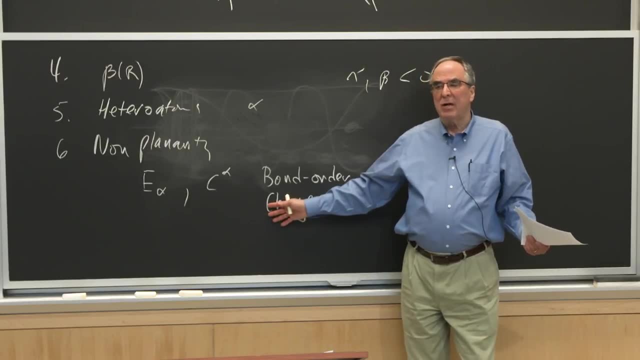 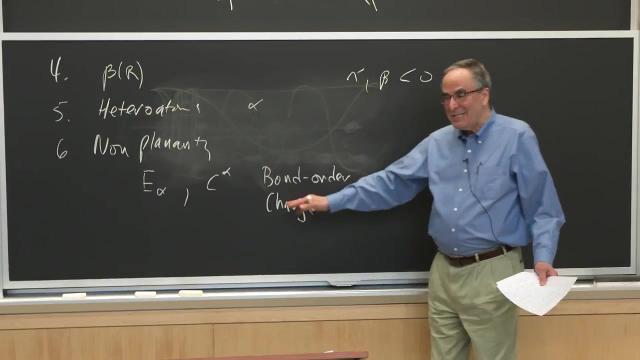 And charge. So sometimes we want to know what is the charge on each atom, If the charge is going to be different from 0. Because that also controls chemistry. Certain things are negatively charged atoms or are sought out by certain classes of reactants. 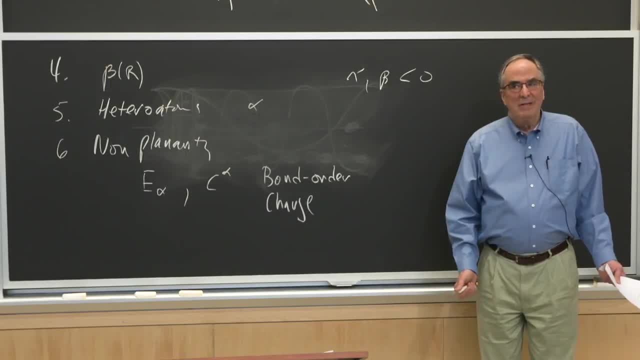 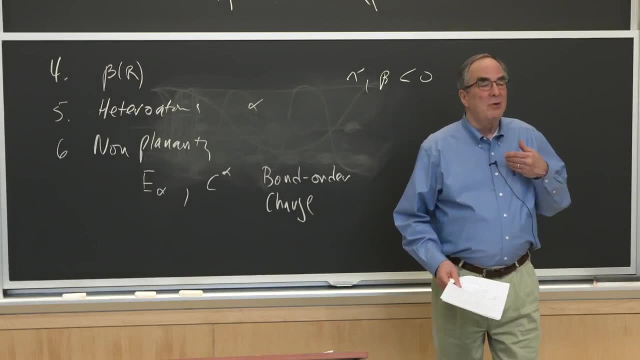 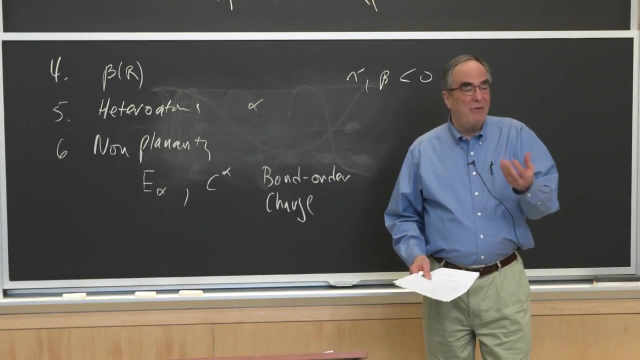 Anyway. so you get all this stuff And of course, some of it will require a little bit of patchwork, But once you do this for your career and you discover that there are certain things that I know how to handle and I use my favorite parameters, 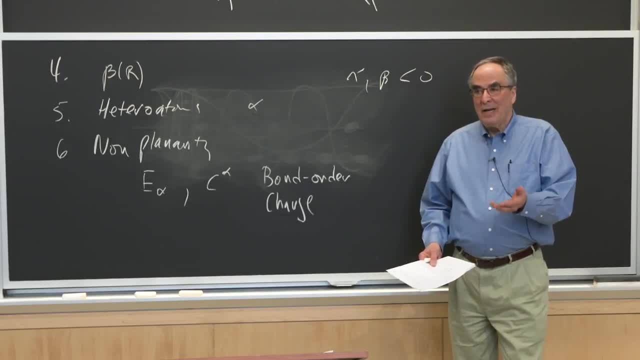 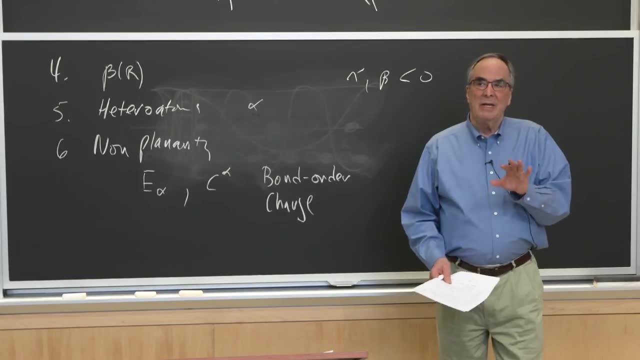 for it and you get closer to the truth. And you always want to be surprised, Because when the crude theory cannot be made consistent with observations, you know you didn't. You didn't, You did something special. You have a molecule which has a property which is unexpected. 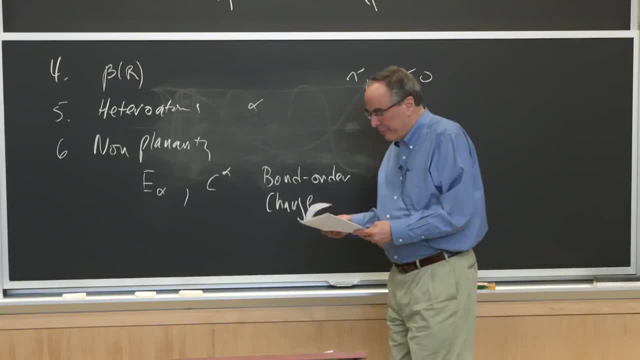 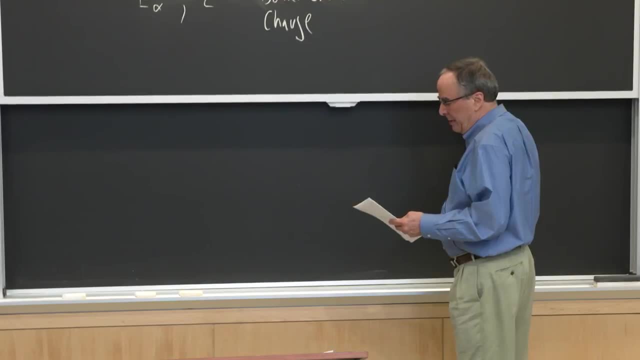 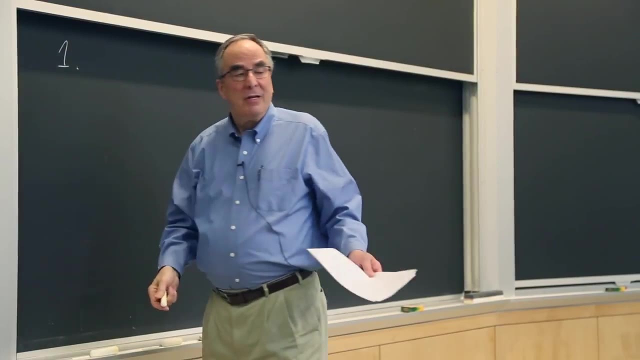 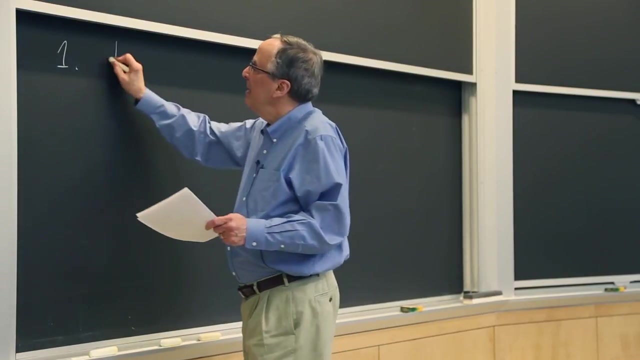 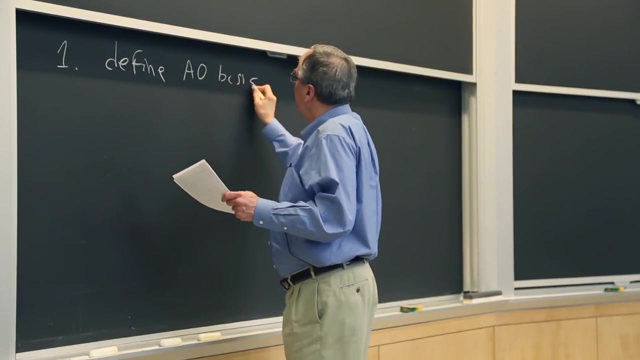 And we like that. So when you're doing quantum chemistry, there are five steps. Or when you're doing molecular orbital theory- And this is one of Troy's rules- We have a five step procedure And we define the atomic orbital basis set. 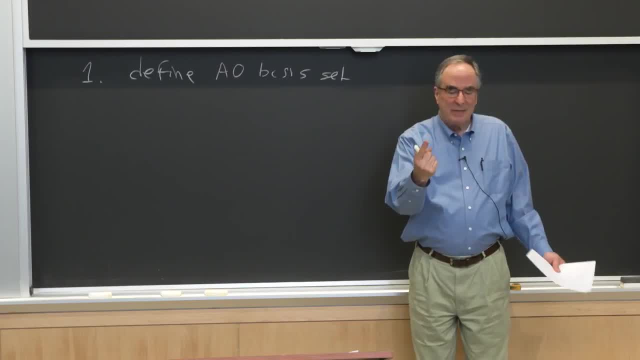 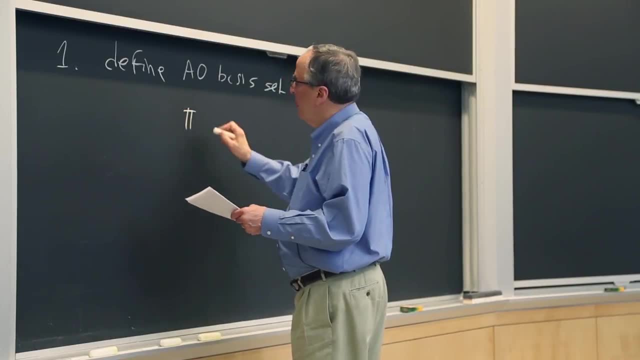 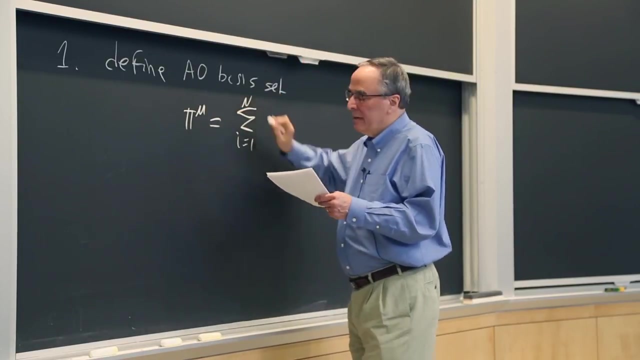 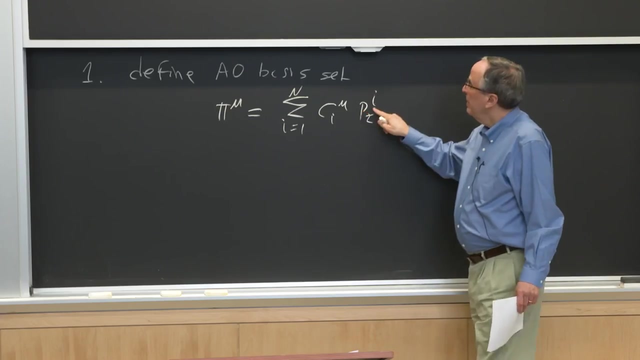 And the basis set is one pz orbital per atom, And so we can have a molecular orbital which is the sum i equals 1 to n. That was ci, mu, pzi. So this is the pz orbital on the i-th atom, This is the coefficient for it, for this particular linear. 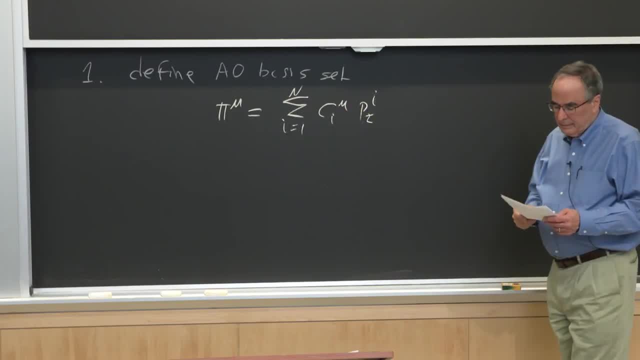 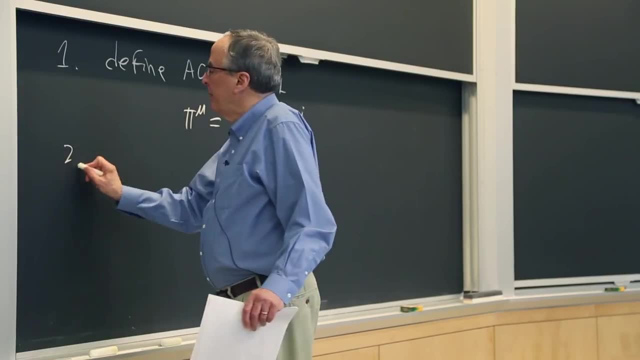 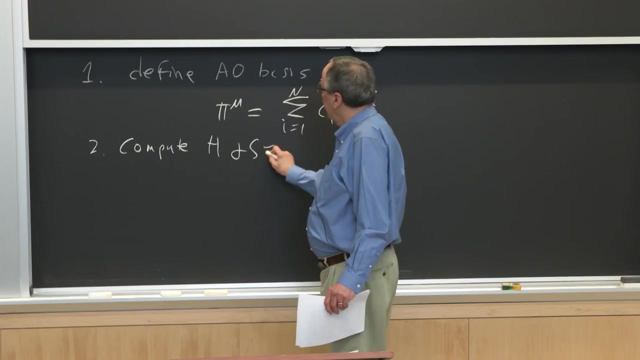 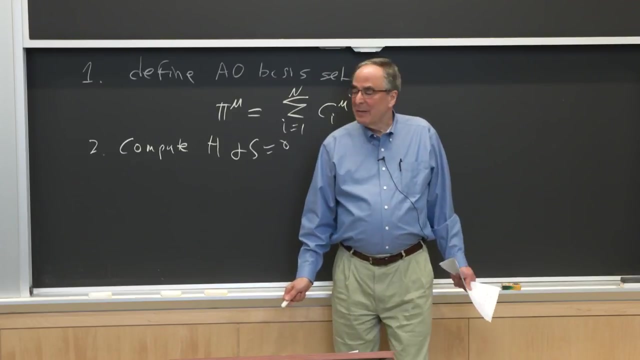 combination. OK, So we have a bunch of molecular orbitals. Next step: compute H and S. But S is 0.. OK, Because we made this ridiculous assumption. It's convenient. This is called the complete neglect of overlap, And we can do that. 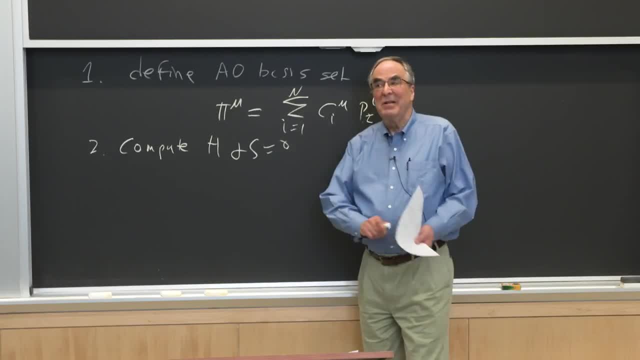 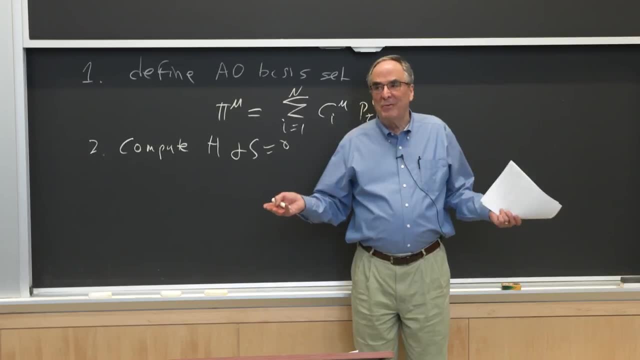 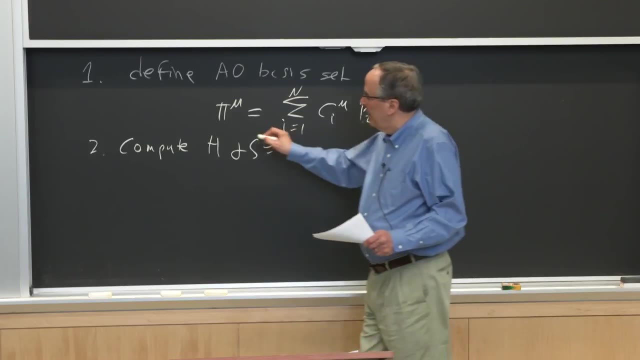 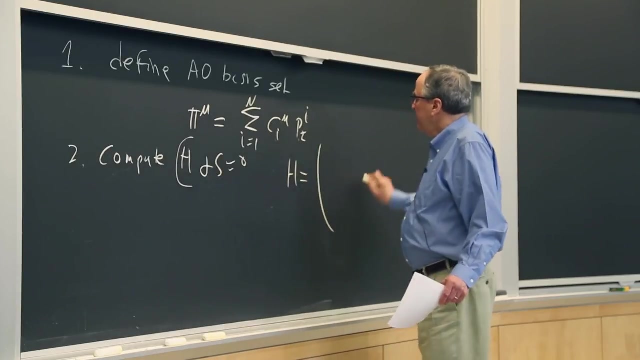 It's wrong, But when you include overlap, it leads to greater complexity of the calculation and not much improvement in the results, And so we normally don't worry about the overlap. OK, So all we care about is this, And, as I said, H has this structure of alpha beta. 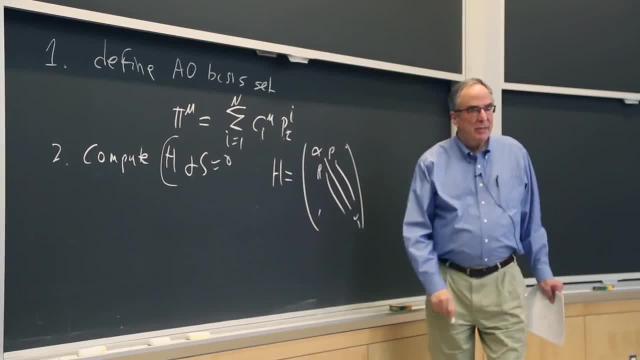 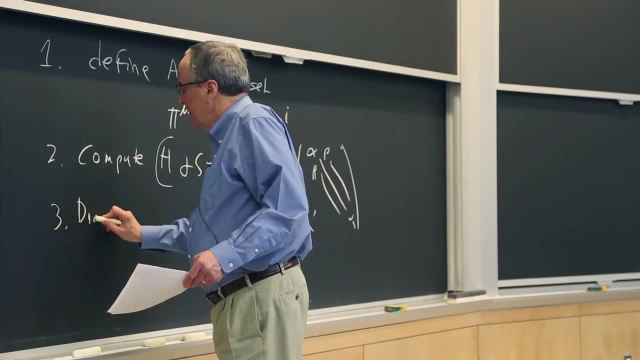 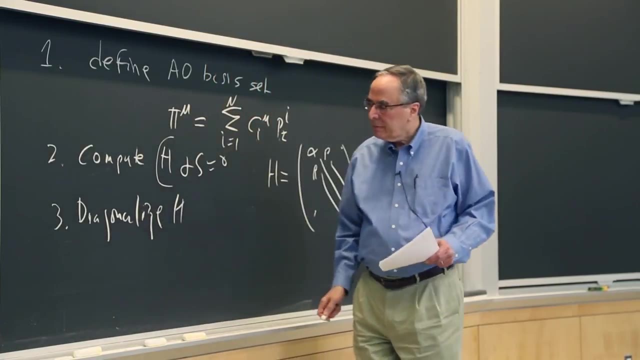 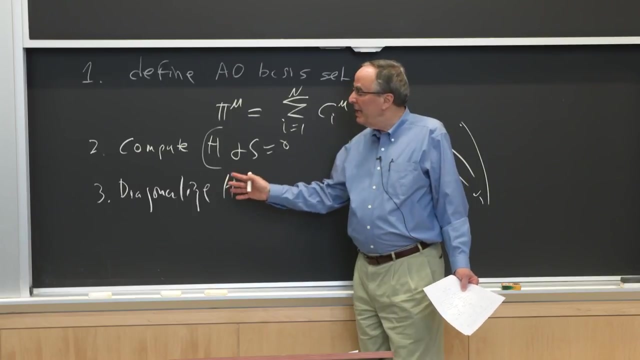 beta tridiagonal structure and maybe something up here. That's it. Then we diagonalize the Hamiltonian, And so this gives us the eigenvectors or eigenvalues, the energies and eigenvectors associated with each energy, each orbital energy. 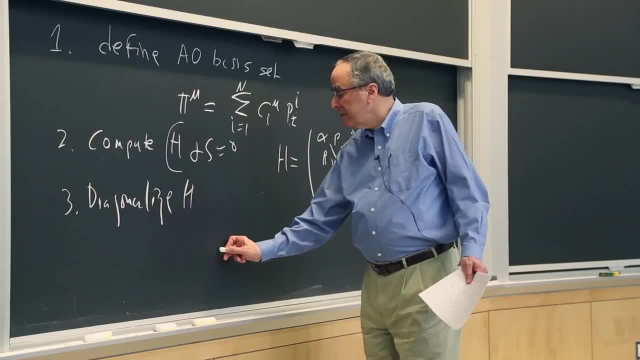 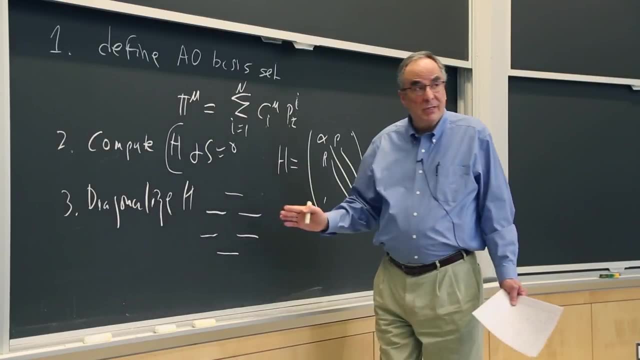 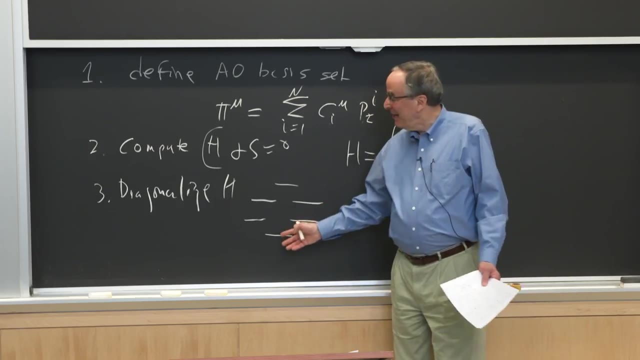 So we fill electrons into the orbitals. Now for benzene. what you would get now- this is important- How many carbon atoms in benzene Right, And how many orbitals will you get from six primitive orbitals Right? 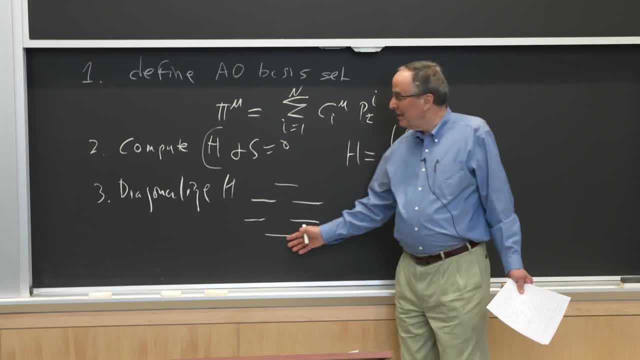 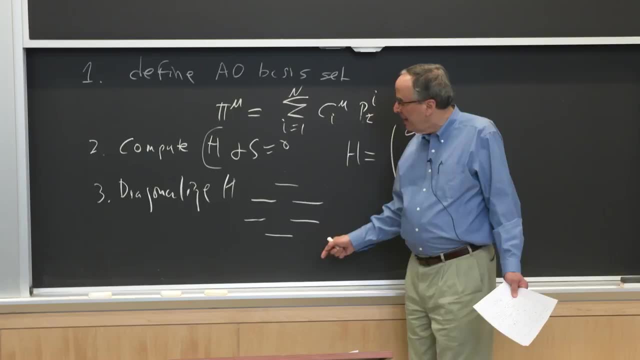 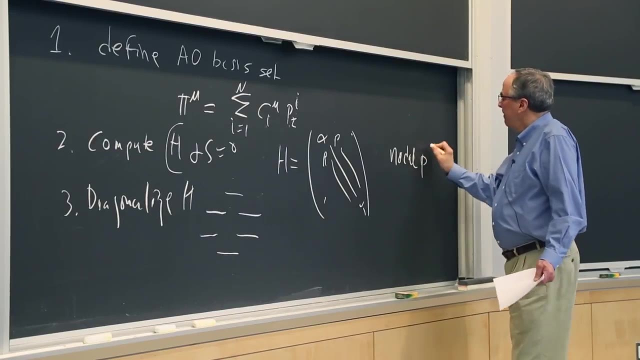 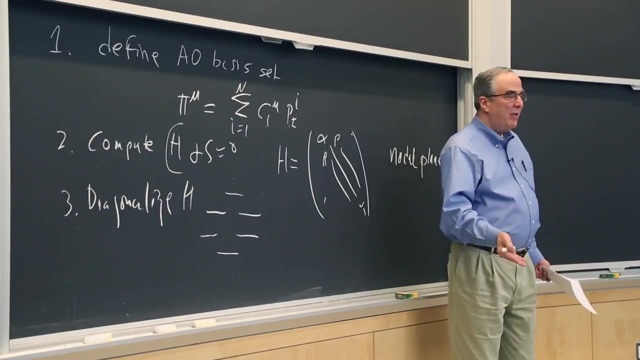 And so there are six energy levels. And it happens that when you solve the secular equation, you get this pattern And you. this is a problem where the number of nodal planes determines the order of energy. And so if you have benzene, you can. 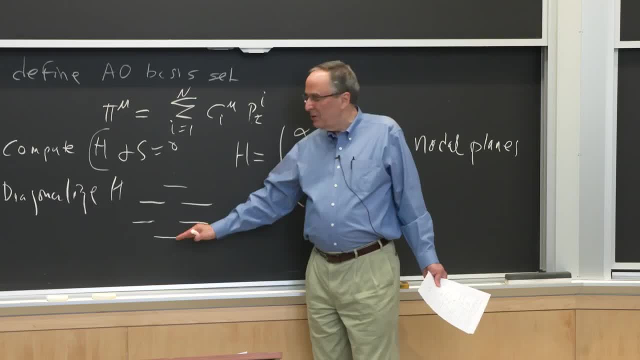 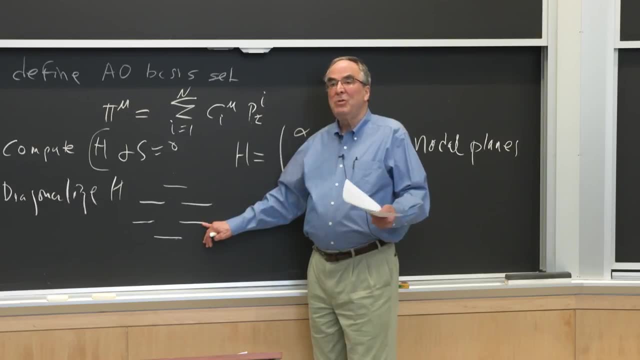 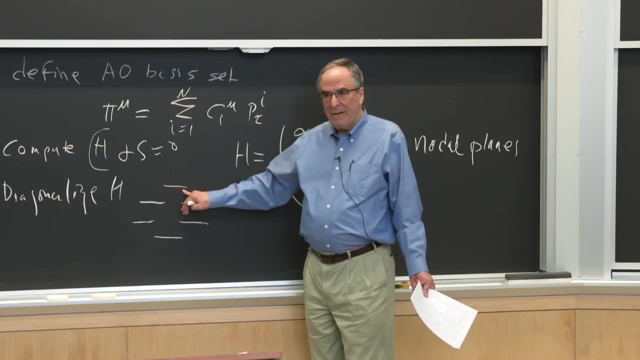 imagine that the orbitals that you can have will be no nodes, nodal planes: one nodal plane And you can have the nodal planes between the atoms or through atoms, and two nodal planes or three. You can't have any more with six atoms. 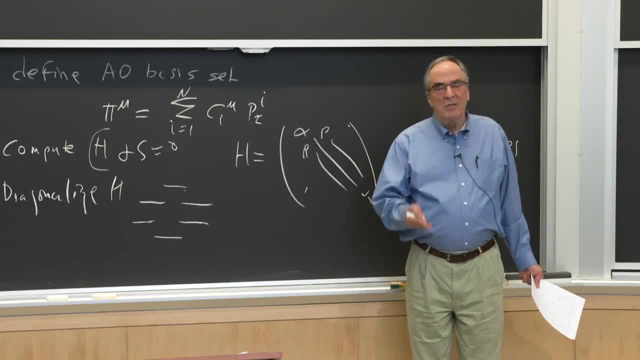 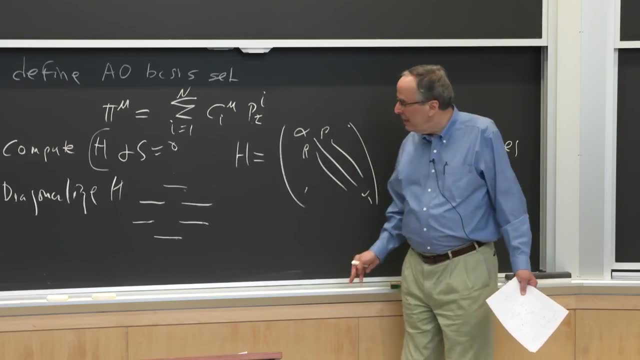 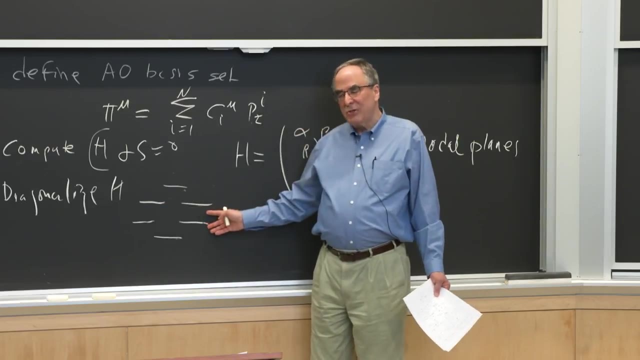 And so you almost don't have to solve this secular equation at all. You can anticipate what the structure is going to be just by saying no nodes, one node, two node, three node, And you can even anticipate double degeneracies, Right. 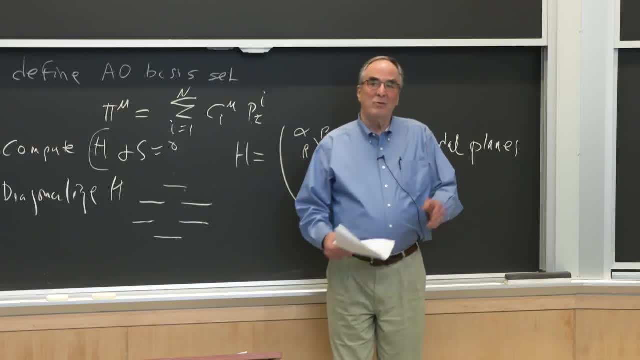 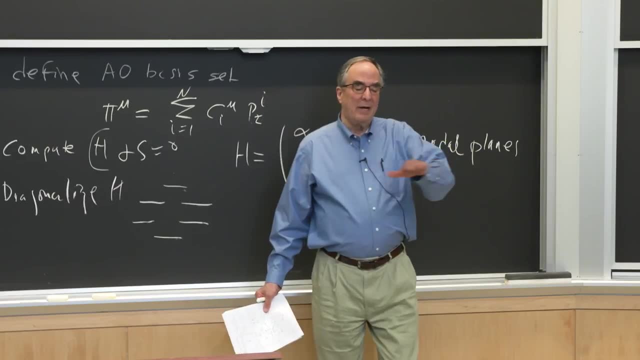 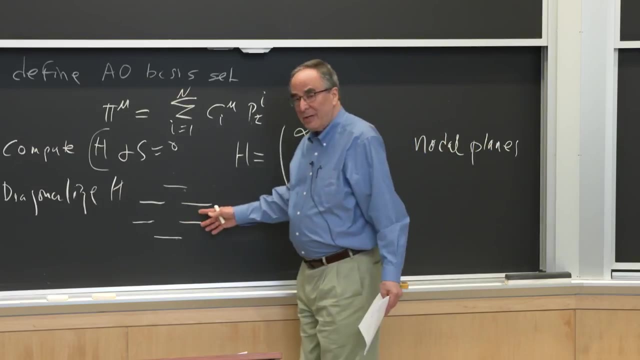 Right, Right, Because if you have two nodal planes, you can put them between through opposite bonds or through opposite atoms, And those are examples of the forms that you would deal with. The only thing you can't do is to know. 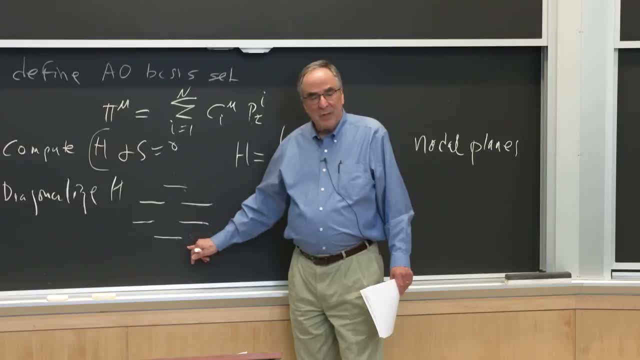 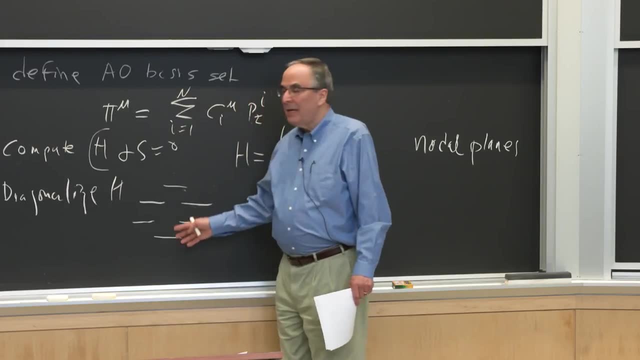 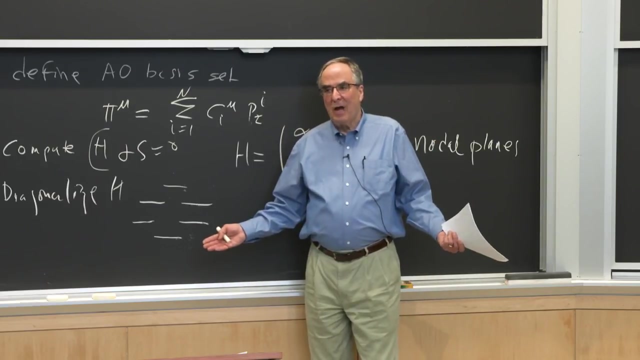 what the order the energies are. But there are tricks for that too. The tricks for that include: some of the eigenvalues is equal to the sum of the diagonal elements, And so we know that the six orbital energies will sum to zero, will sum to six alpha. 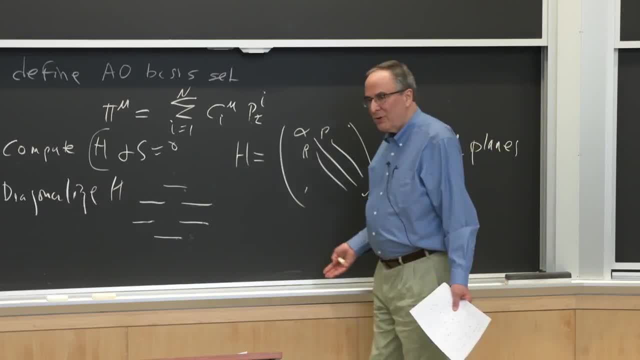 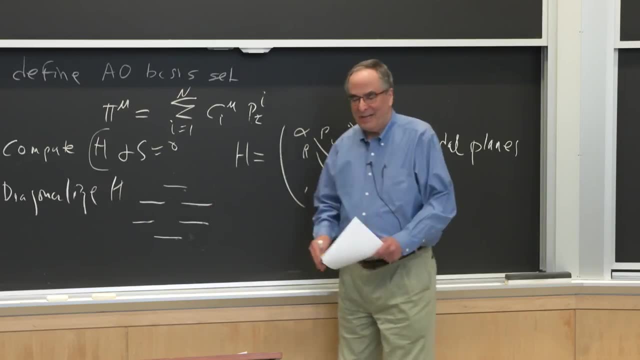 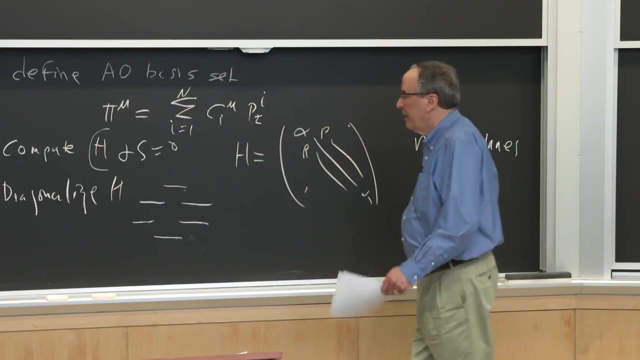 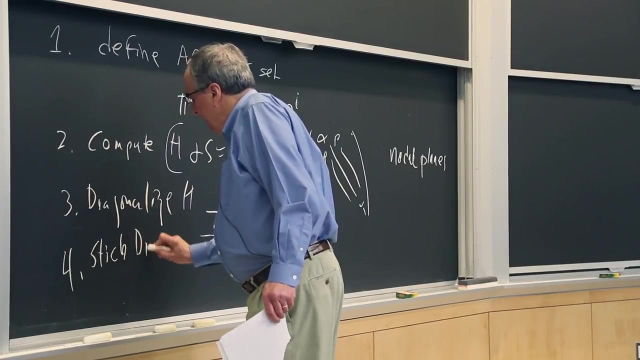 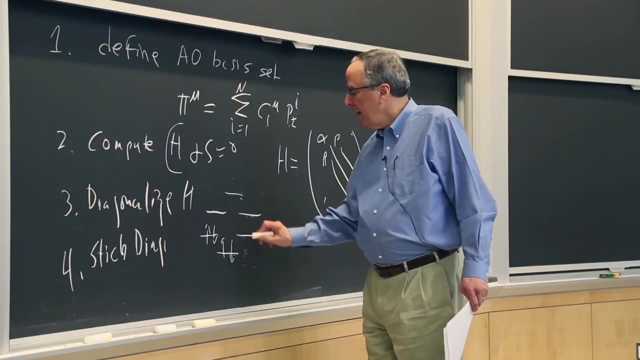 The betas go away, And there are other tricks that you can do, But generally you solve the equation. You don't want to push your requirements for symmetry too far, So we end up doing that And then stick diagrams. We fill electrons into orbitals in energy order. 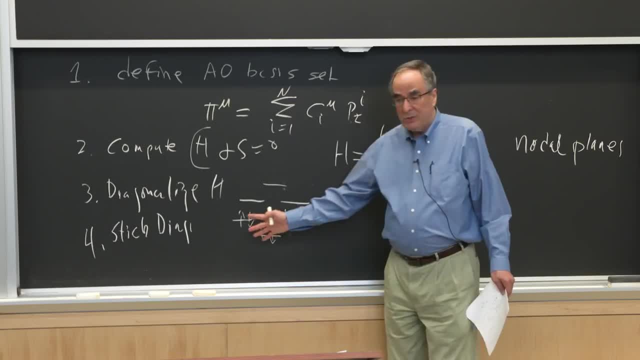 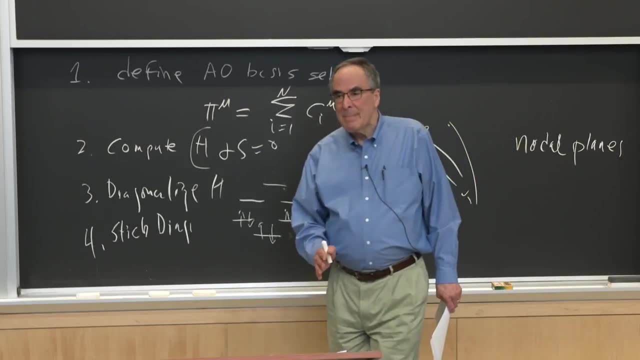 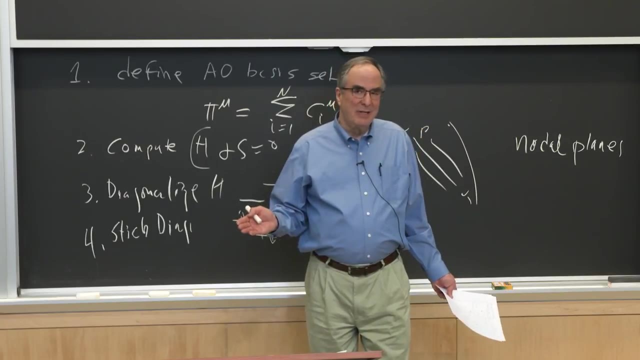 And for benzene there are six of them, And so this is then the solution. OK, The lowest energy state of benzene. This is called the independent electron approximation. They don't know about each other. This is illegal, But it's legal in the sense, if you. 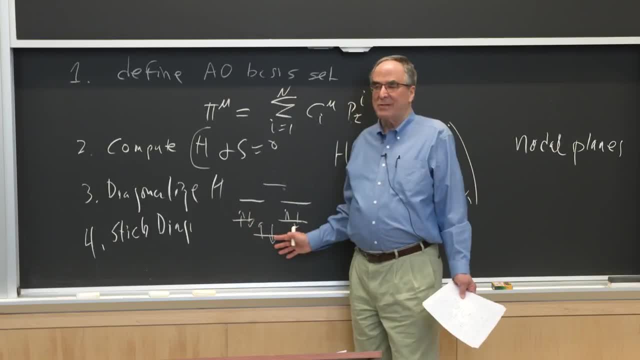 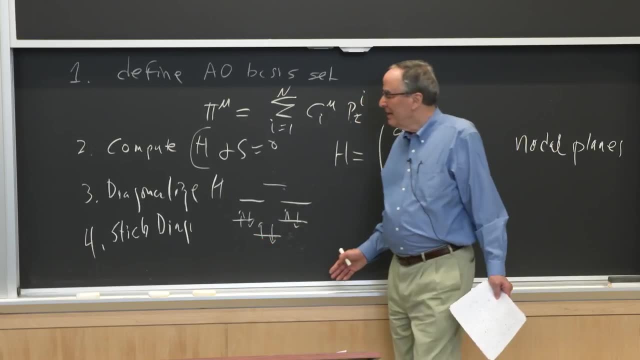 have two electrons in every orbital, they're all. you have nothing but singlet states. The ground state is always going to be a singlet state, unless you have something really weird going on, like in O2.. But that's not Huckel theory. 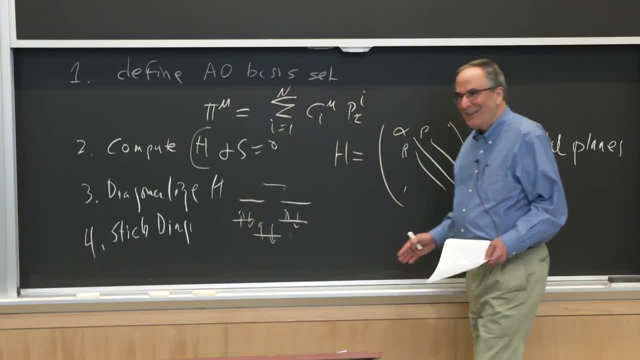 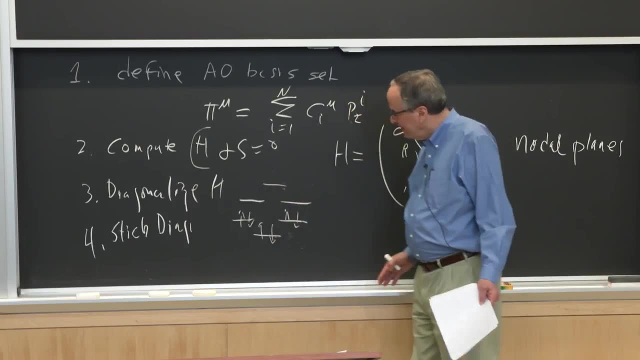 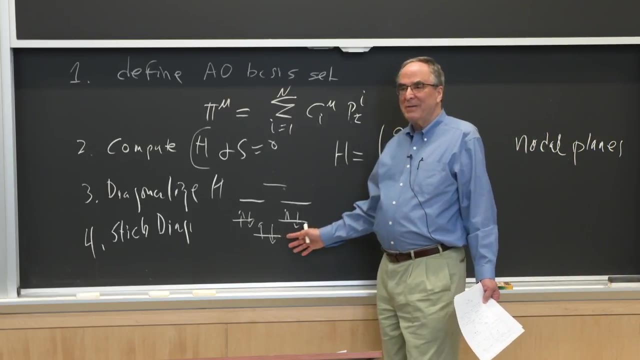 But it's examinable. Why does oxygen have a triplet ground state? That's something that every textbook says. you've got to know that. Of course, they don't really tell you anything more except something to memorize. So generally you have two electrons in each orbital. 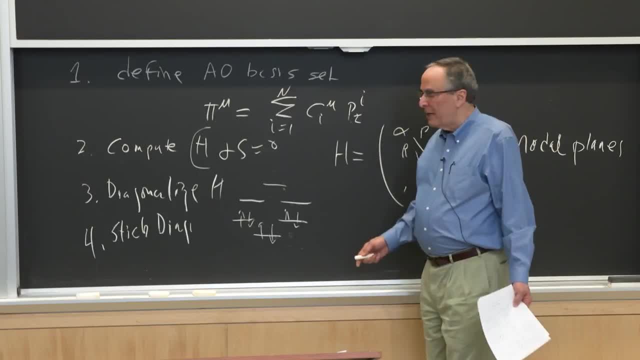 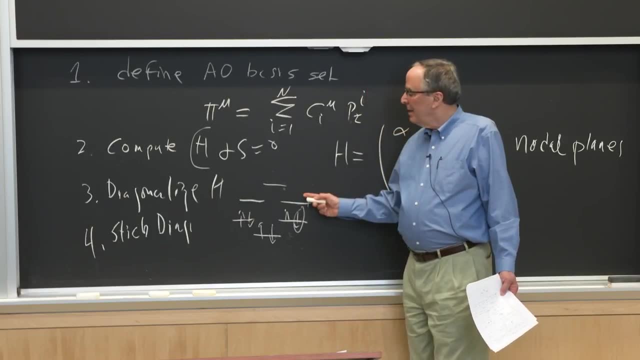 It's singlets. Now, if you're going to do spectroscopy, you're going to do this. If you're doing spectroscopy, you would perhaps promote one of these guys to a higher state, And so you'll have singlets and triplets. 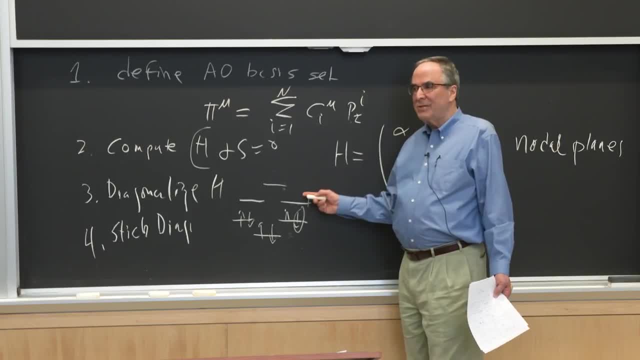 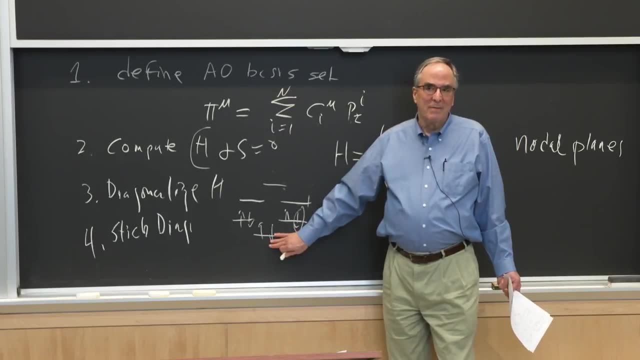 But of course the only transition you would see would be a singlet-to-singlet transition. So you might as well forget about triplets, And you might as well forget about having to anti-symmetrize. You can get away with murder, especially in Huckel theory. 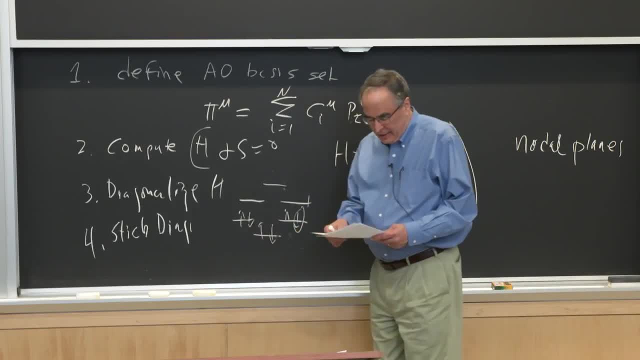 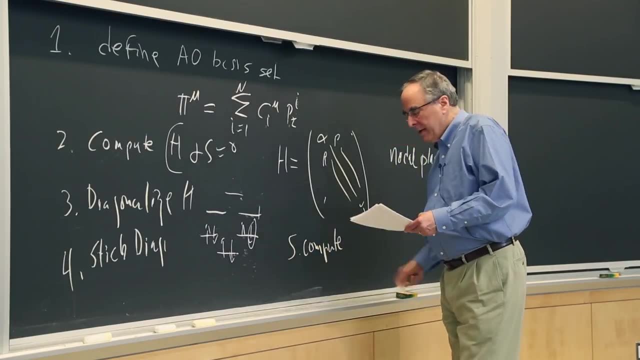 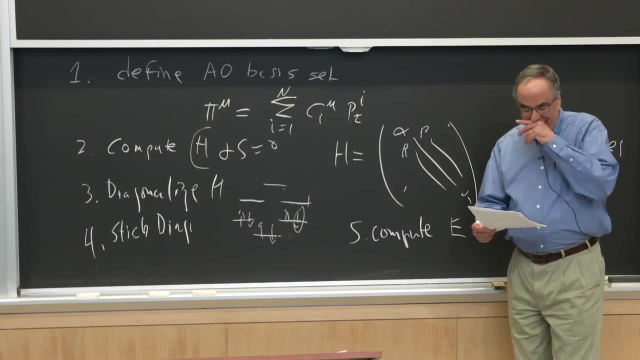 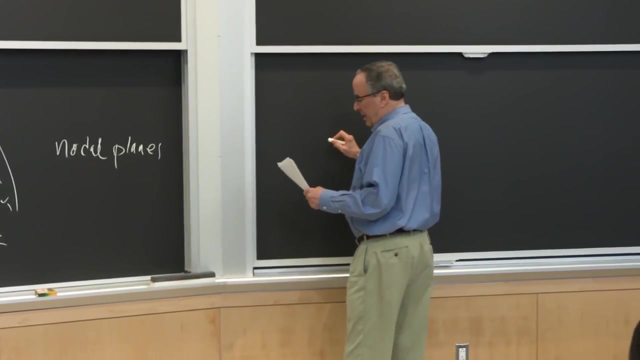 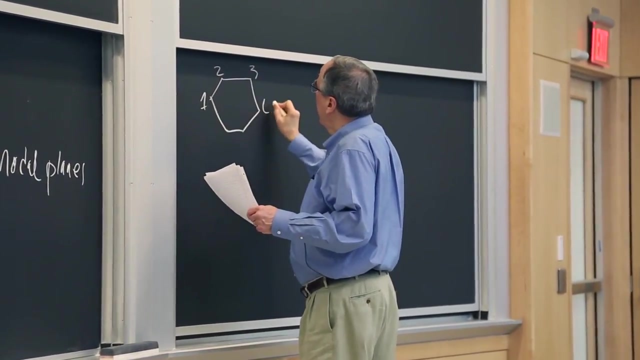 So we have a stick, We have a stick diagram, We fill electrons into the thing And then we compute the energy of the many electron problem. And so let's just do this, And you've all seen this. So we number the atoms. 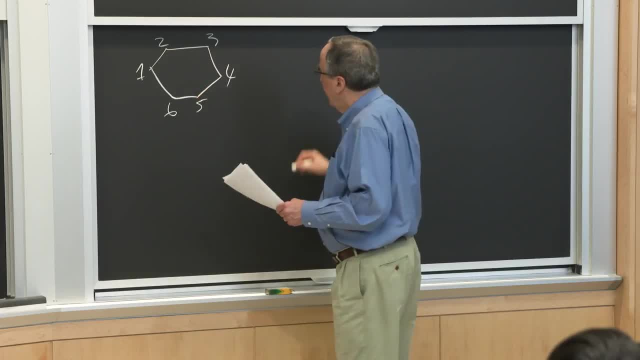 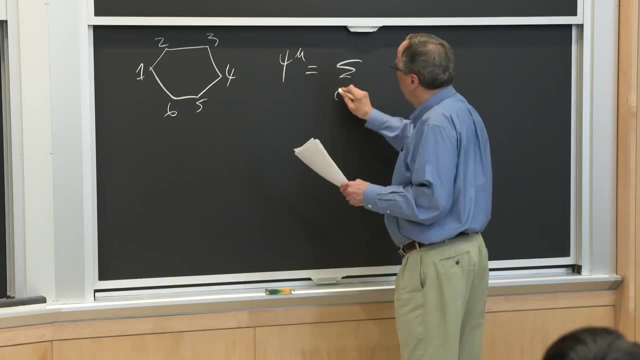 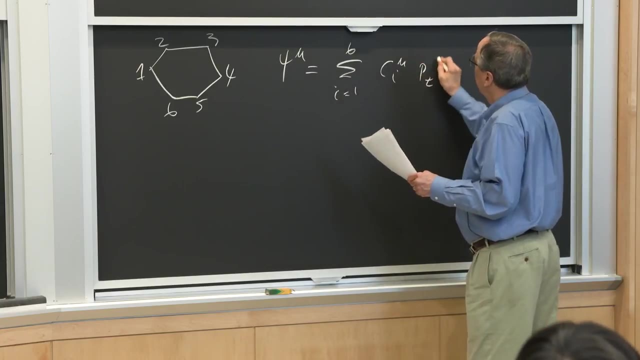 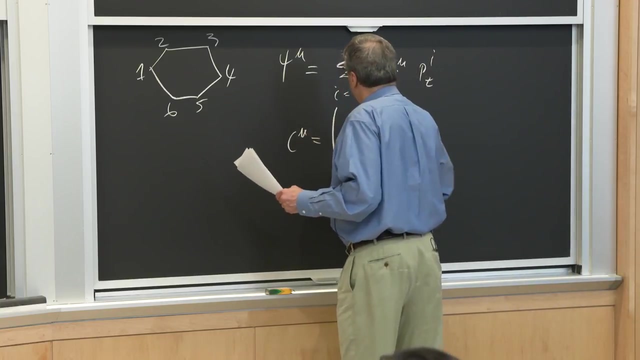 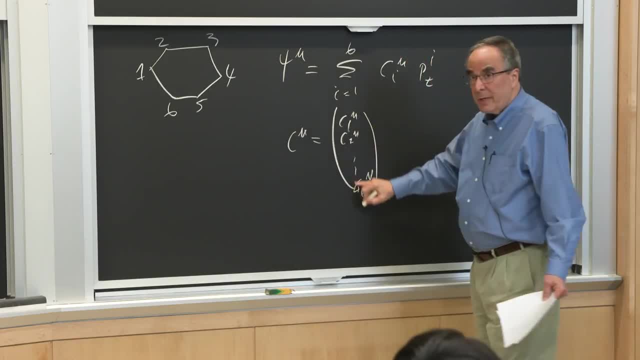 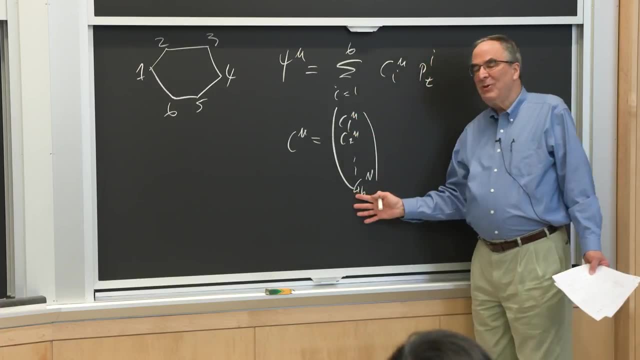 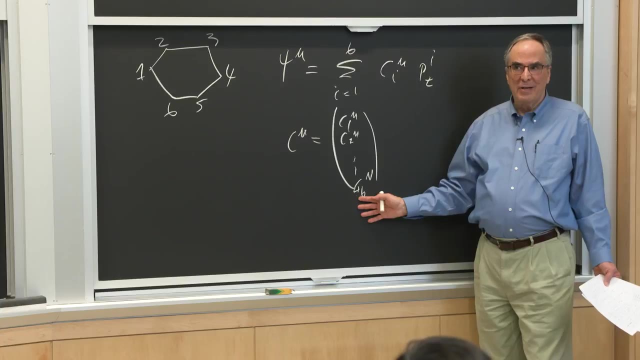 It's a c6 mu. These are the mixing coefficients. Well, for benzene it's pretty simple, because you know that if you have no nodes in symmetry, all of these are going to be the same, And so if you put 1s here, you put a 1 over square root of 6. 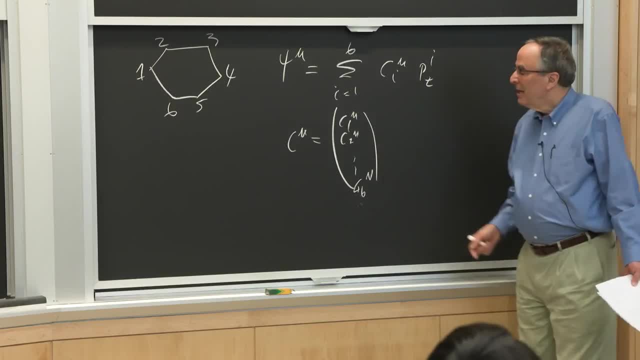 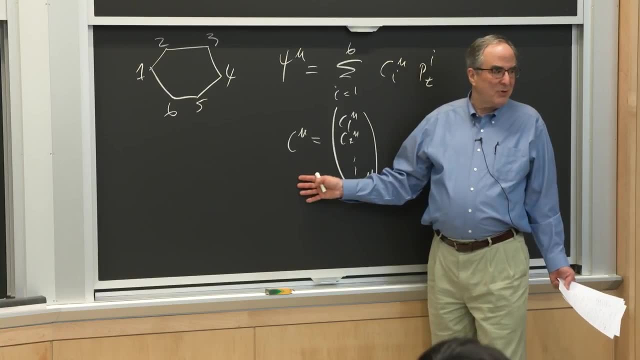 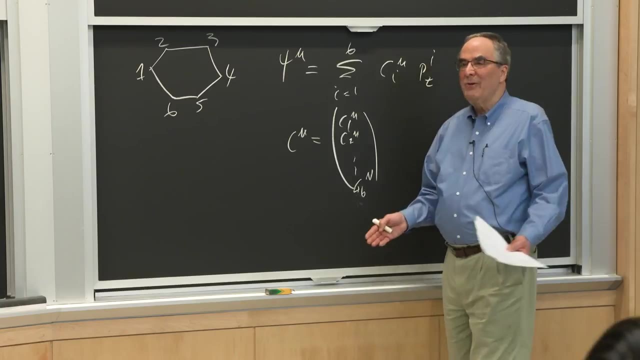 out in front for normalization, for normalization. And you can figure out the eigenvectors for benzene, all of them just by counting the number of nodes. And that's useful, because if you know the eigenvectors, then you can show what the eigenvalue is. 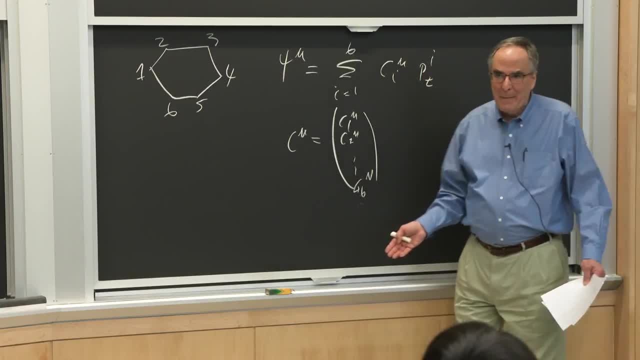 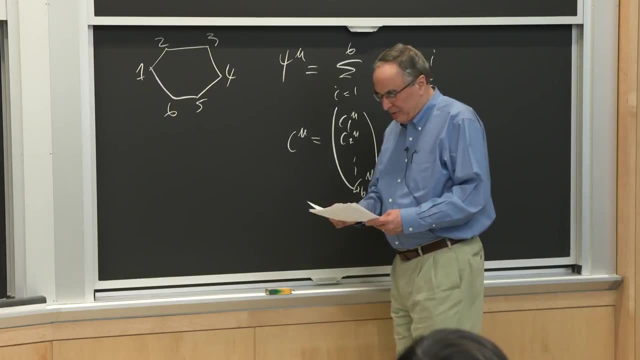 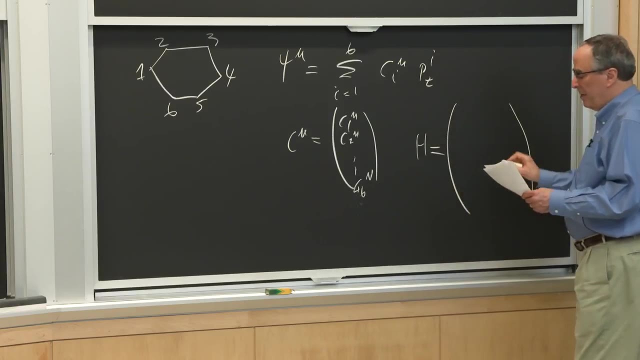 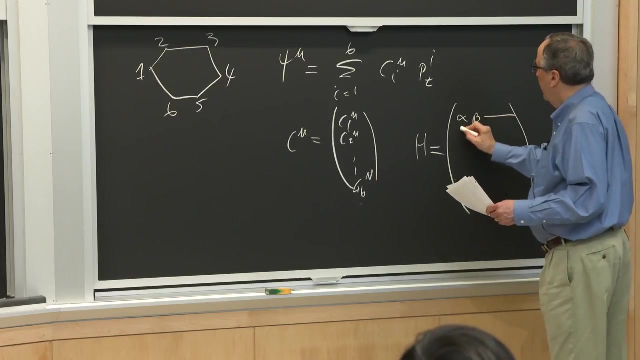 by multiplying the original Hamiltonian by an eigenvector, So you can. So anyway, we have this And then the Hamiltonian, we have alpha beta and then zeros and beta, alpha beta and then zeros, et cetera. 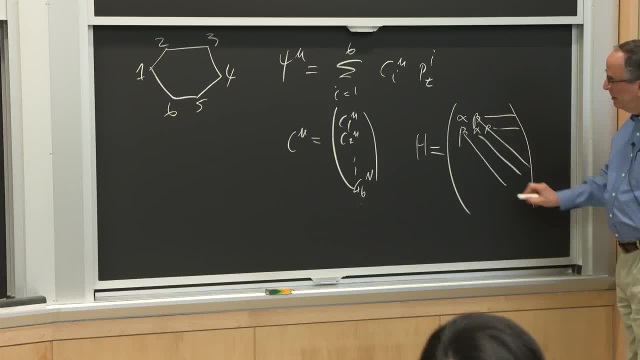 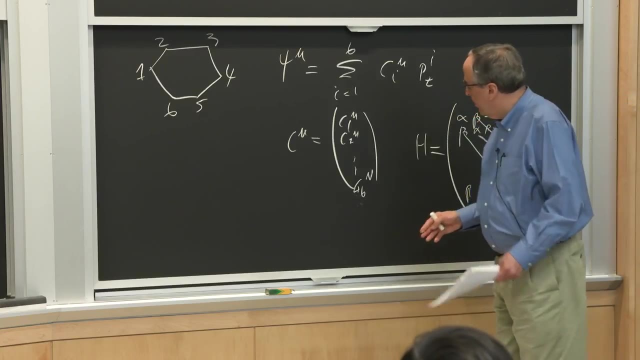 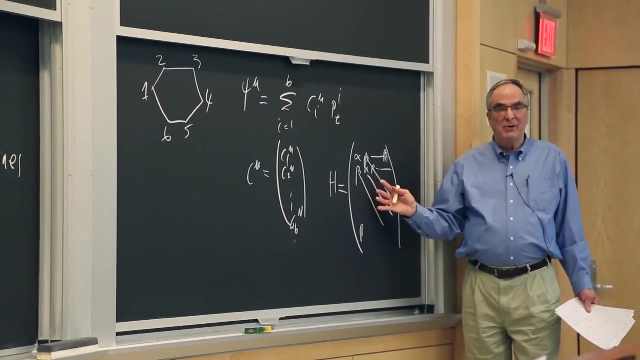 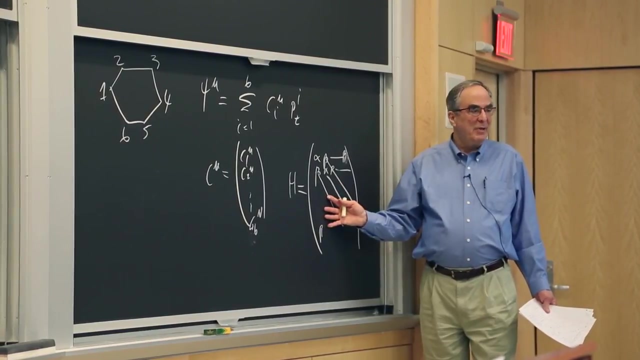 And so we have this tridiagonal structure, And because it's a ring, we have a beta here and here. So then we ask our computer to diagonalize this, Or you use clever tricks from algebra to find the eigenvalues. But I don't recommend it. 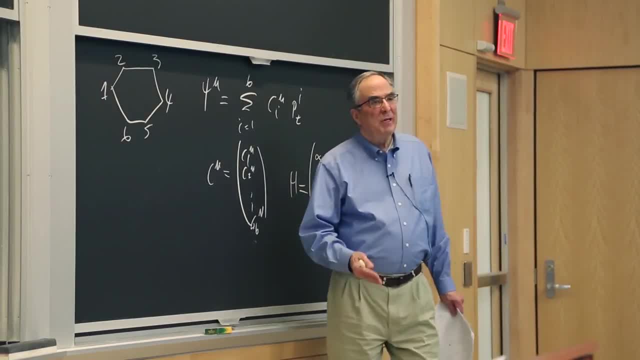 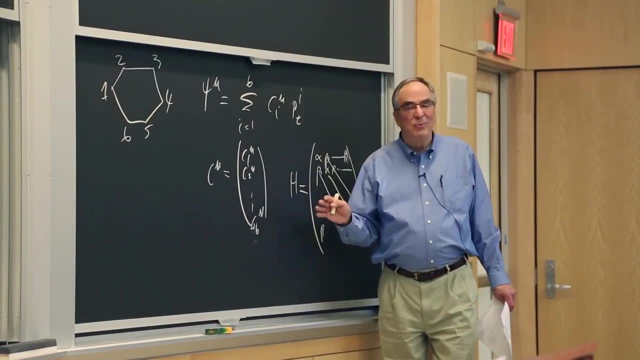 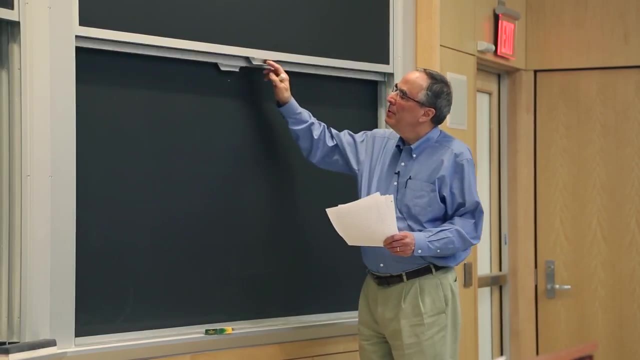 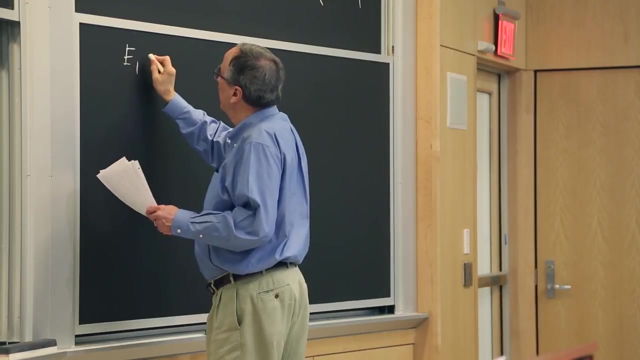 I mean, the general problem is going to be something where you have to use a computer. So don't develop tricks unless you want to check to see whether you programmed the computer correctly. And so when you do this, you get E1, the lowest energy. 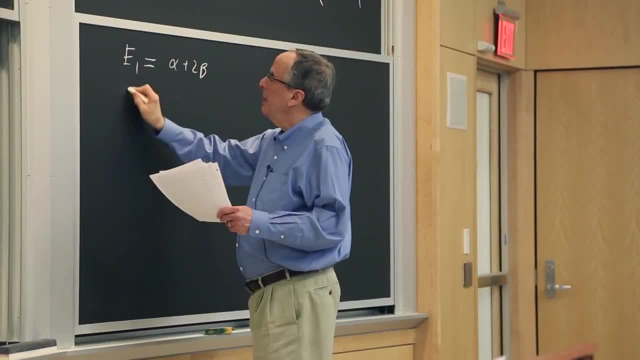 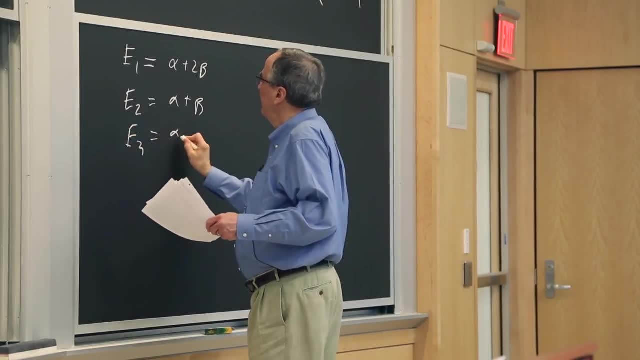 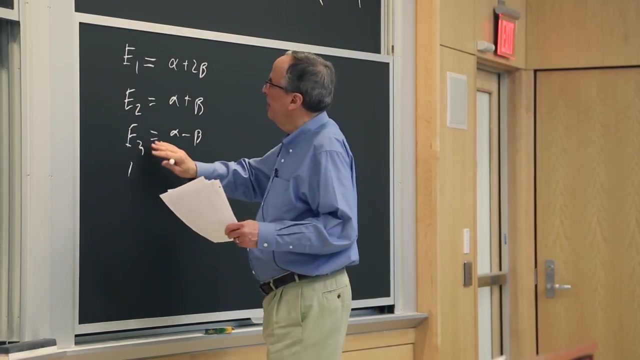 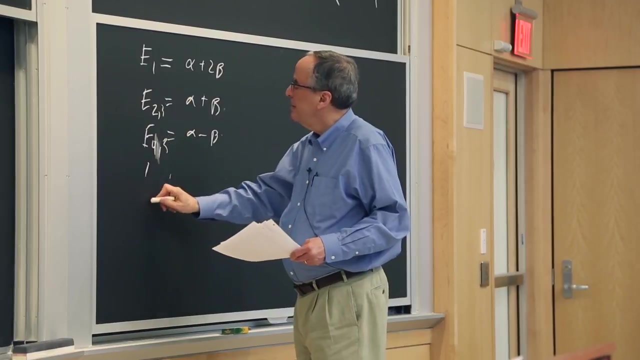 is alpha plus 2 beta And E2 is alpha plus beta And E3 is alpha. It's alpha minus beta And, I'm sorry, E2 and E3 are both this, And E4 and E5 are this And E6 is alpha minus 2 beta. 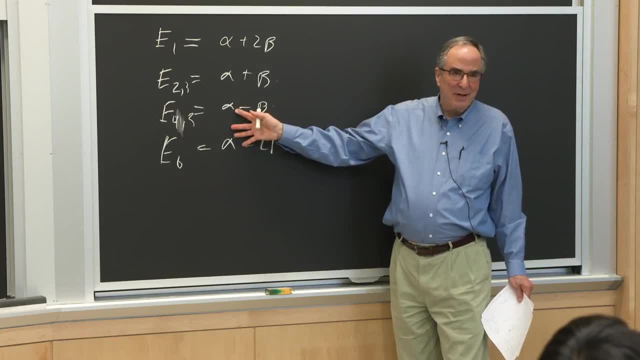 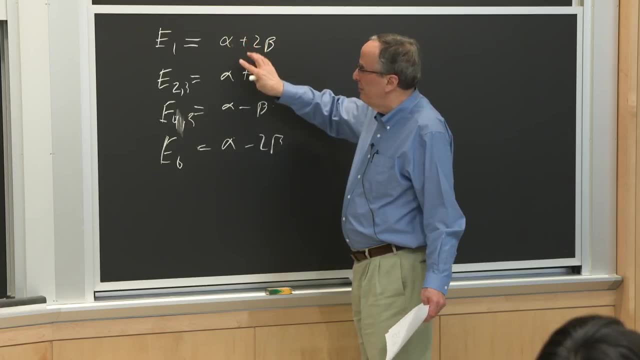 Now, we don't really care about these orbitals because they don't put electrons in them, And so when you put the electrons in the orbitals, you get two for this, two for this, two for that, And so we just calculate the sum of the energies. 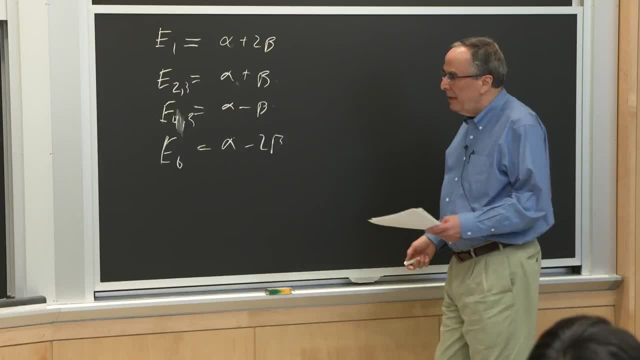 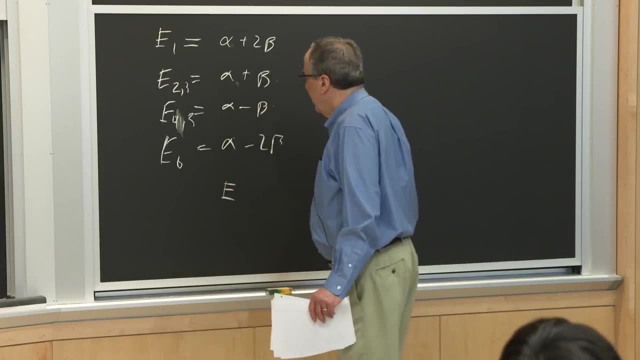 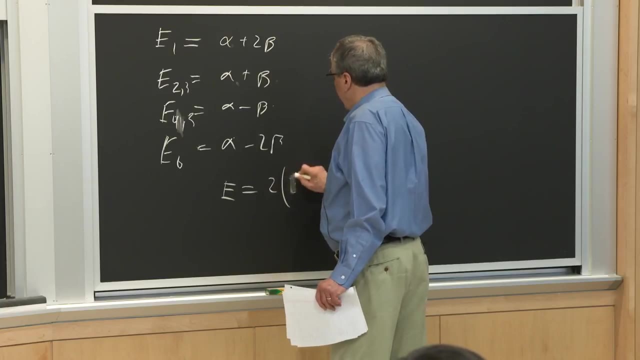 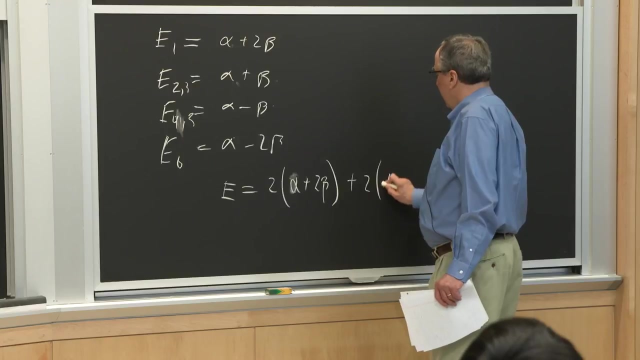 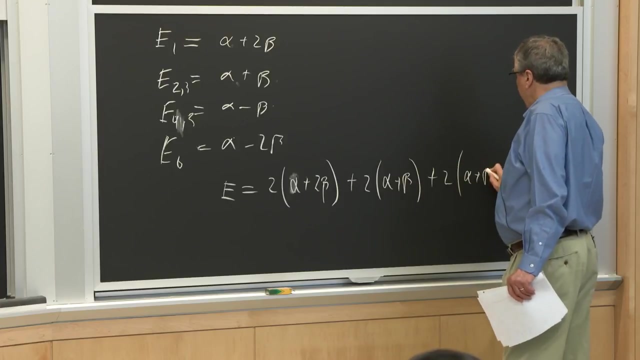 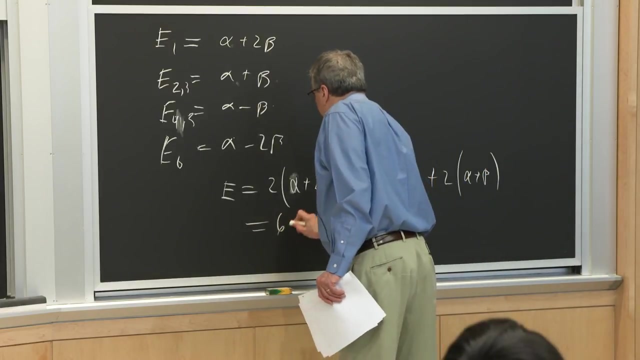 And we end up getting the energy levels for benzene. The ground state is going to be 2 alpha Alpha plus 2 beta plus 2 alpha plus beta plus 2 alpha plus beta, right, And so this gives you 6 alpha plus 8 beta. 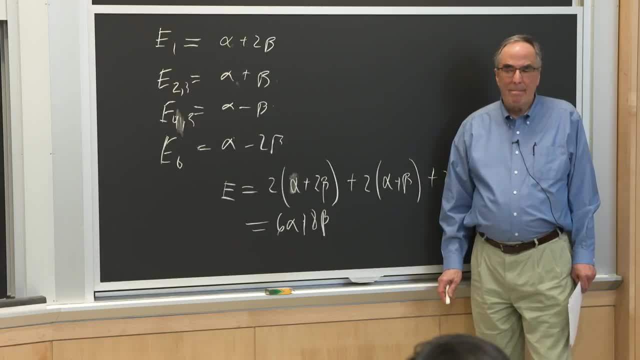 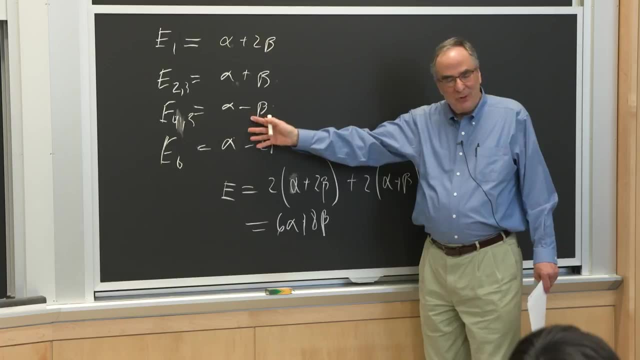 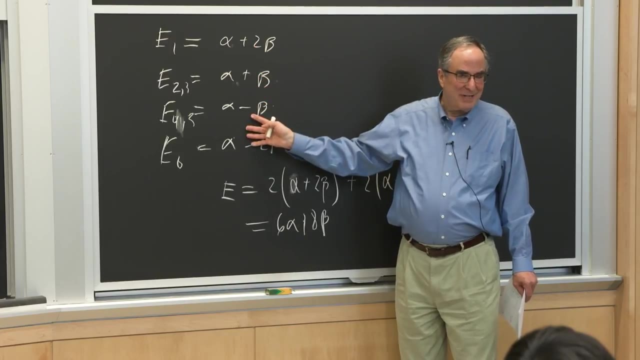 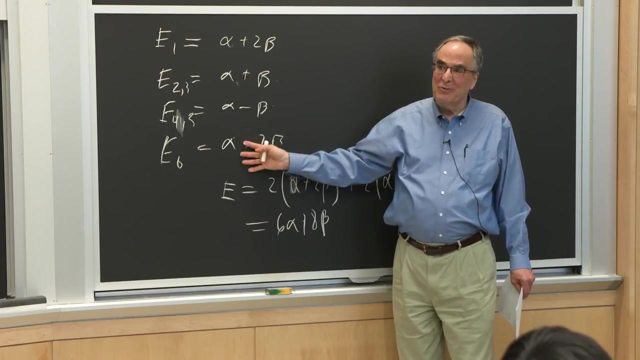 Now this: you might have guessed it, but you didn't guess it. Your computer told you that, And the computer actually likes numbers rather than symbols, And so to actually obtain this simple structure from the computer requires a little bit of manipulation. 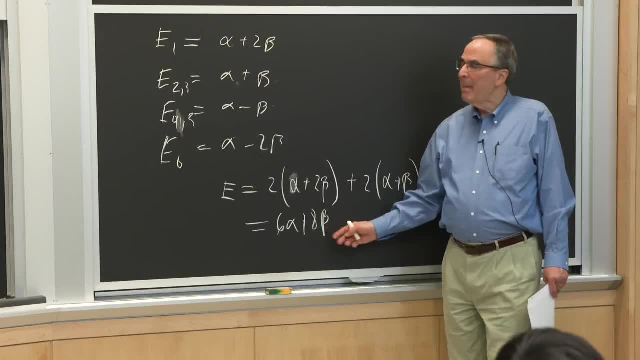 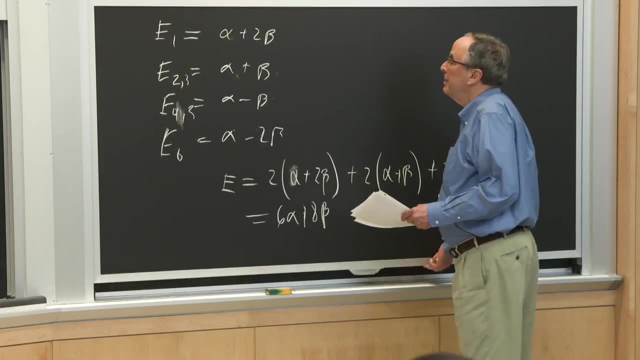 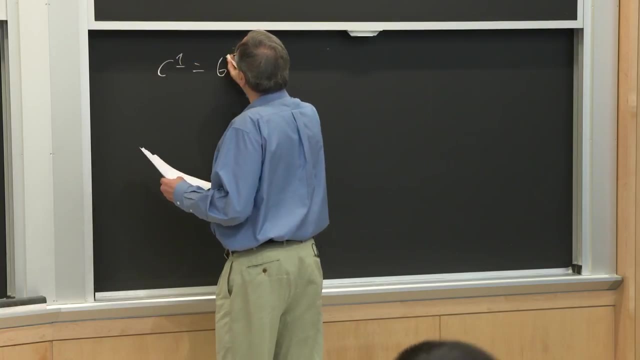 But you still get 6 alpha plus 8 beta, Alpha plus 8 beta, And you also get the eigenvectors And that's the stuff that you know. So C1 is 1 over square root of 6, 1, 1, all of those. 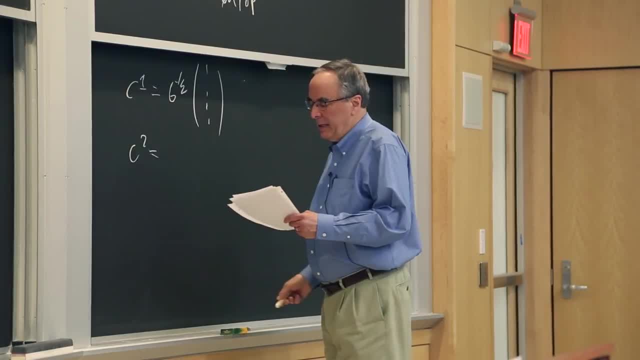 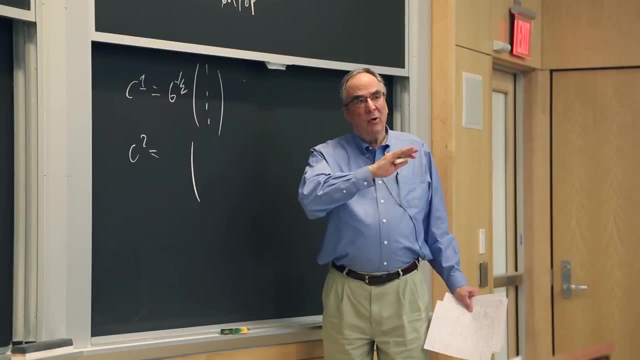 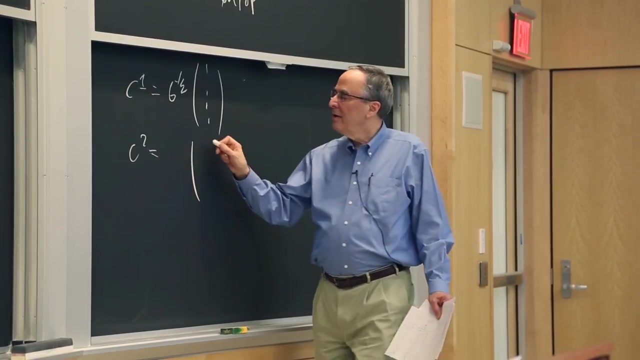 And C2 is going to be something a little bit more complicated. We can have, We can have the nodal plane going through atoms, And so if it goes through atom 1, it's also going to go through atom 4.. And so we have 0 and 0, 1, 1, 1, 1.. 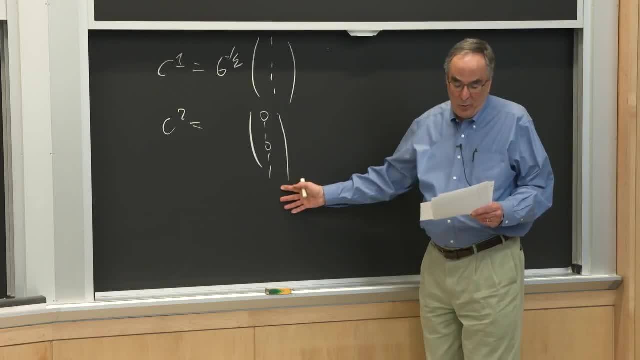 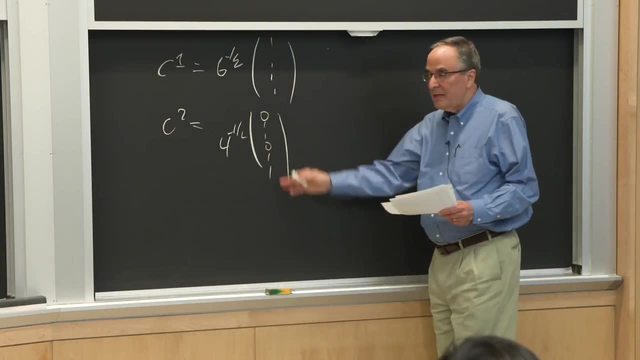 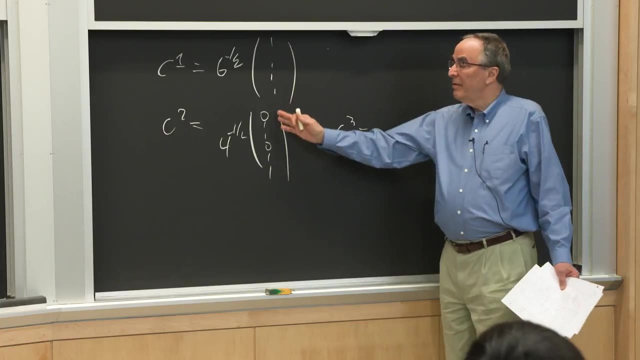 And now to figure out how to normalize that we just 1 over square root of 4, and so on. We can figure these things out. C3 is going to be an eigenvector Now, instead of having the nodal plane going through atoms. 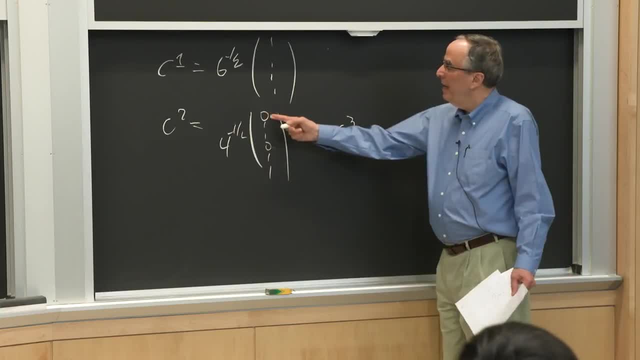 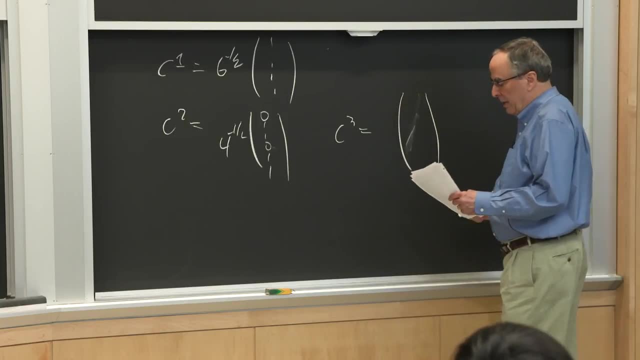 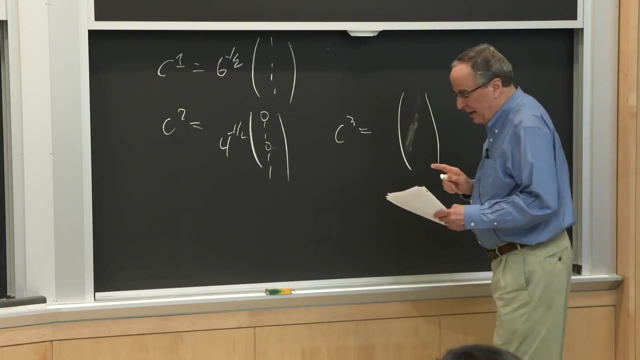 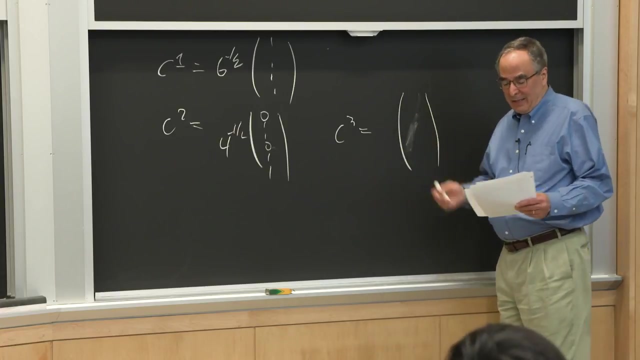 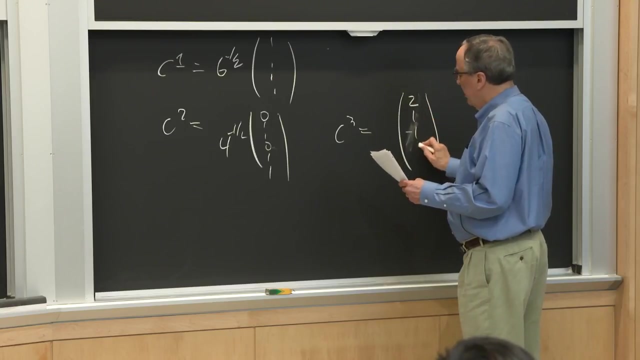 it's going between atoms, And so instead of having any 0's, you're going to have something more complicated. And now I can see that there's something in my notes which is subject to how you You actually impose the symmetry, But suppose you have something like this: 2, 1, minus 1,. 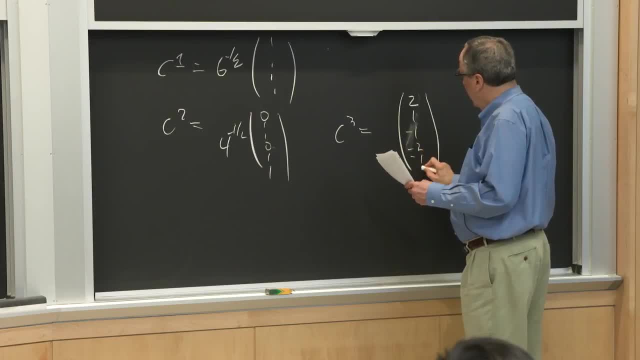 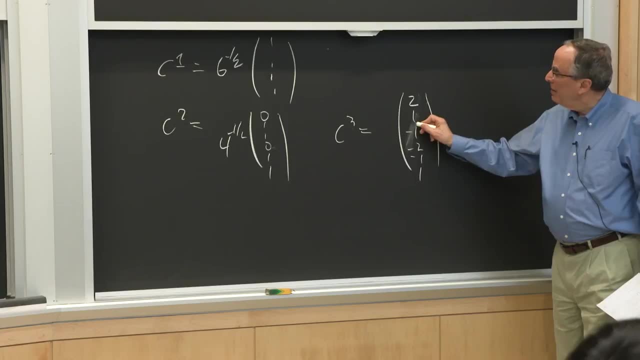 minus 2, minus 1, 1.. So why did I use these numbers? Well, I had to have a nodal plane here between atoms 2 and 3.. And the corresponding guy will be: Well, that should have been a 2 at the bottom. 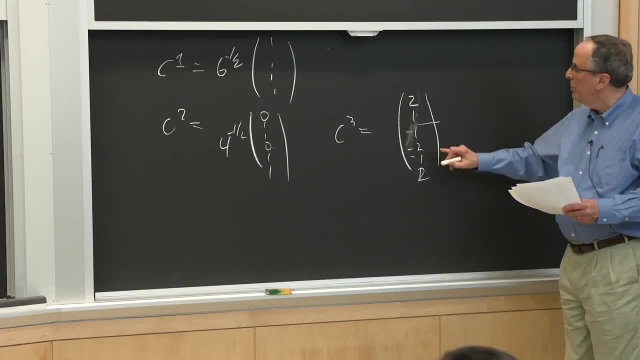 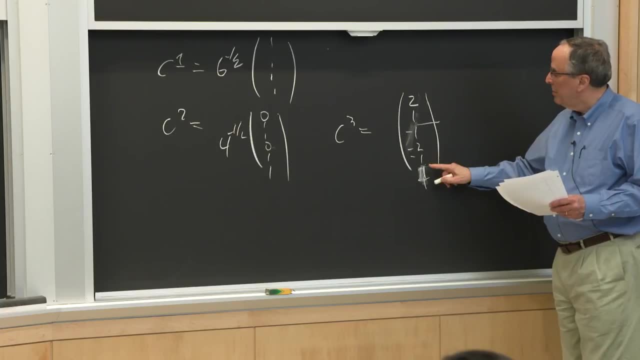 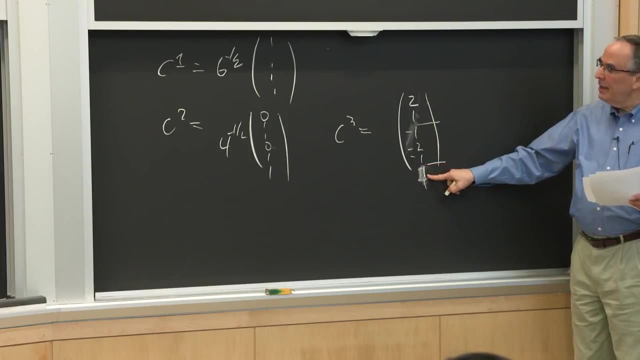 Let me just make sure I'm doing this right. No, I had a 2. OK, it's a 1. OK, and so the last one is here. So the sign change occurs twice and those correspond to opposite bonds. 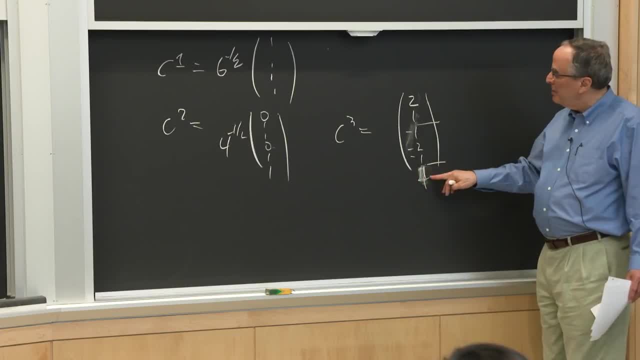 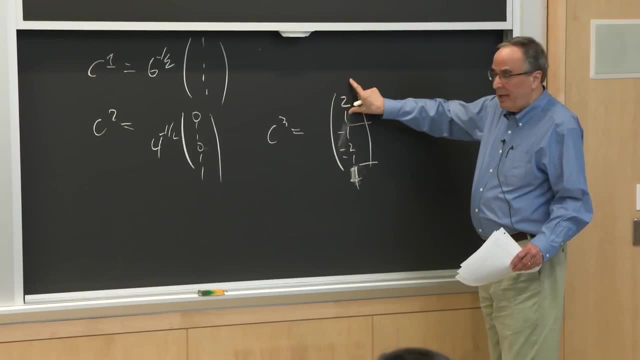 And anyway, if this is, Why were there 2's? Well, the 2's are between two atoms that have 1's, And so it's going to have a larger eigenvector, And you can figure it out lots of ways. 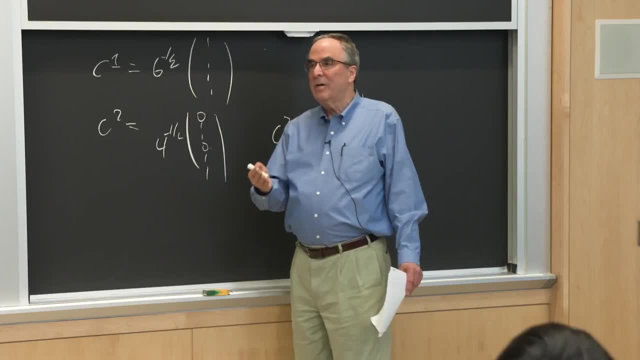 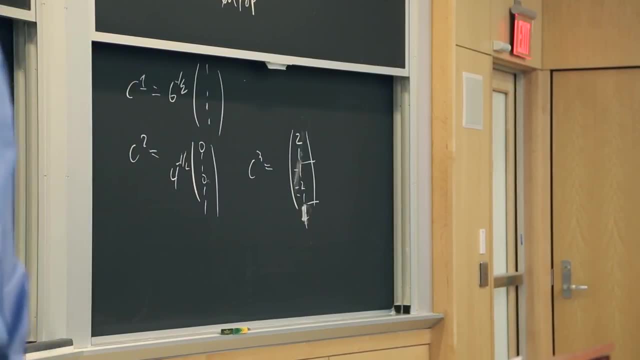 You can also say: well, every atom has to be used up. Yes, So should there also be a sign change in C2?? Could there also be a sign change in C2?? C, b and c, Yeah, Yeah. 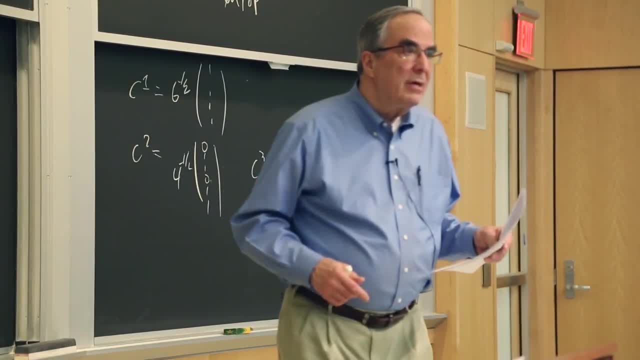 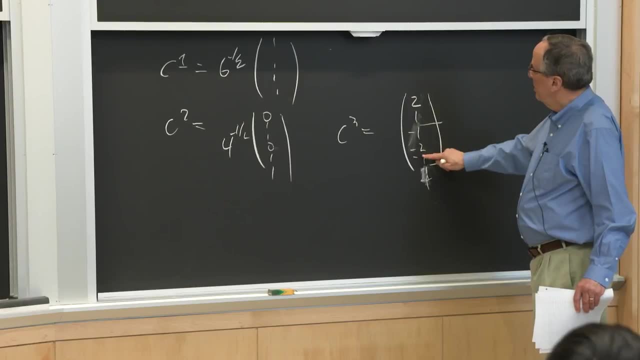 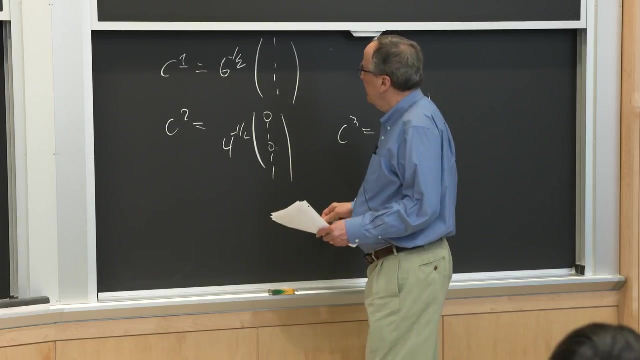 C2, 6 should be bigger. Did I screw up? Yeah, No, no, it's C2, not C3.. I'm sorry, The previous one. Oh yeah, yeah these. So opposite sides, OK. 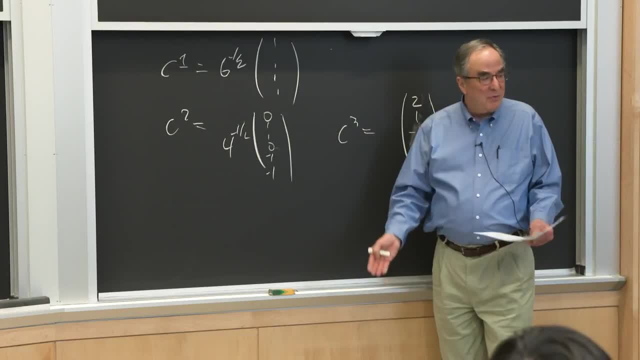 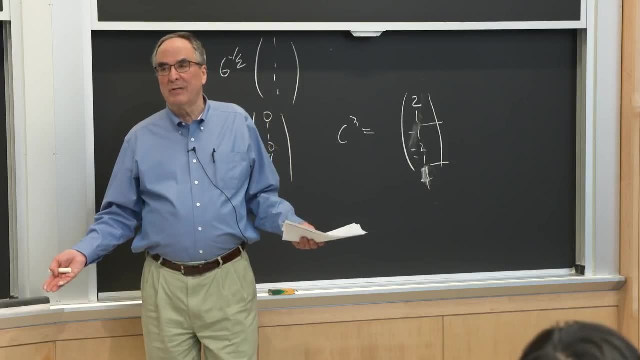 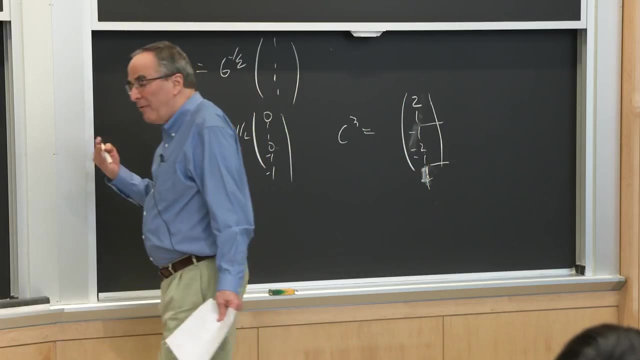 All right, it doesn't matter, The computer tells you, It tells you. But sometimes you can approach the problem very quickly and just say: I know what the eigenvectors are going to be and I have to normalize them. And so, but one of the things that you often 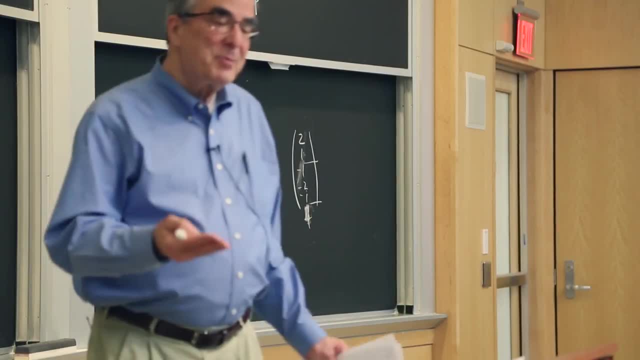 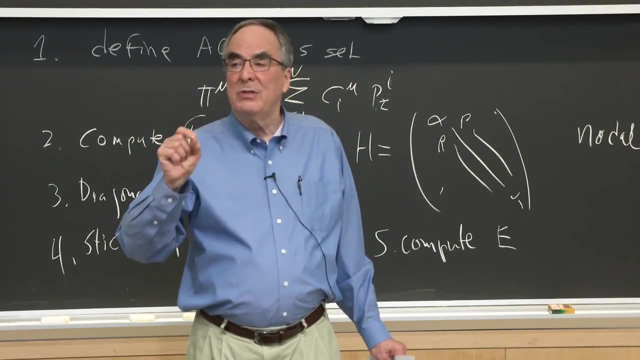 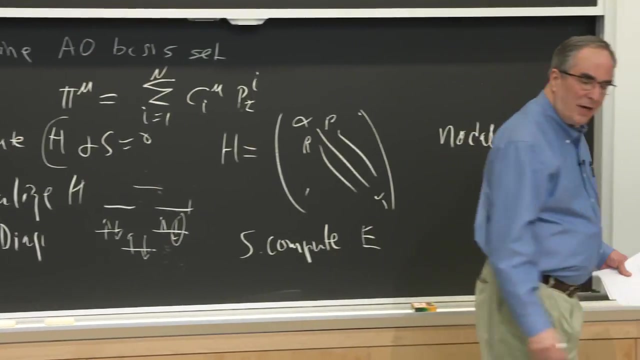 do if you're trying to be smart and skip steps is to say: OK, we have six eigenvectors And each of the atomic orbitals gets used up completely among the six eigenvectors. And I do that all the time because it's. 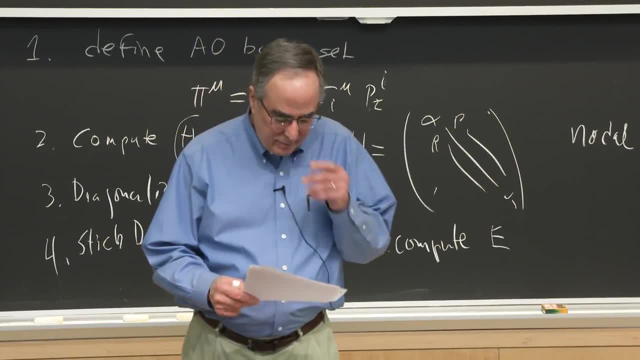 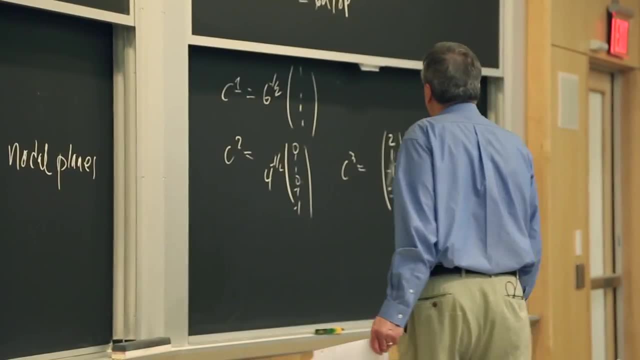 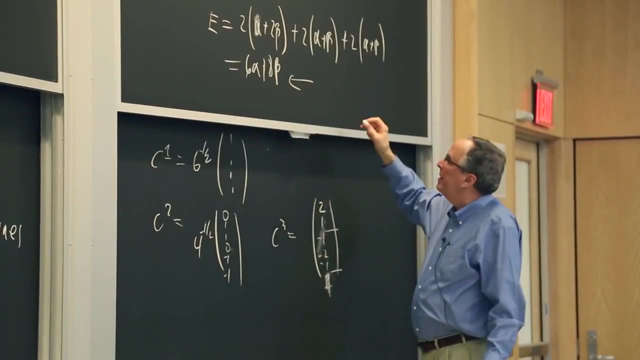 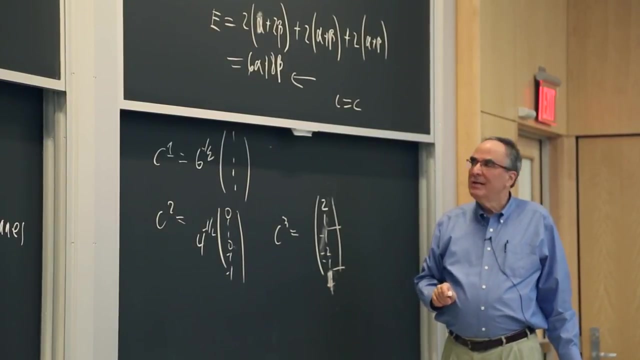 a very useful way of making sure I haven't screwed up. OK, so we get this And that's perfectly OK. We don't know how significant it is, But if we say we had three of these three ethylenes, 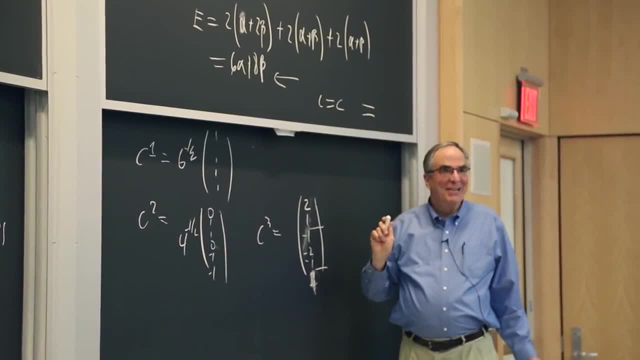 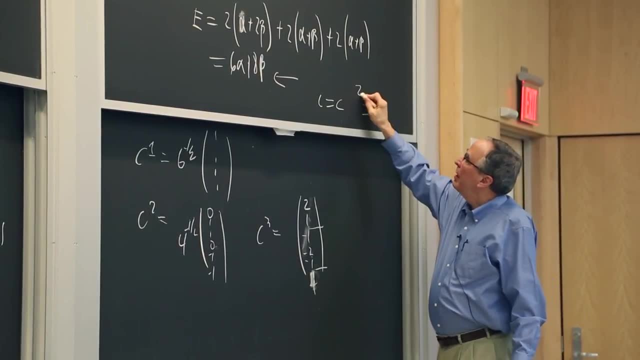 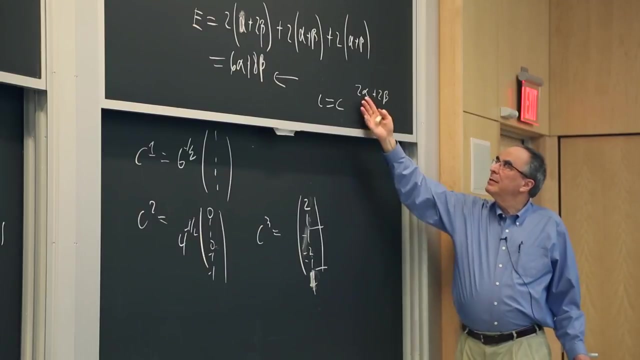 I guess if an organic chemist would just do that, right. But anyway, if we had three of these, when you do this you get 2 alpha plus 2 beta, So we get 6 alpha plus 6 beta, And alpha and beta are both negative. 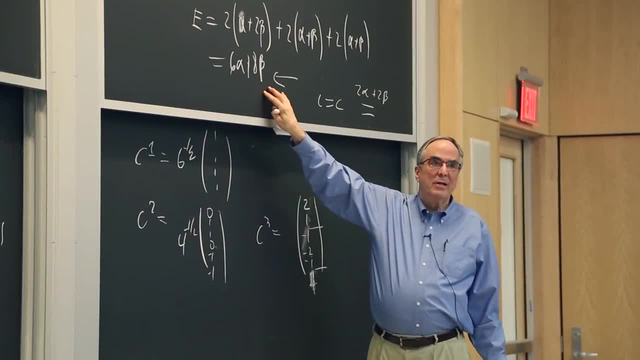 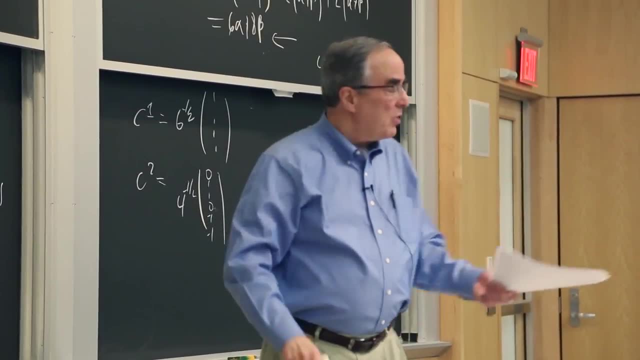 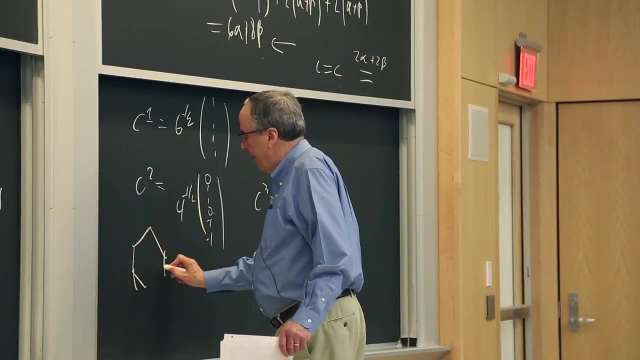 And so the energy for three ethylenes did I screw up again? But how would those ethylenes be developed into one another? They're separate. So we're just saying: is benzene, we could draw benzene. 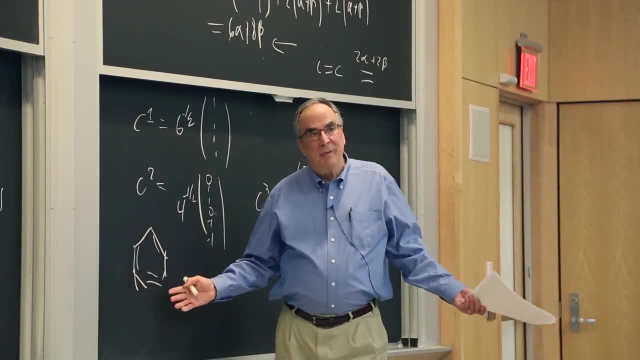 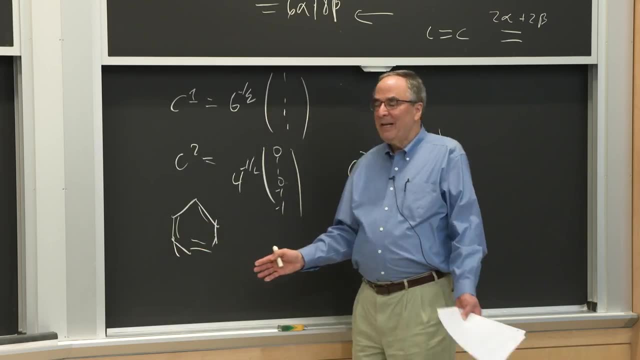 And so we could say we have three isolated bonds, And since we don't care about the sigma structure and no bonds are adjacent, they're additive, And so we represent benzene. The primitive structure for benzene is three ethylenes. 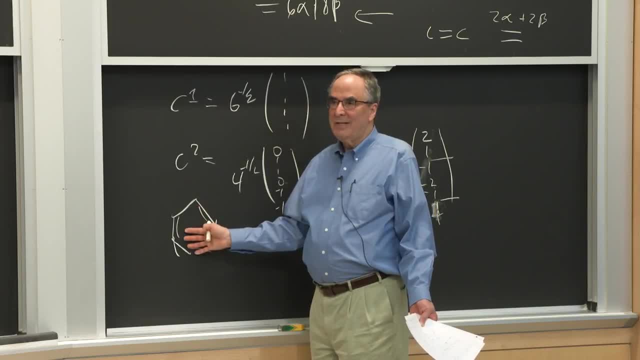 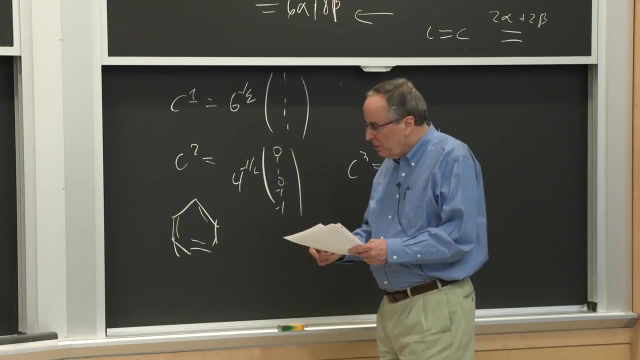 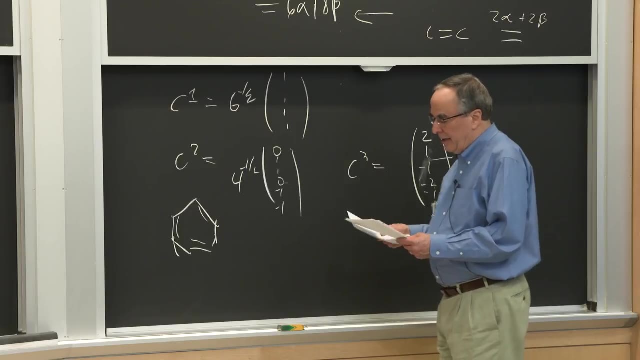 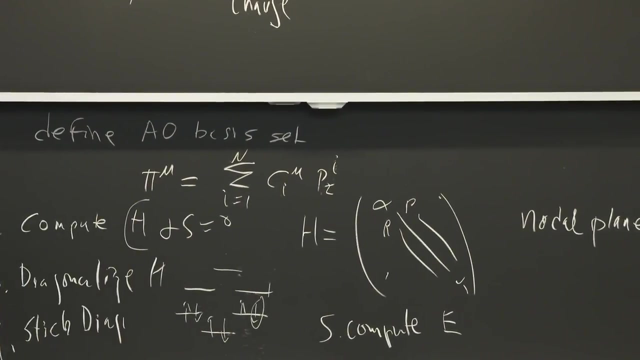 And benzene is two beta better. That's the resonance stabilization. That's a great thing, OK, So we get a resonance stabilization, And now the more subtle and wonderful stuff is: we have these eigenvectors. We have these eigenvectors. 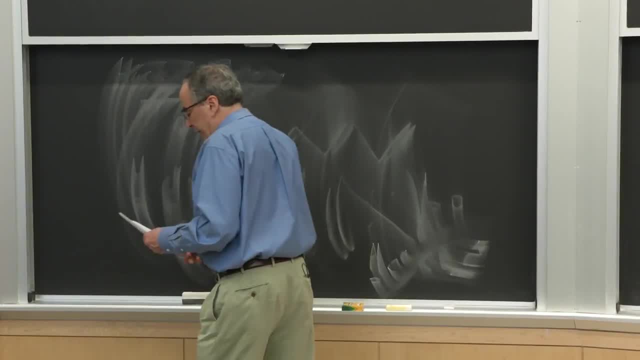 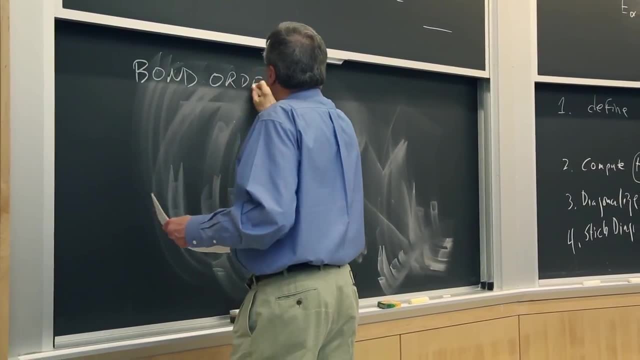 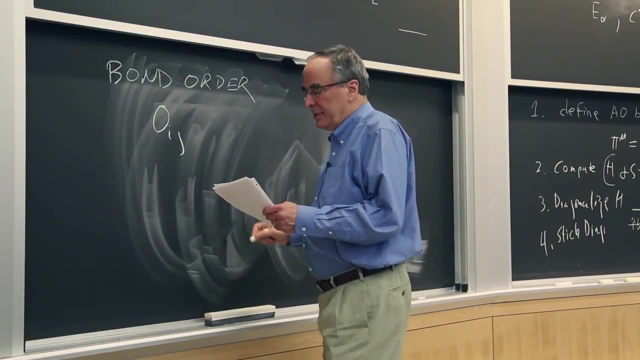 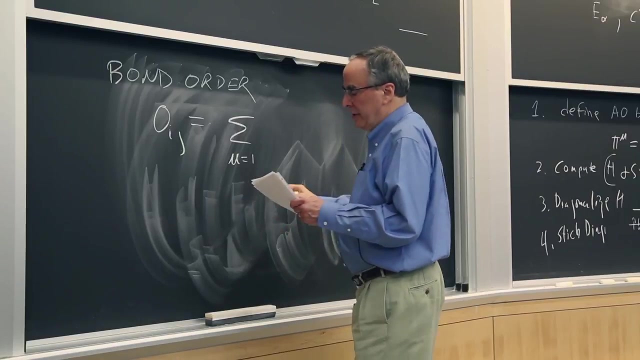 And we have the energies And we can do stuff with them. And one thing is bond order, And so we have a formula: The bond order between atoms i and j is equal to the sum for mu equals 1 to the including only. 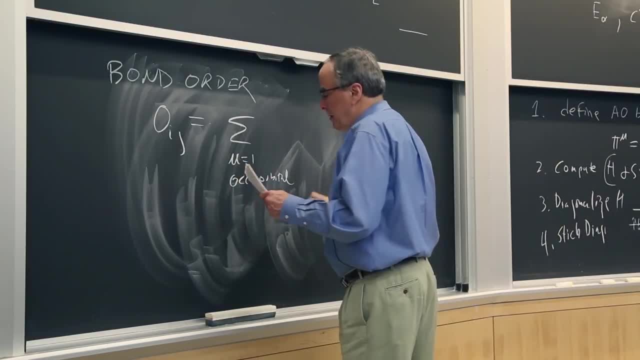 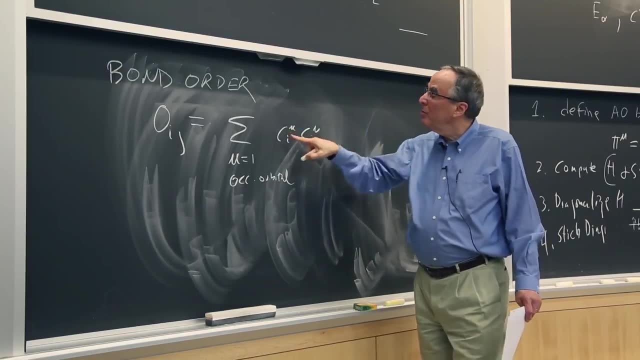 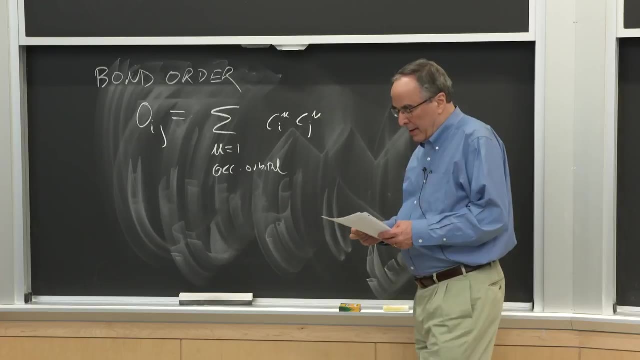 the occupied orbitals, And we can do that by taking the bond order of C, i, mu, C, j, mu. So we have the mu orbitals, the mu molecular orbitals, and we have the adjacent atoms, And this gives you the bond order. 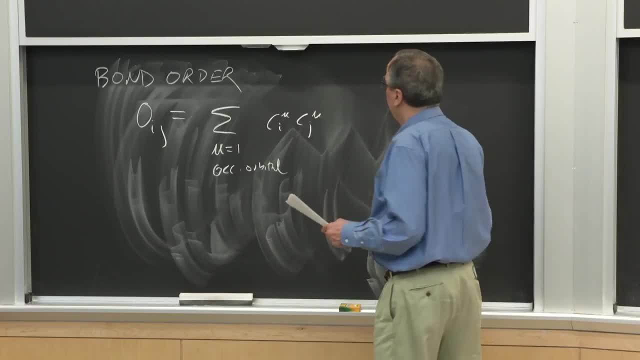 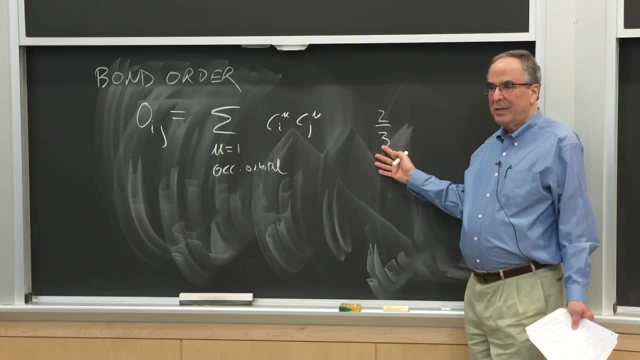 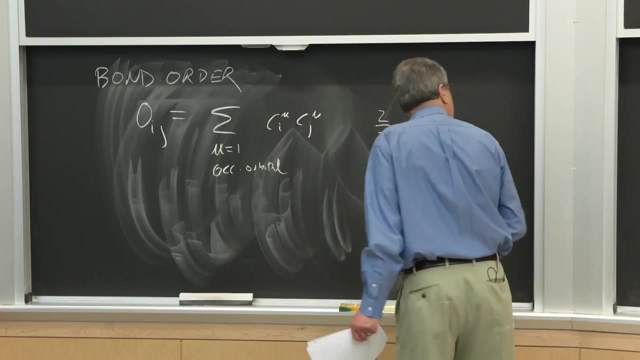 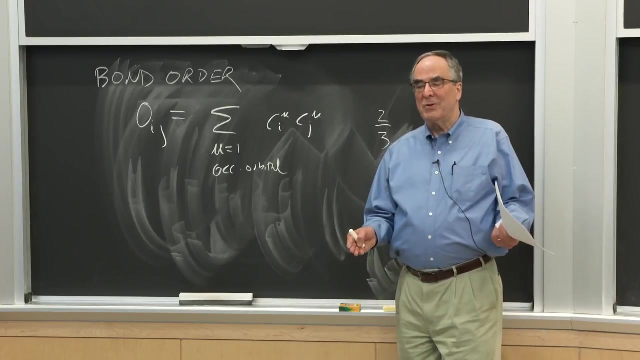 And so we can calculate the bond order And we find that every bond has a bond order, a pi bond order of 2 thirds, which is neat Because The non-resonant structure says three of the bonds have a bond order of 0, a pi bond order of 0,. 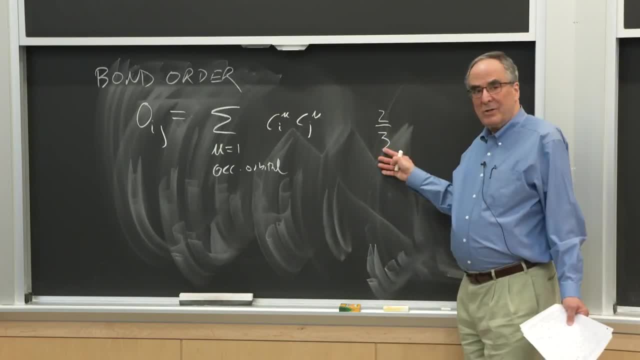 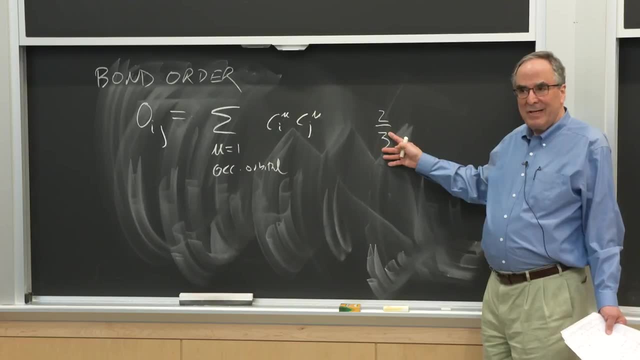 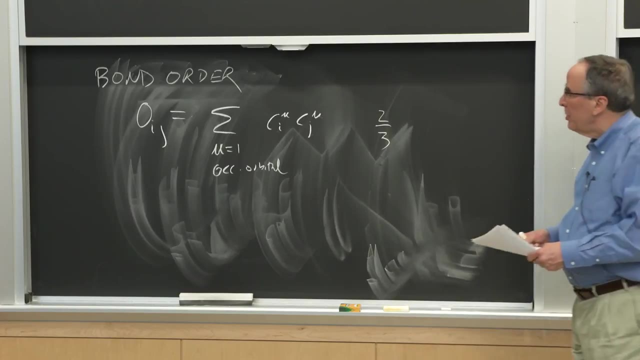 and three have a bond order of 1. And so the average is 1 half And this is bigger than 1 half And it's uniform. So you can do this And you can say: OK, the 1, 2 bond order, the 2, 3 bond order. 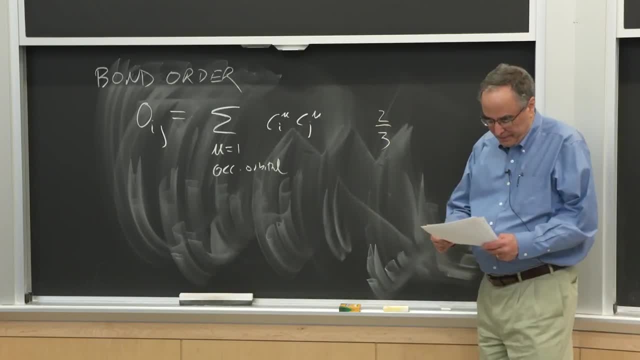 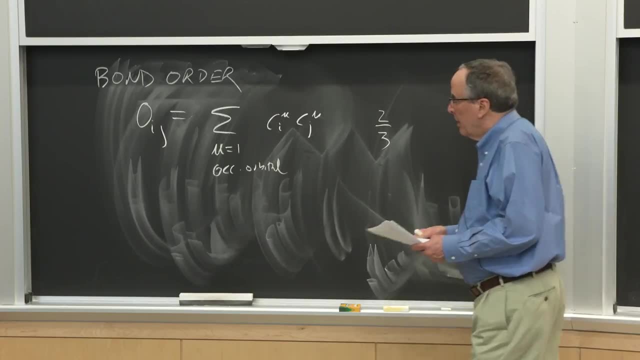 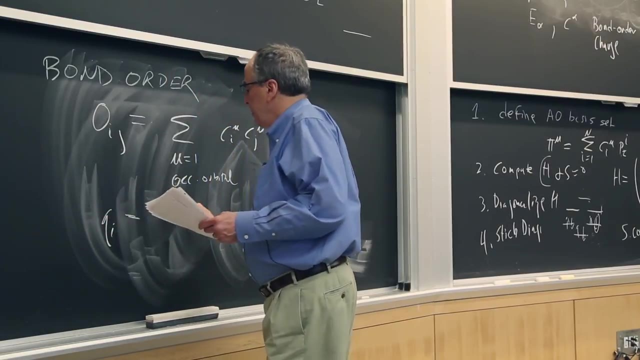 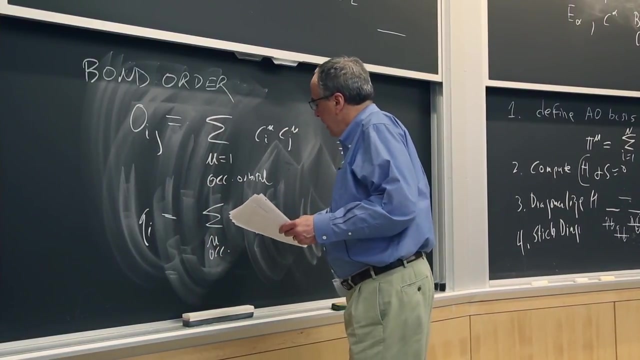 You do the laborious calculation, you always get 2 thirds. Now you could also calculate the charge on atom i, And that is again mu for the occupied orbitals, And that would be C, i, C, i, mu, C, i, mu. 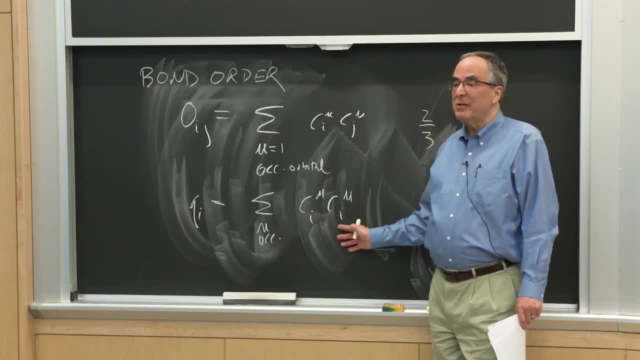 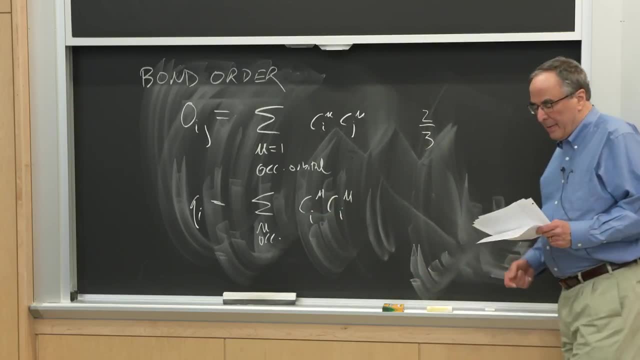 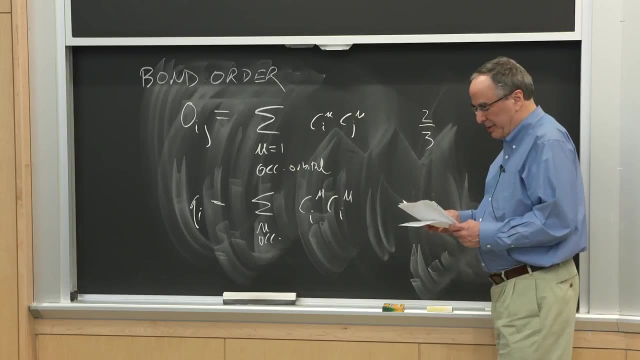 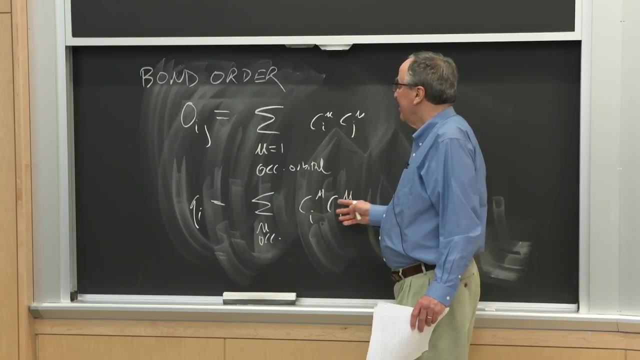 And so for benzene, you would expect this to come out to be 0. And it does, So there is no charge. Let me just make sure that that, Well, there's a, There's an equal charge on each atom, whether it's 0 or 1. sixth,